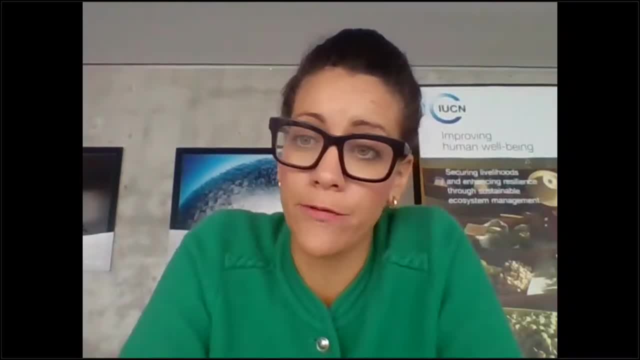 UN BB&J intersessional work. So it's an online forum And, for those of you who have followed it, it was actually on environmental impact assessments, which is very timely, because that is actually a very timely webinar. So thank you so much for joining us today And 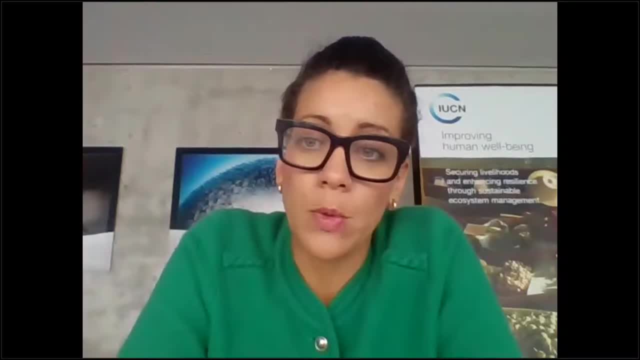 this is actually the topic of today's webinar. We're looking into integrating climate change into environmental impact assessments. So my name is Mina Ebbs and I work for IUCN's Global Marine and Polar Program, So this is a webinar that we put together jointly together. 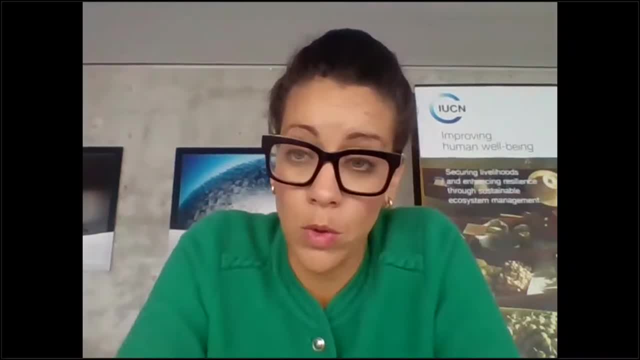 with IUCN's World Commission on International Environmental Law, And so today, this today's meeting, will actually be recorded, And we will have a moderator, Simi Payne, who is the chair for IUCN's Commission on World International Environmental Law, And we will also be joined by three distinguished speakers that will share their experience. 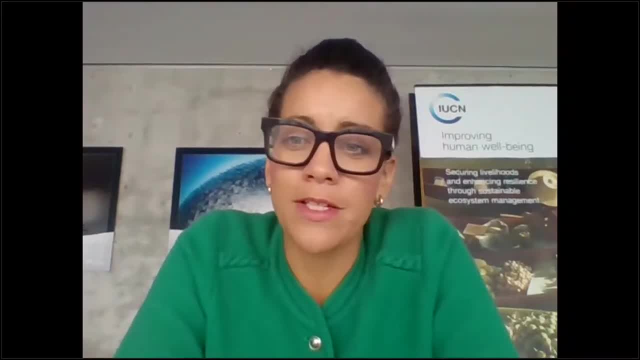 as well and give a short presentation. We will also invite our high seas advisor, Kristina Järda, to give some remark. you will be able to ask questions. you can drop them in the question panel. Kristina Järda in chat. 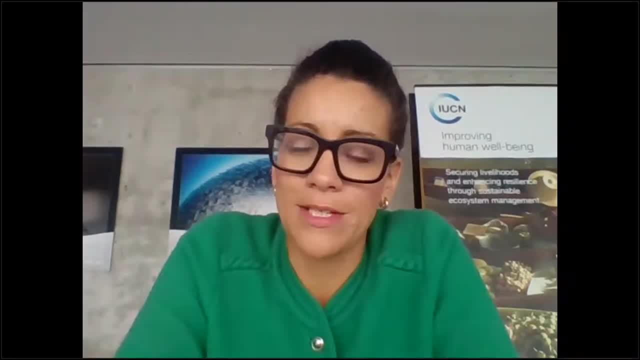 And then we will be able to address them after the presentation when we open up for questions. So we look forward to your active participation And also like to thank everyone once again who is joining us today, And also for two DOSI, which is the deep ocean stewardship. 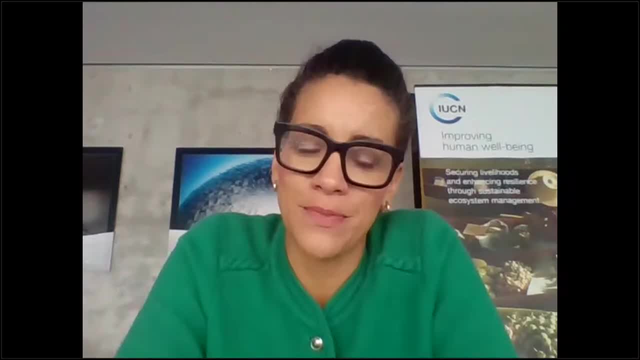 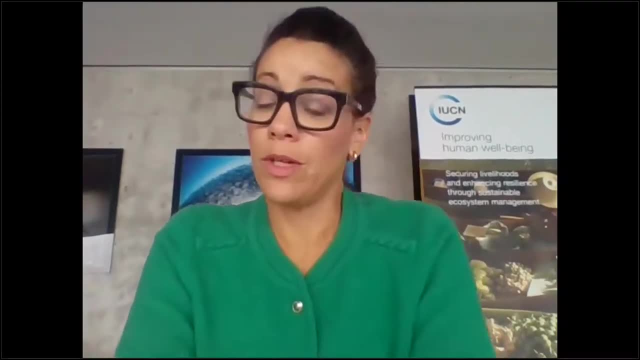 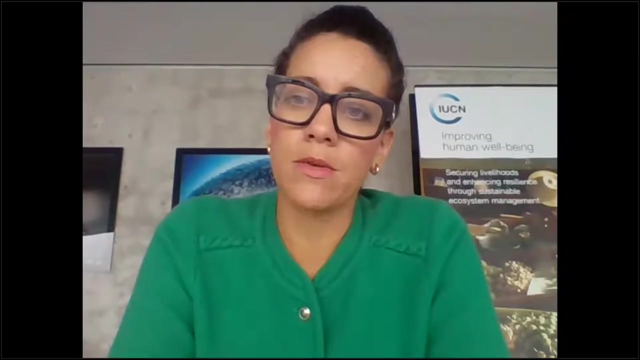 initiative, So also part of organizing this, together with irritation in its Commission. so, Without further delay, I'd like to hand over and, before doing so, also like to extend our gratitude towards the government of Sweden, which are sponsoring this series of webinar. 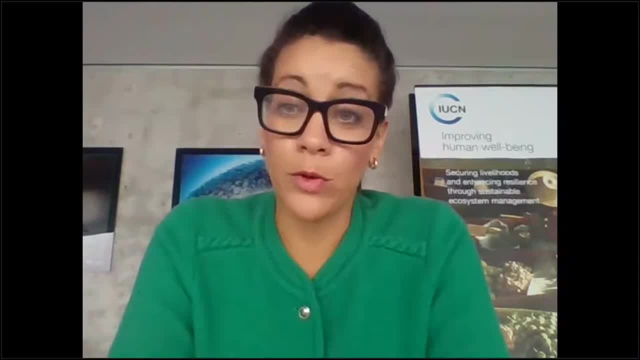 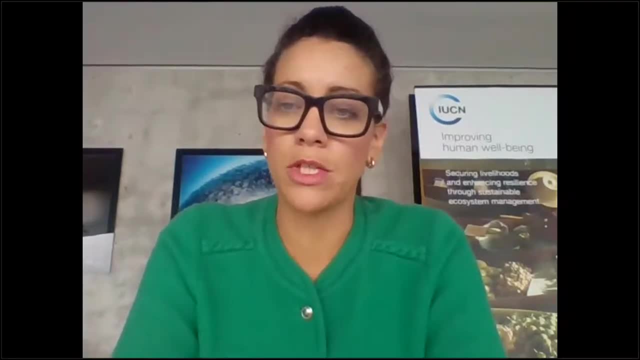 We will come back in the end and conclude and give you a schedule for the next webinar. We are also intending to build a knowledge series on biodiversity beyond national jurisdiction, in conjunction or in parallel to, as the informal discussions are going on and leading up to the 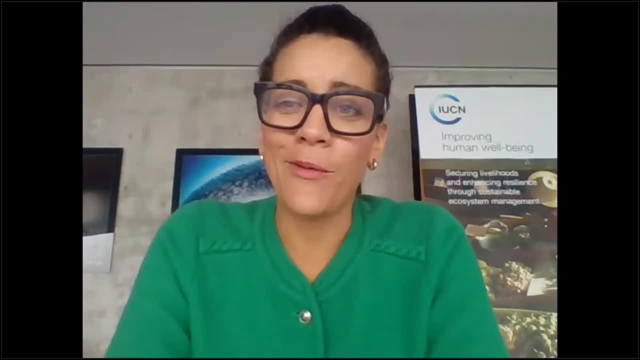 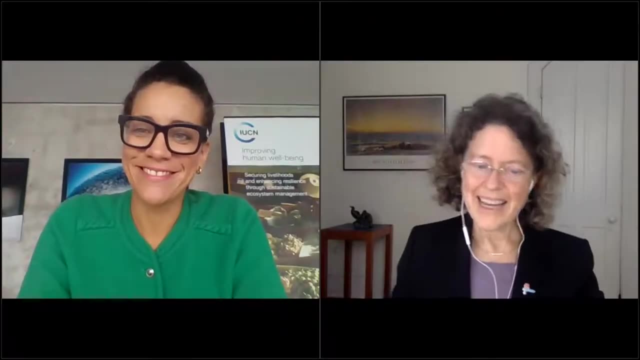 IGC4.. So, once again, thank you very much and I will hand over to Simi Paine, Over to you. Thank you very much. Thank you, Mina. It's a pleasure to be here with you all this morning. Good morning, good evening. 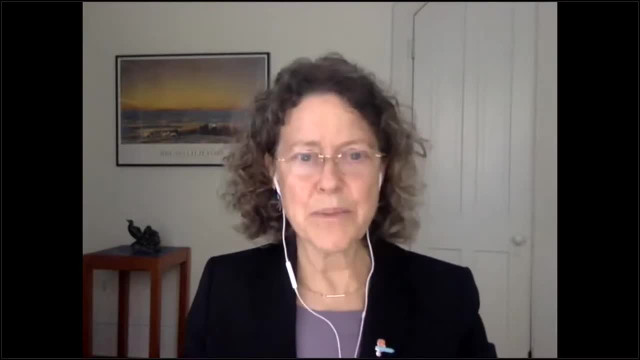 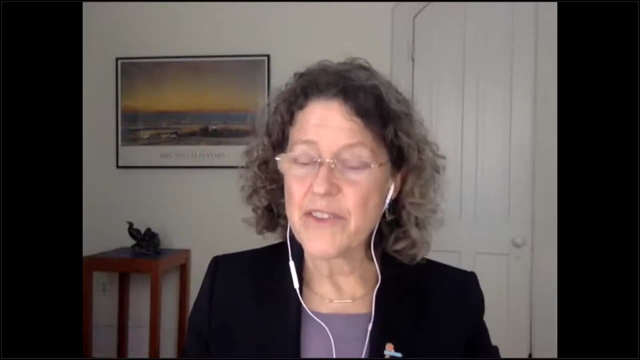 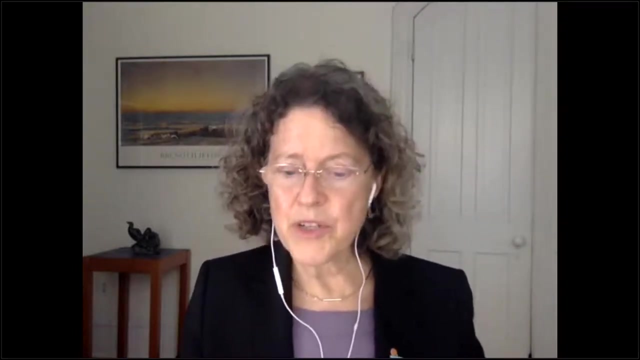 Good morning, good afternoon and good evening. It's a pleasure to be with you. to hear today We have seen that increasing scientific understanding of the physical and biological ocean tells us that ocean health is essential to human health and survival And that it is beautiful, dynamic and connected. After many years of work leading up to the 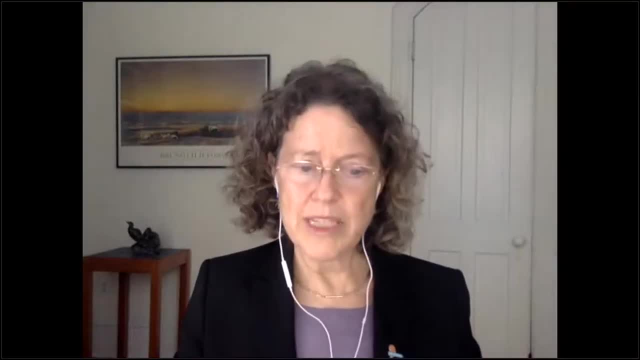 negotiation. in 2017, the UN General Assembly authorized four meetings to negotiate a new legally binding agreement for the conservation and sustainable use of marine biological diversity in areas beyond national jurisdiction- the BB&J agreement. I know many of you are deeply familiar with this, and even 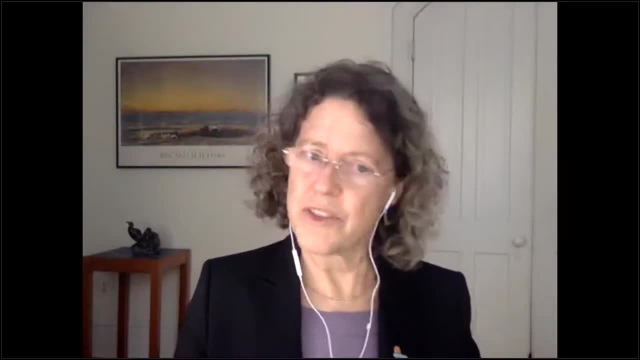 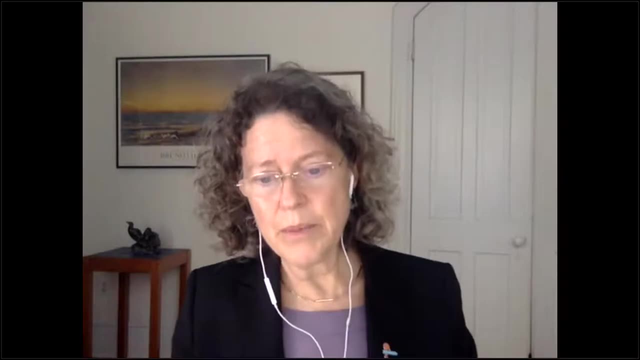 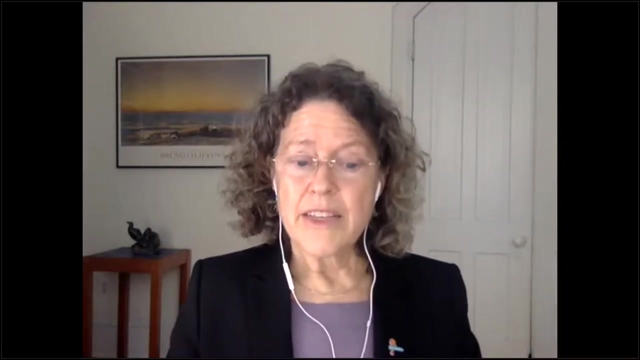 may have negotiated this already, but for those who are just joining, a little background. After three meetings of the negotiators, a text had been developed, but many questions remained unresolved and still remain unresolved. The fourth meeting, scheduled for this past March. 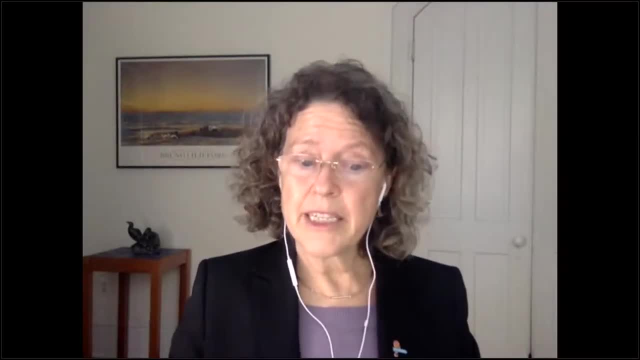 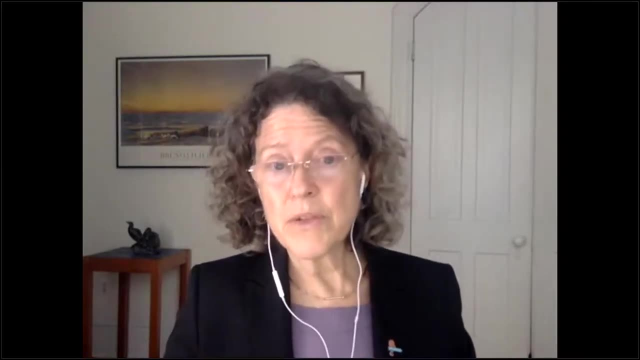 having been postponed. Ambassador Rina Lee initiated the novel intersessional process that Mina referred to, and the first round of these online chat-style exchanges has just finished, having engaged with four environmental impact assessment issues. Today, our panel is joined by Ambassador Rina Lee and Ambassador Rina Lee. 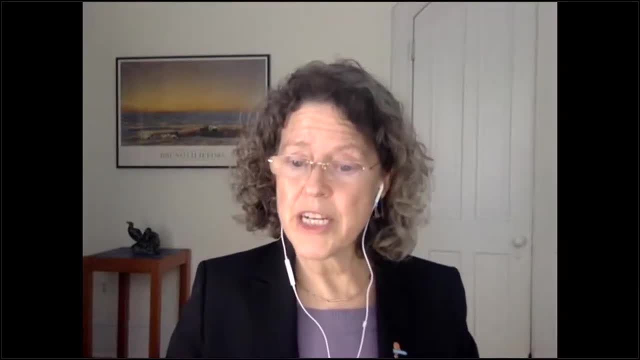 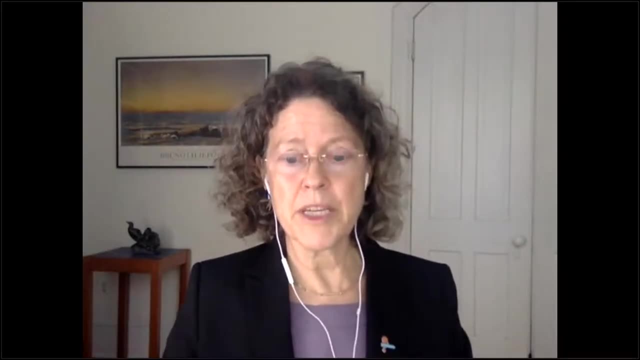 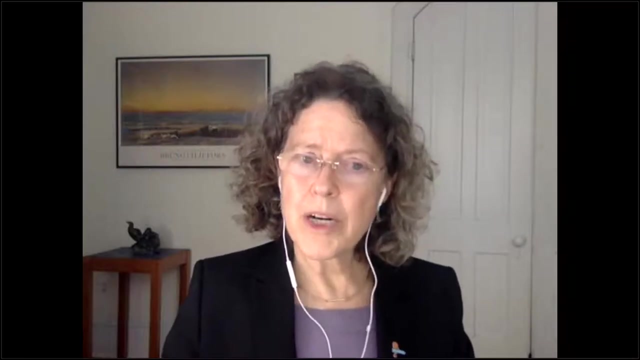 Our experts offer you their knowledge of how climate change affects the ocean, why it is critical that climate change be considered in all aspects of the BB&J Treaty, and how that can be done within the EIA process. A hallmark of climate change is uncertainty. The effects of climate change on Earth's physical 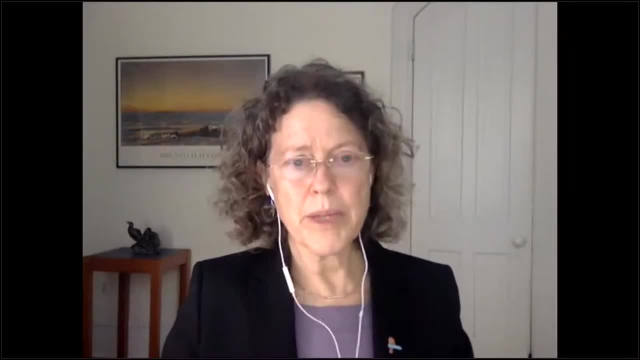 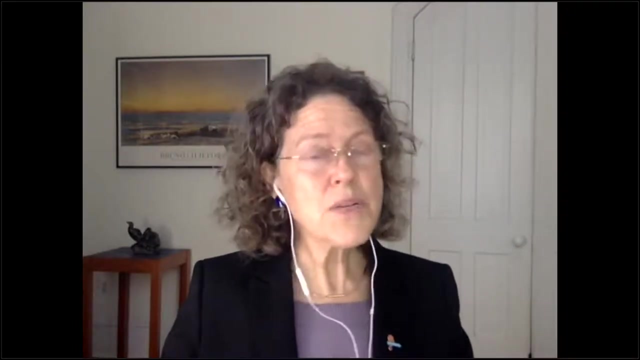 and biological systems are occurring with greater rapidity than anticipated. The BB&J agreement that we put in place now will govern rights, duties and cooperation between states in the ocean long into the future. That's why we want to Futur-Proof it to ensure that the 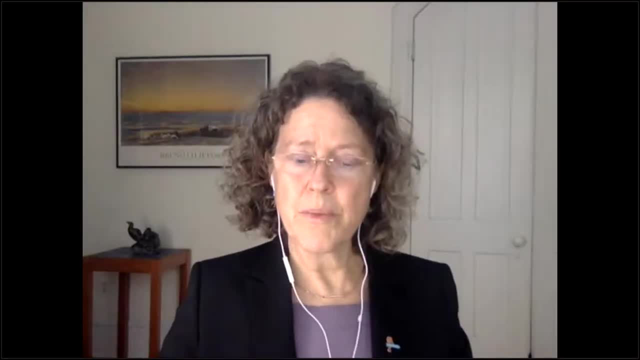 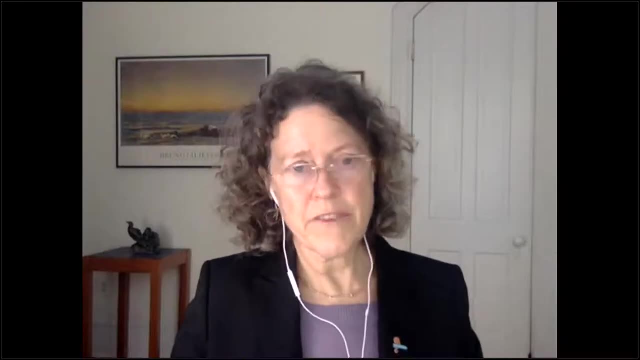 new agreement is fit for purpose. fifty years from now and longer, Lisa Levin will take us into the ocean with her current research on the effects of climate change on the ocean. Then Meinhardh Doughelle will explain all this. Meinhardh Doughelle will explain what the P-PCI-5ày finde in the ECA-109 agreement is, but then bystock, another piece of information. Meinhardh DoughElle will explain more deeply than ever in new terms of whole defense management. so there will be new and new movements on the issue of the PLO-PCI In the plante eres partido qe w expanding into Naje� máep tech presidencia en Christianity. 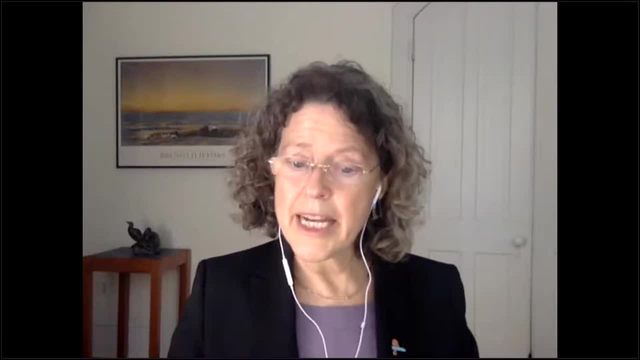 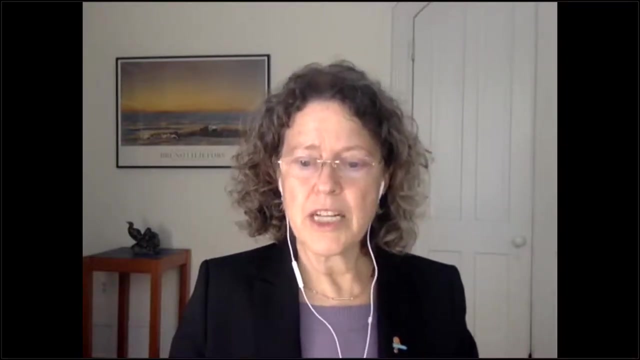 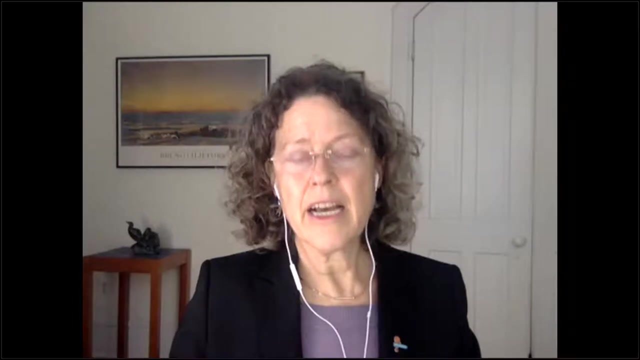 on the ocean. Then Meinhard Doell will explain how environmental impact assessment can be used to integrate information about cumulative effects, and the effects of climate change in particular, into project planning and approval, leading to recommendations for the BB&J text. Glenn Wright will present a case study of the mesopelagic zone. 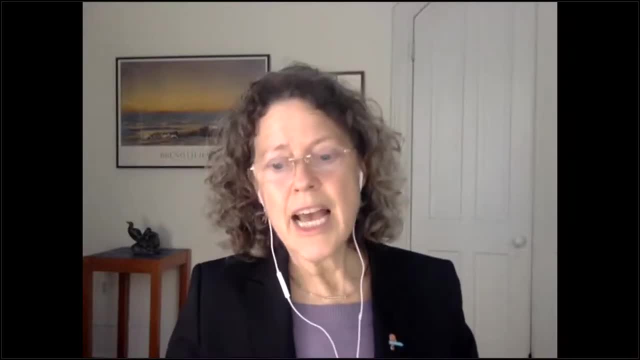 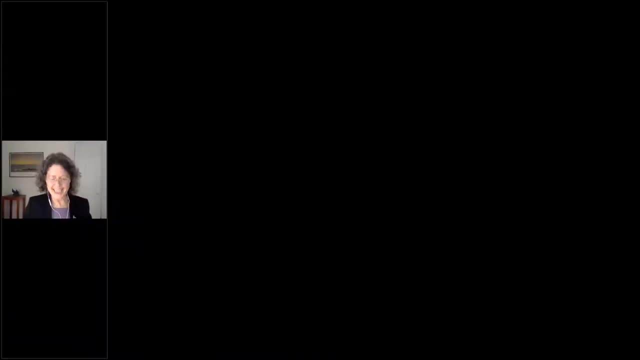 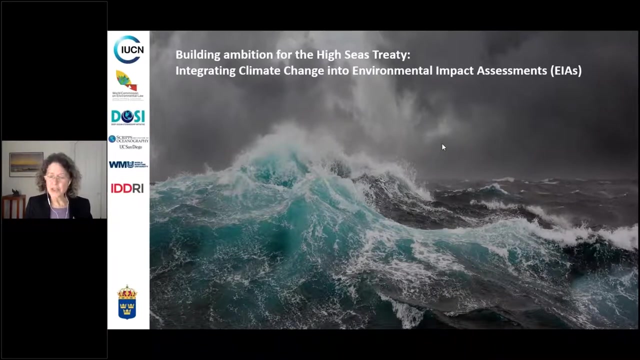 Kristina Gerda will join us for the Q&A session at the end, and you're welcome to type your questions at any time into the questions box, So please use it freely. Dr Lisa Levin I'd like to now introduce is the Distinguished Professor of Biological. 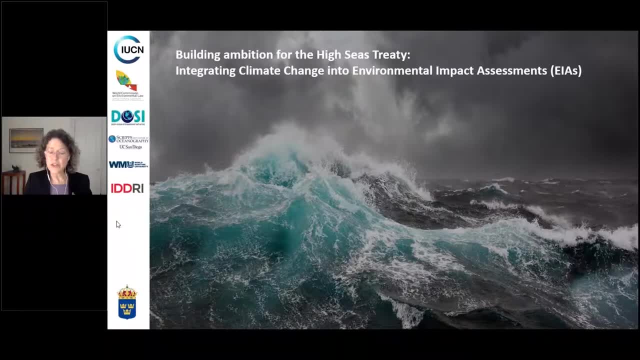 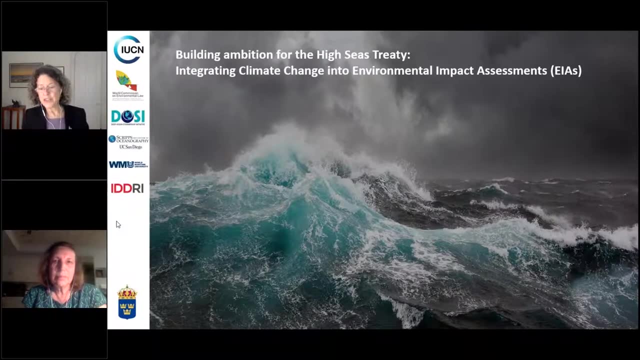 Oceanography and Marine Ecology at the Scripps Institution of Oceanography University of California, San Diego. She co-founded the Deep Ocean Stewardship Initiative, DOCE, which is a group that seeks to integrate science, technology, policy, law and economics to 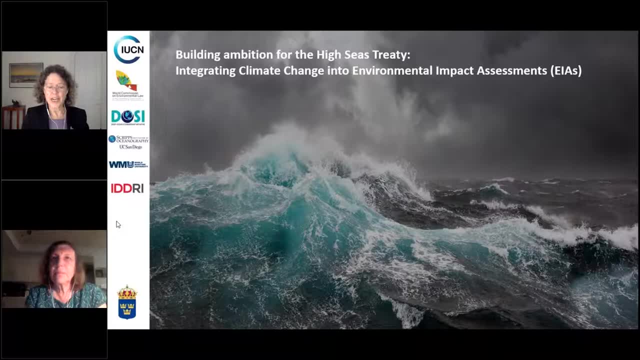 advise on the management of resource use in the deep ocean in order to maintain the integrity of deep ocean ecosystems. She also co-leads the Deep Ocean Observing Strategy, DOOS, which outlines the requirements for future deep ocean observations. Dr Levin is a fellow. 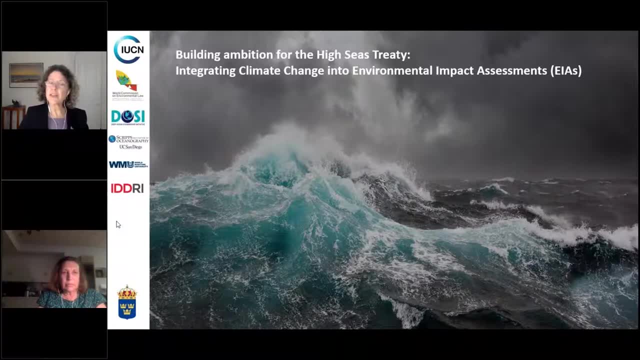 of the American Association for the Advancement of Science in the American Geophysics, and she's also a member of the Association for the Advancement of Science in the American Geophysical Union and received the Prince Albert I Grand Medal for Science for her work. 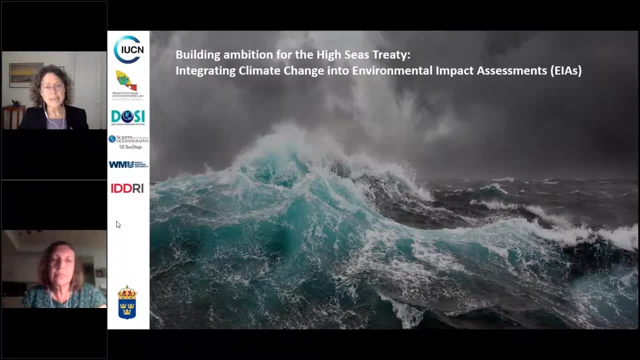 linking deep ocean science and policy, Particularly relevant today. she studies ecosystems subject to oxygen and sulfide stress, ocean acidification and ocean deoxygenation resulting from climate change, and contributes her knowledge to IPCC reports and at the UNFCCC Conference. 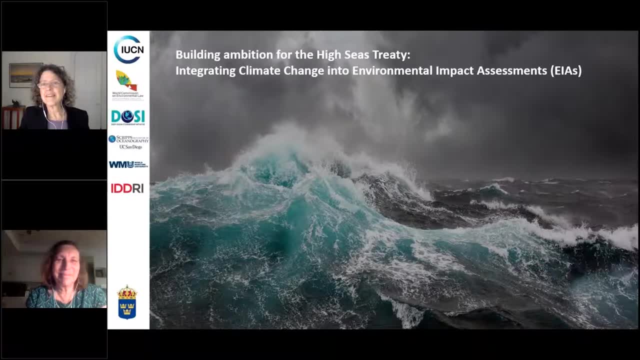 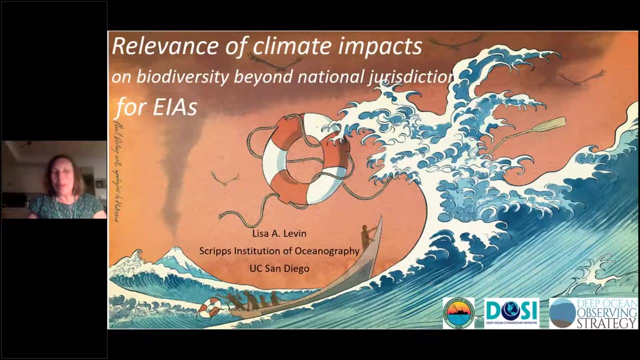 of the Parties, Lisa, over to you. Thank you, Hey, I'm hoping my slides. oh, there they are. Good day everybody. It's my pleasure to be able to talk to you about the relevance of climate impacts on biodiversity. 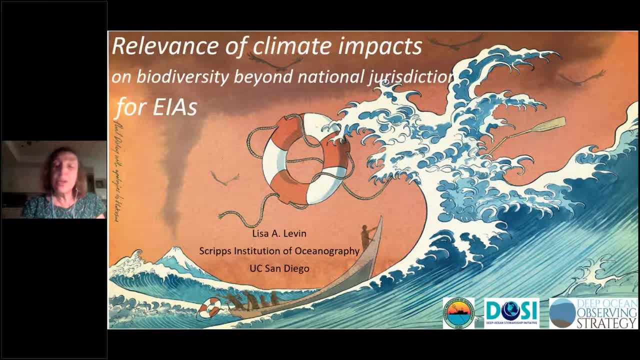 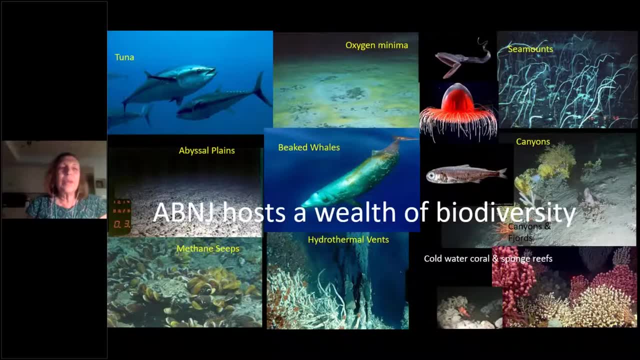 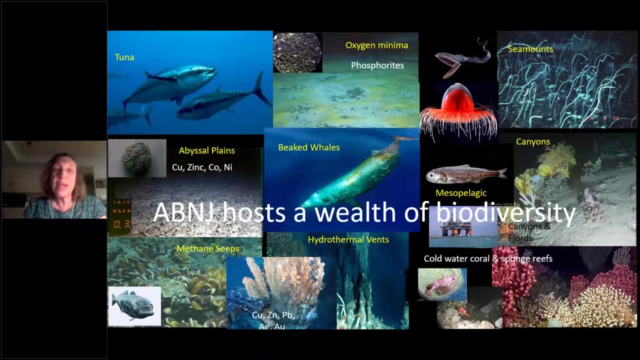 beyond national jurisdiction and how they are relevant to environmental impact assessment. Next slide: We know that areas beyond national jurisdiction host a wealth of biodiversity. This takes the form of tuna, whales, fish jellies in the water and a vast array of fascinating 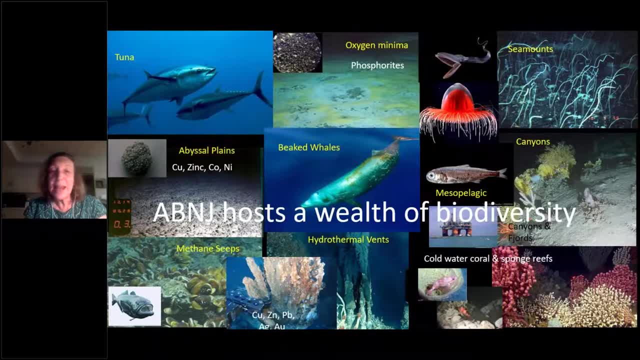 ecosystems on the sea floor, sea mounts, canyons, chemosynthetic ecosystems and biogenic habitats. We also know that these systems are associated with resources of growing commercial interest: minerals- I'm sorry, go back, please. minerals- fish. 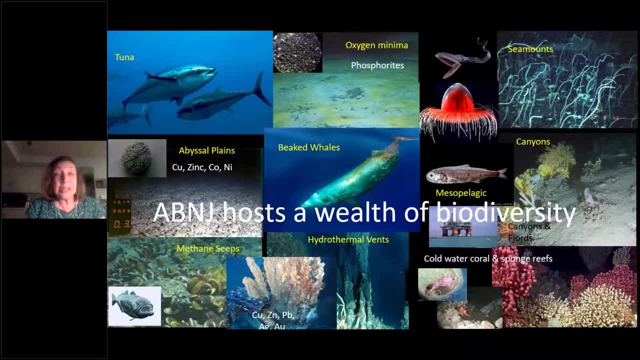 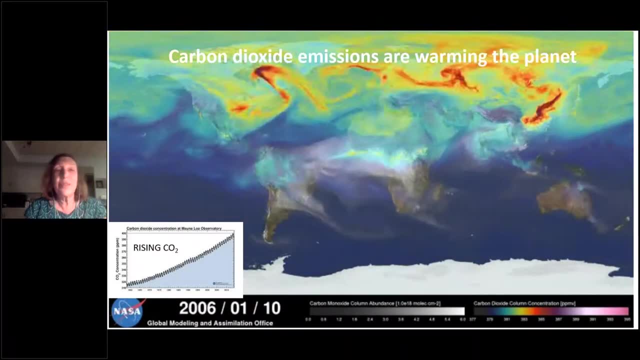 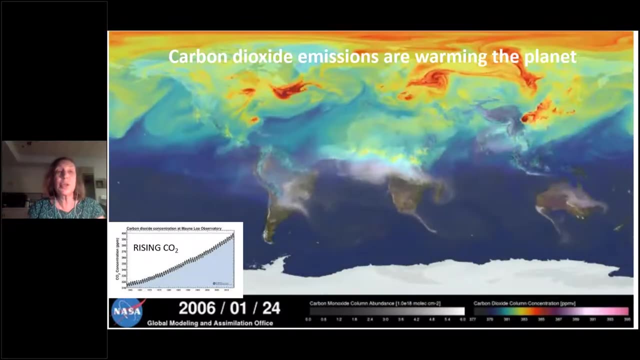 and energy and genetic resources. Okay, next, please. At the same time, we have humans emitting massive amounts of carbon dioxide into the atmosphere that are warming the planet, And although much of these emissions, as you can see, occurs in the Northern hemisphere, 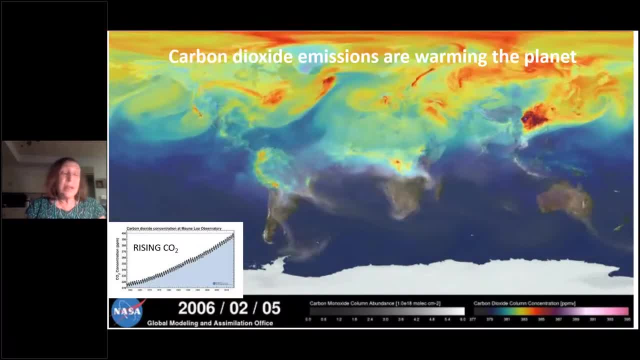 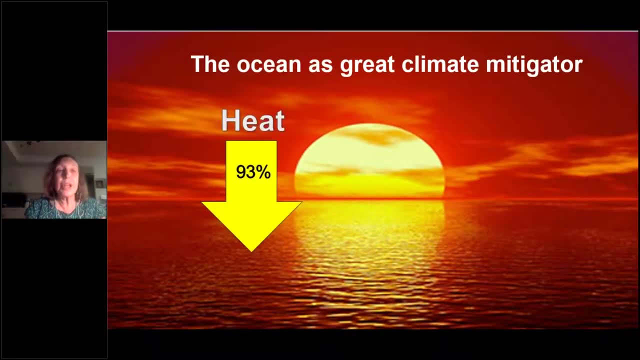 this affects the entire planet And the entire ocean. Next, please. About 93% of the excess heat generated by this carbon dioxide is taken up by the ocean, So our ocean is a tremendous climate mitigator. This heat leads to reduced oxygen solubility. 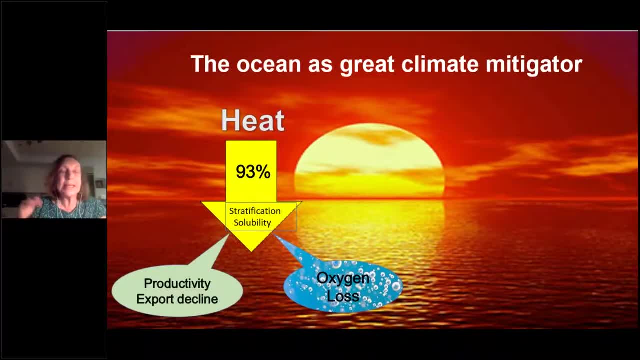 and increased stratification, That is, a reduced vertical mixing of the sea floor, And that leads to oxygen loss, of what we call ocean deoxygenation, And it also leads to reduced export of primary productivity from the surface to the deep sea through the water. 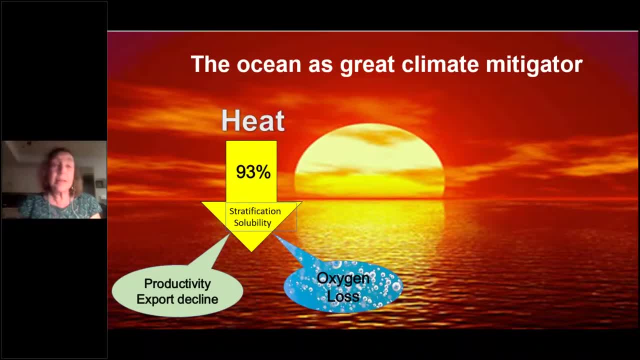 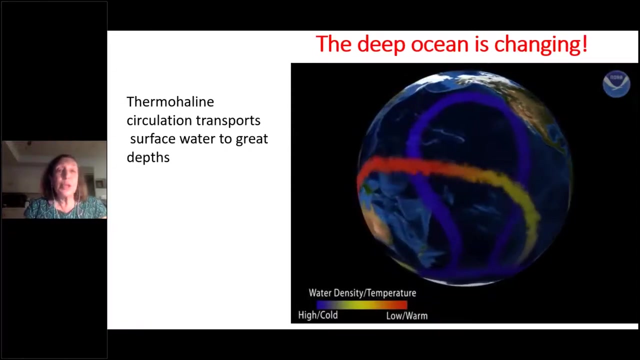 And so there's less food for organisms in deep water. Next, please, We know that the ocean takes up massive amounts of carbon dioxide- about a quarter of the excess carbon dioxide- And this leads to a phenomenon we call ocean acidification. Now, all these changes are happening at the ocean surface. 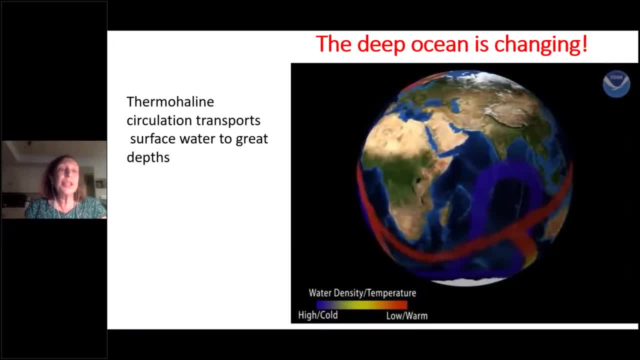 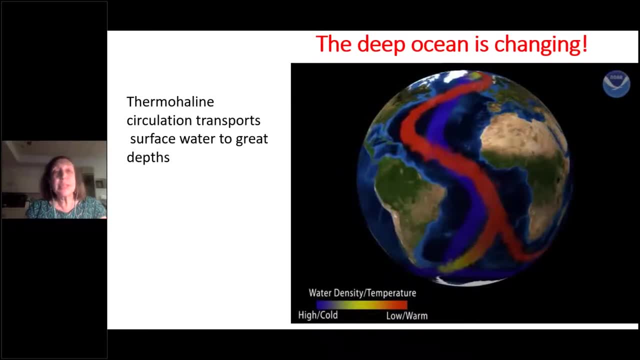 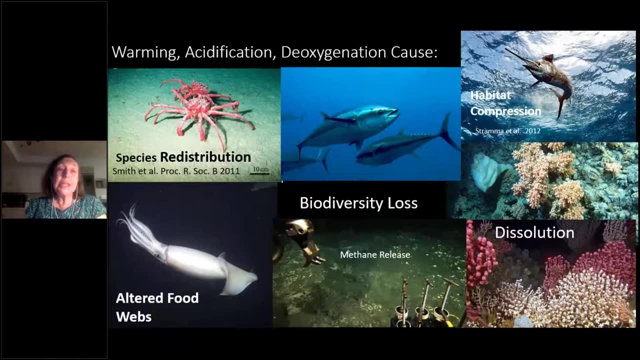 but they don't stay at the surface. Thermohaline circulation transports that more acidic, less oxygenated, warmer surface water to great depths, And so the deep ocean is changing. These changes- warming, acidification and deoxygenation- are causing redistribution of species. 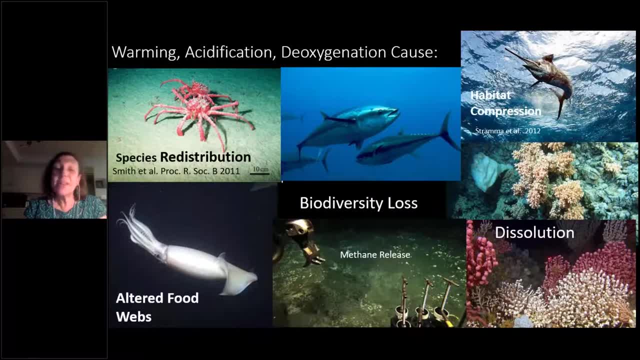 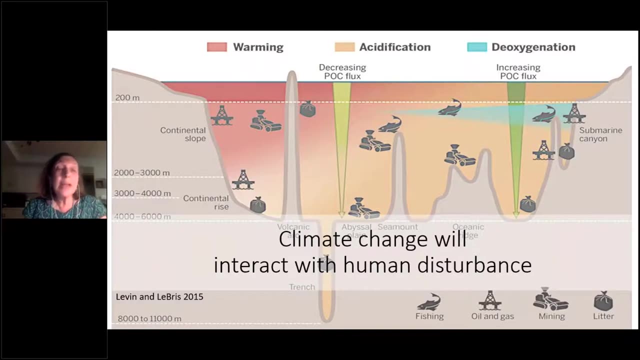 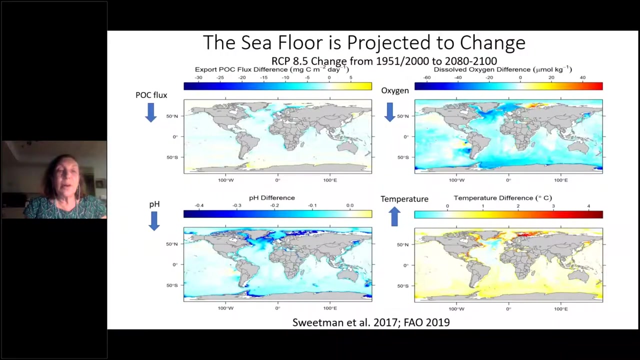 compression of habitats, changes in food webs, loss of biodiversity and, potentially, dissolution of our deep water corals. These changes, these climate induced changes, will interact with human disturbance in many different ways. Next, please, We know that there are massive changes occurring or projected to occur. 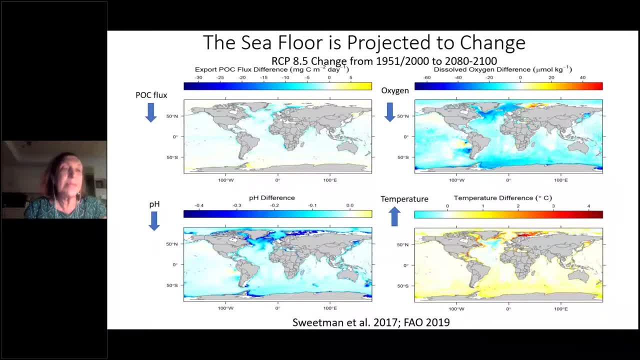 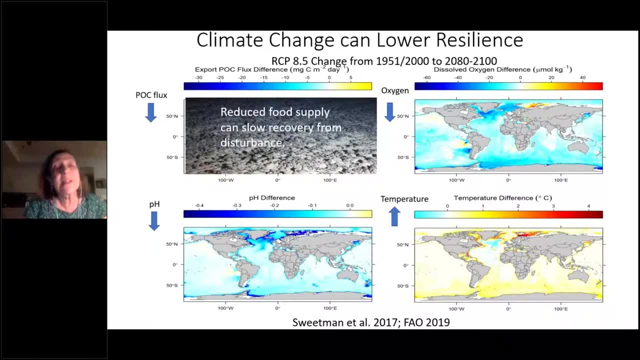 on the sea floor. For example, a reduction in food supply, POC flux leads to the reduced leads to less food on the sea floor and potentially slower recovery of animals from disturbances like seabed mining or bottom fishing. We know that massive areas of the open ocean 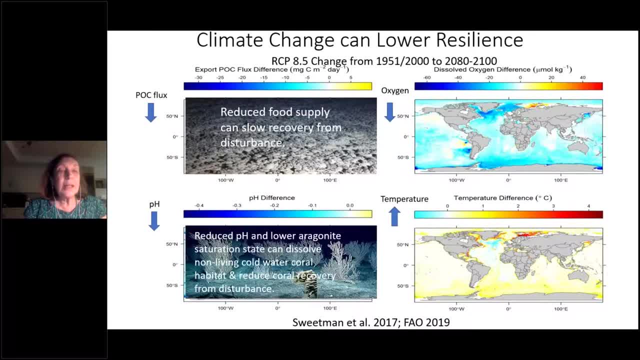 are subject to declines in pH And that decline leads to, which is associated with lower aragonite saturation, can dissolve non-living cold water corals and actually slow the recovery time of corals from disturbance. Large areas of the deep ocean experience declining oxygen. 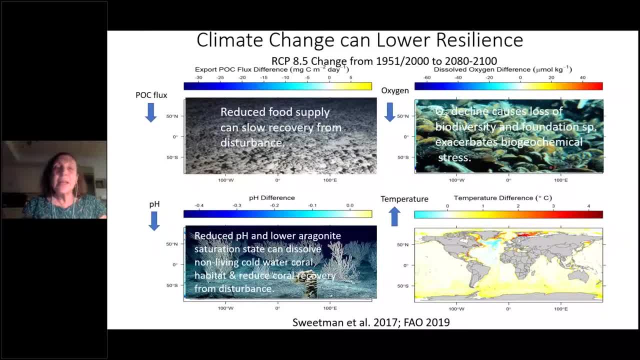 And this leads to next, please. It leads to loss of biodiversity and loss of foundation species and exacerbated biogeochemical stress, And we know that warming temperatures over much of the ocean leads to rising metabolic rates and the redistribution of species and of different kinds of biogenic habitats. 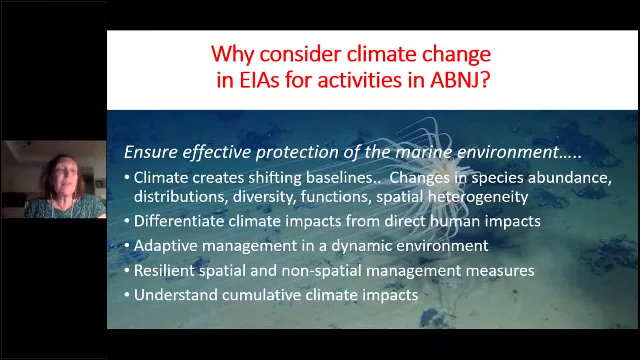 So why might we consider climate change and development of environmental impact assessments in ABNJ? Well, I would argue this is a necessary to ensure effective protection of the marine environment. Climate changes, the climate creates shifts and shifting, I should say climate change- creates shifting baselines. 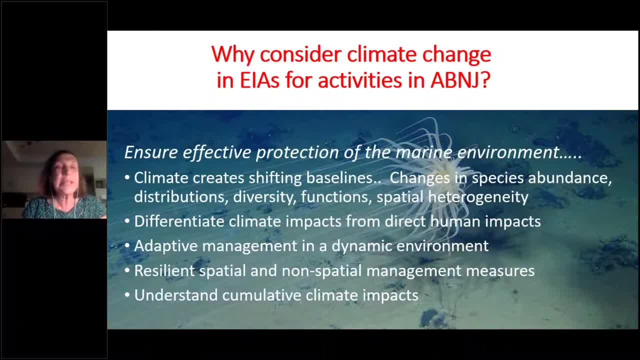 with changes in species abundance, distributions, diversity, functions and spatial heterogeneity. We need to understand climate change, to differentiate climate impacts from direct human impacts, to enable adaptive management in a dynamic environment, to create resilient spatial and non-spatial management, and to understand cumulative climate impacts. 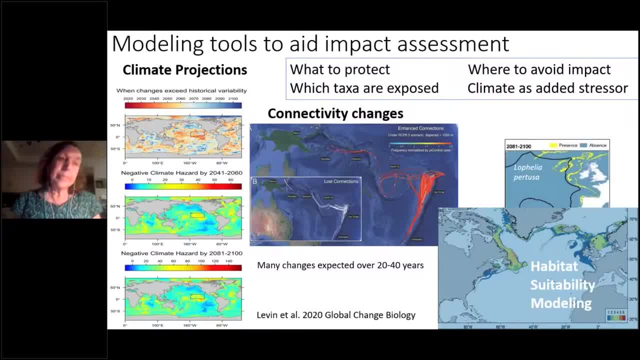 to create resilient spatial and non-spatial management and to understand cumulative climate impacts. We have a host of different modeling tools that can aid us in doing this. We have climate projections into the future that can tell us which areas will exceed natural variability and when. 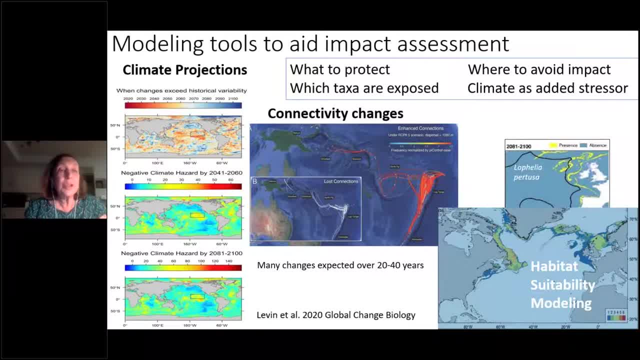 And we can look at cumulative climate hazards in combination with models that project changes in connectivity and changes in habitat suitability, And together these models can tell us what to protect, which tax are most exposed to climate change, where to avoid impact and how climate might act as an added stressor. 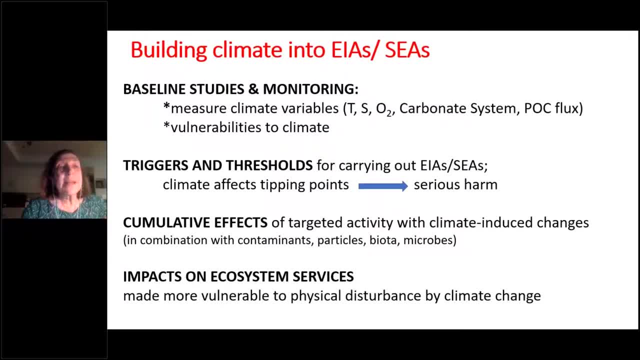 So to build climate into environmental impact assessments, we need to incorporate it into our baseline studies and monitoring. We need to consider climate in developing triggers and thresholds for carrying out EIAs. We need to consider climate as a cumulative effect and we need to understand how climate impacts can affect the environment for multiple purposes. 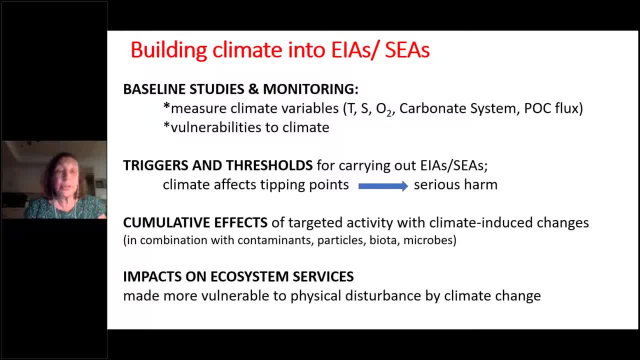 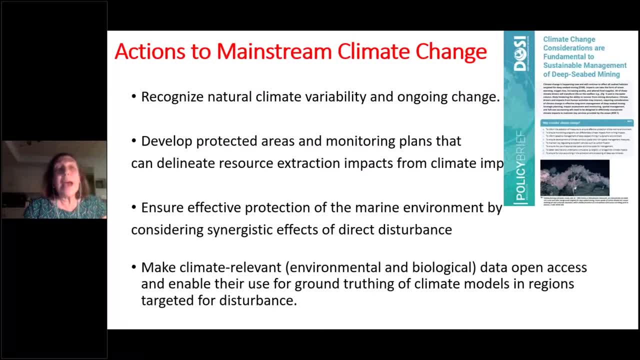 understand how climate impacts ecosystem services and so what kinds of actions can we take to mainstream climate change? we need to recognize that natural climate variability and ongoing change are happening and part of the ocean in areas beyond national jurisdiction. we need to develop protected areas and monitoring plans that can delineate resource extraction impacts from climate. 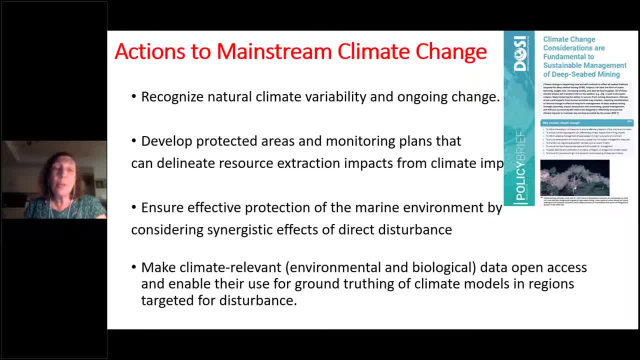 impacts. we need to ensure effective protection of the marine environment by considering the synergistic effects of direct disturbance. and then, finally, it's very important that we meet, make climate relevant data open access and enable their use for ground truth and climate models and other kinds of models in 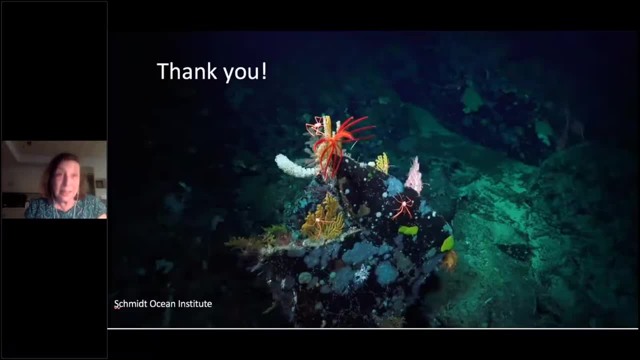 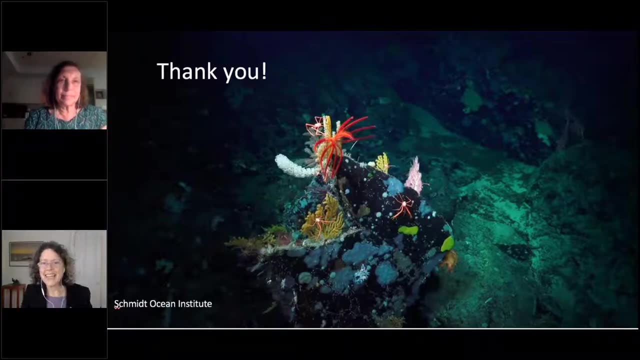 regions targeted for disturbance, and with that, I'd like to thank you all for listening you. Thank You, Lisa. that was a wonderful presentation. you've made it clear that the oceans health is essential to climate change mitigation and that it's vulnerable to climate change stress in multiple ways, but that we can provide. 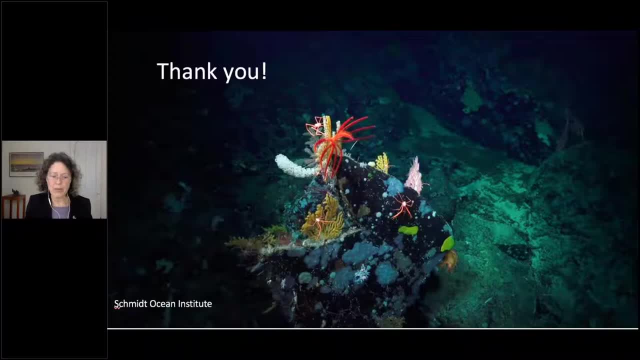 some protection for ocean systems if we carefully manage our human activities that affect it, and a number of the points you've made about the science are going to be quite relevant both to the intersection of the ocean and the ocean's environment and to the international discussions just finished and the ones coming up. this in the next. 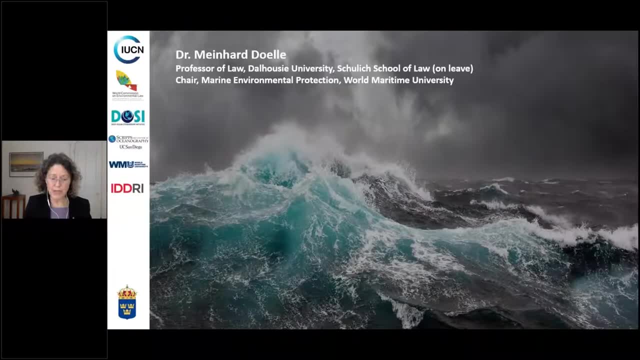 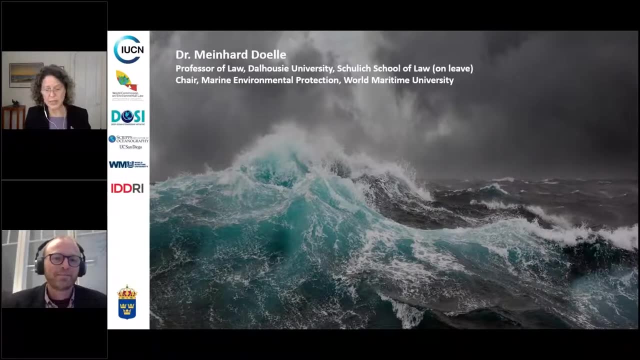 couple of months. so I'd like now to introduce my heart dwell professor. mine heart dwell is the Canadian chair and head of ocean sustainability governance and management at World Maritime University. he's also a professor at the Schulich School of Law at Dalhousie University. he's advised governments in 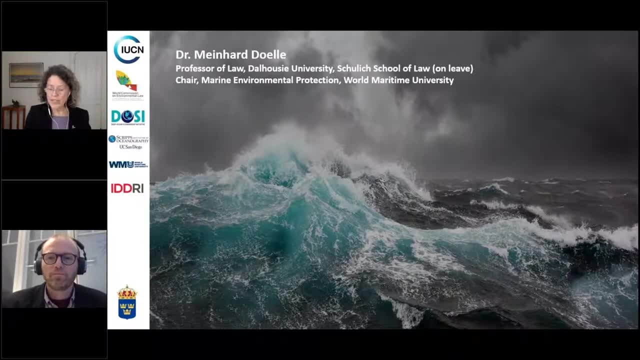 Canada on environmental assessment. contributing to drafting environmental assessment was at federal and provincial levels. he's overseen several project and strategic EIA processes and writes extensively on both climate change and environmental assessment. mine heart, please tell us how we actually go about learning lessons for the EIA sections of the BB and J. 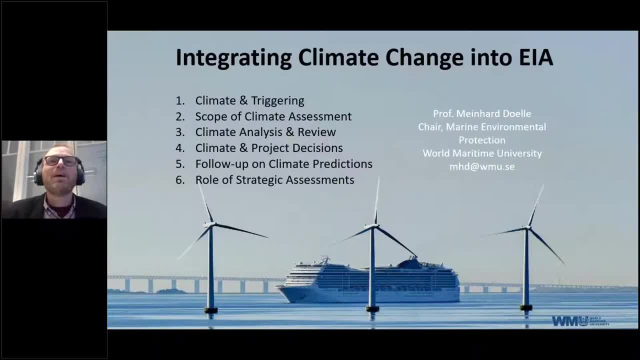 agreement thanks. thank you, Sydney. so time is short, so let me give you a three key messages upfront, in case I run out of time in the end. So my first key message is that the consideration of climate change is critical for effective environmental impact assessment. We cannot afford to ignore this critical issue in the EIA process. 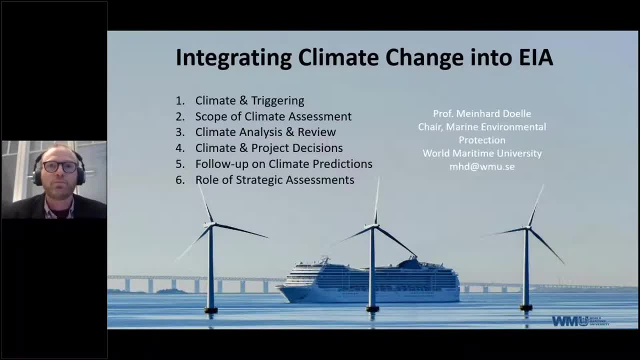 and I think this was very well illustrated by Professor Levin's presentation. The second point is that it is important to recognize that there's growing experience with the integration of climate change into EIA in many domestic EIA processes and also a growing academic literature to draw on. So the BB&J regime has experience and ideas that it can draw on. 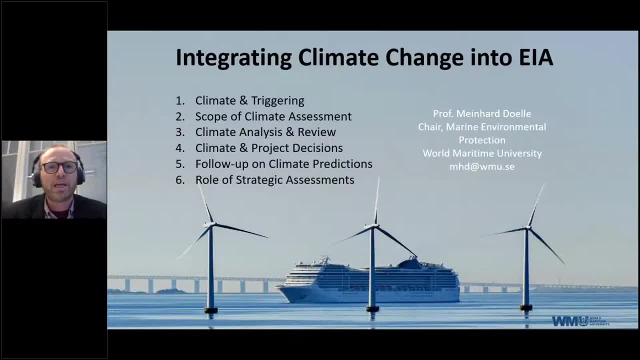 The third one is that the key climate issues to include in an EIA are. there are four of them. The first is greenhouse gas emissions associated with a given project. The second are projects in the EIA. The third one is that the key climate issues to include in an EIA are. there are four of. 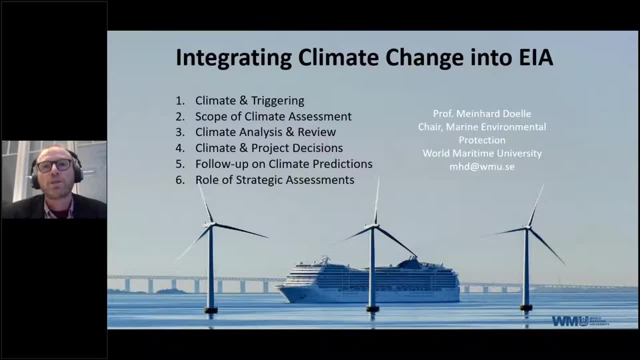 The first is greenhouse gas emissions associated with a given project. The second are projects in impacts on climate, sinks and reservoirs. The third is the interaction between project impacts and climate impacts on ecosystems and their resilience. And the fourth is the impact of climate change on a proposed project. So in the time that I have, let me just briefly touch on. 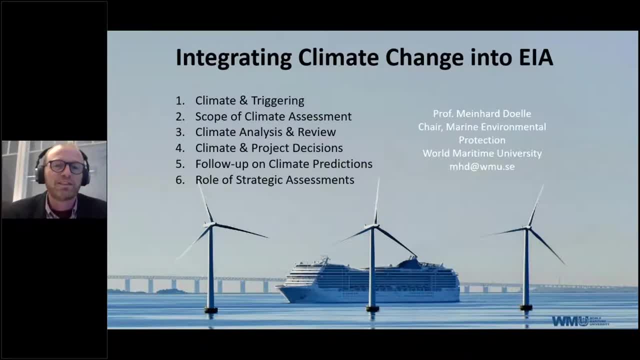 a number of the issues associated with this, in light of the six elements of environment look-back assessment that are on the slide that you have in front of you. So I'll start with triggering, because triggering is, of course, a key part of the assessment process. So, with respect to 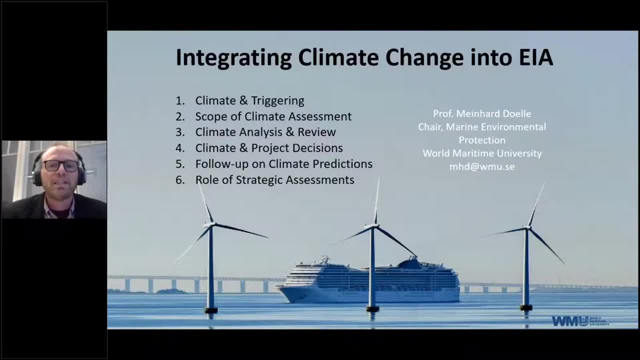 integrating climate change into EIA. the key issue here is: to what extent should climate consideration affect whether a project gets assessed, And there are three basic climate triggers that have been utilized and that should be considered. One is essentially a greenhouse gas emission trigger, So that's either annual project emissions, project life. 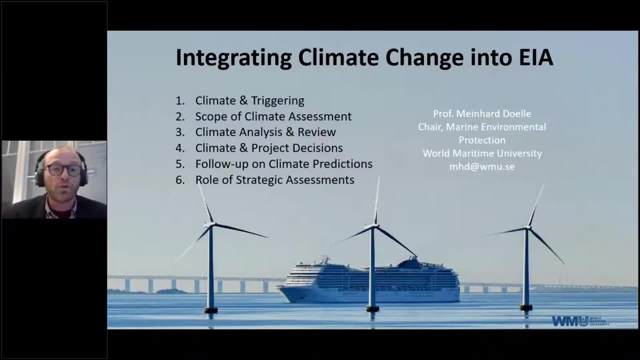 cycle emissions or a combination of those, So thresholds associated with the emissions of the project. The second is to what extent the proposed project poses a risk to ocean sinks and reservoirs. And the third would be what I call a type of activity trigger, So where you trigger. 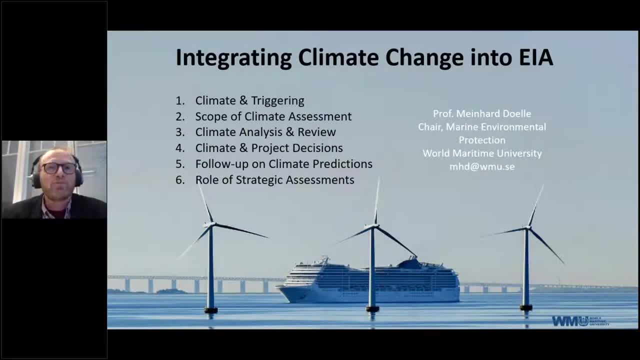 a project just because of the type of project it is. it's associated with significant risks, such as oil and gas development, for example, And most domestic processes that have considered climate change as a trigger have worked with a combination of these approaches. So the second 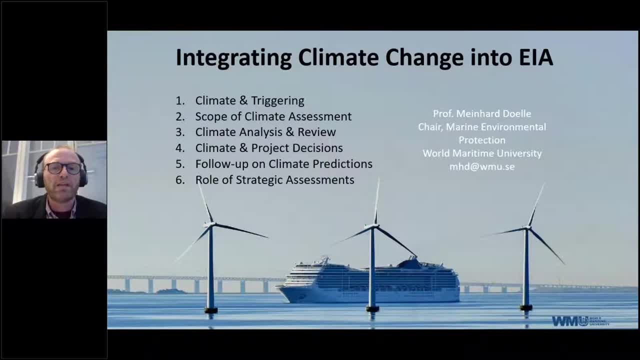 issue, then, is scope, the scope and the climate consideration, So there's really three, I think, issues to consider. to begin from, One is: what is the scope of greenhouse gas emissions to consider in the assessment, And many jurisdictions have played around with this idea of scope 1, 2 and 3 emissions. where scope 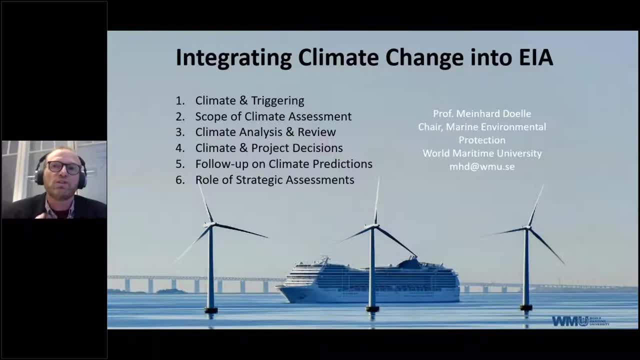 one emissions are emissions that are directly associated with the project. scope two emissions are emissions embedded in energy and other material used for the project and scope six are emissions targeted to the project. All the other issues would the three would might be rid отпositedies within part of the project. 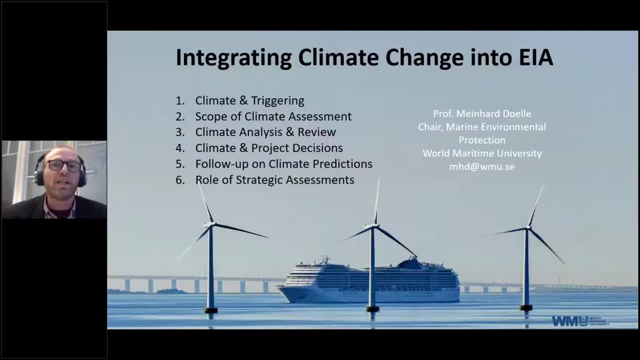 three emissions are indirect emissions that are enabled by a project, such as upstream or downstream emissions. And then you have to consider the scope of impacts on ocean sinks and reservoirs and the scope of the interaction between project impacts and climate impacts on affected ecosystems. And my final point on scope and information gathering is that it's 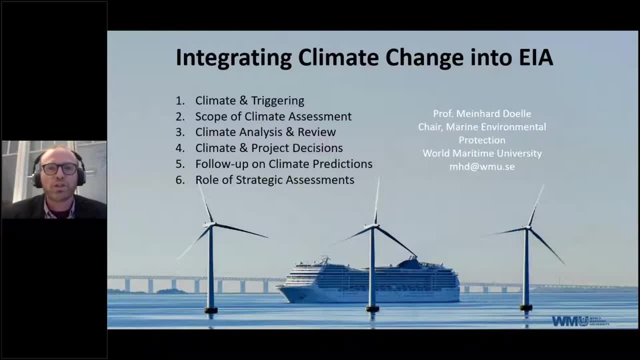 important to recognize- and there's a growing recognition in the EA literature certainly- that all impacts are cumulative. So when we talk about this challenge of doing cumulative impact assessment, we have to recognize that all project impacts, all impacts of human activities are cumulative. And so then we move to analysis and review. We start with the gross emissions of 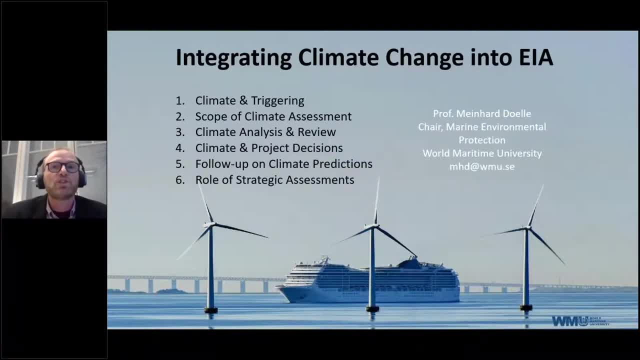 the project We have considered. we then consider what are the net emissions. So to what extent do the emissions impact the project? And then we have to consider the impact of the project, And then we have to consider the impact of the project, And then we have to consider the impact of the. 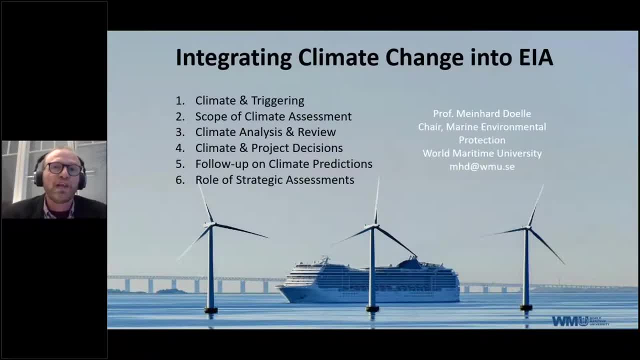 emissions from a project, displace or reduce emissions elsewhere? What do the emissions tell us about the project's effect on efforts to decarbonize? Does it help those efforts? Does it hurt those efforts? What effect does the project have on the resilience and effectiveness of ocean? 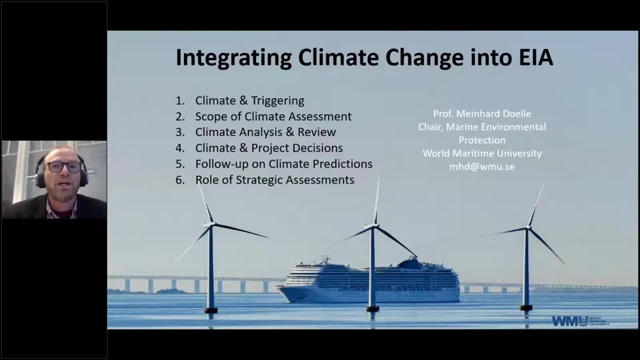 sinks and reservoirs, which is critical, of course, in the high seas. And what do we know about the risks and uncertainties, of the predictions that are being made about these impacts And one of the key messages there that many jurisdictions are now realizing and coming to? 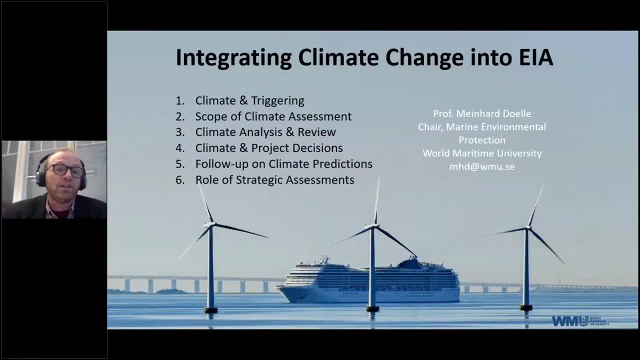 deal with is the need to work with different scenarios, And a simple example of that is different scenarios about the level of mitigation and the associated climate impacts. that results from different levels of mitigation efforts globally. We then get to decision making, where we then consider the project's impact on decarbonization efforts. 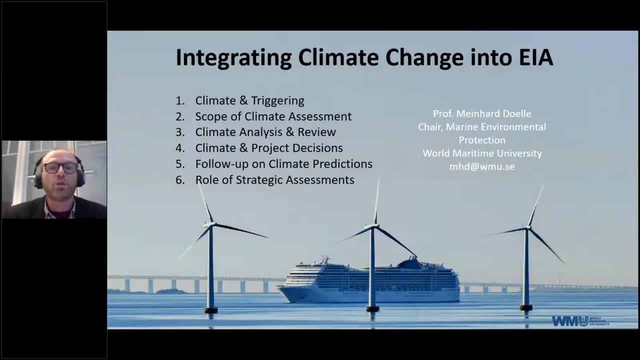 consider whether the project supports or undermines the resilience, viability and effectiveness of ocean sinks, and recognizes that decisions are being made in the face of risks and uncertainties. And then, often forgotten, is the post-decision phase, where we track compliance with terms and conditions, where we track accuracy of predictions about greenhouse gas emissions. 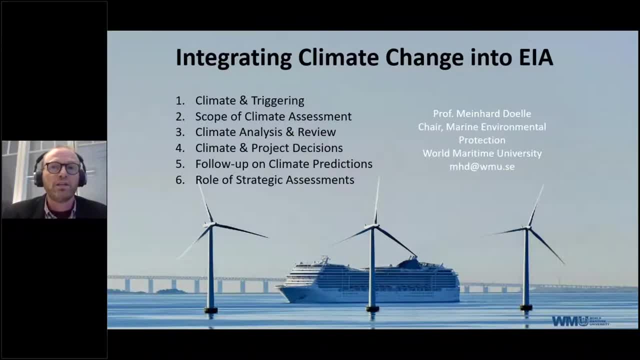 and where we track accuracy of predictions about greenhouse gas emissions. And then we do that both to learn for future assessments but also to make adjustments to the terms and conditions under which projects are approved. And that leaves me with my final point, and that is the role of strategic assessments, And I include in the concept of strategic. 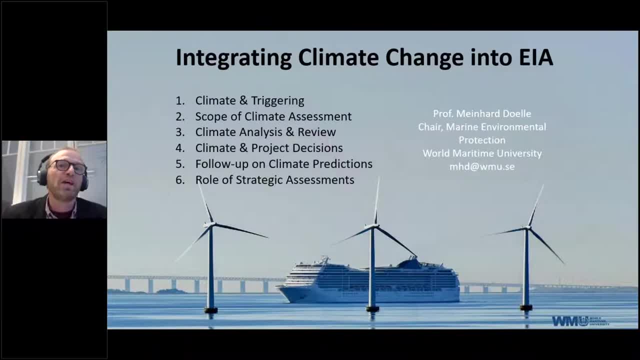 assessment, regional assessments, And I just want to make the point that some of the challenges that are associated with cumulative effects generally, and dealing with climate change, environmental impact assessment in particular, are difficult to resolve at a project level alone. So doing strategic and regional assessments in particular are critical to enhancing climate. 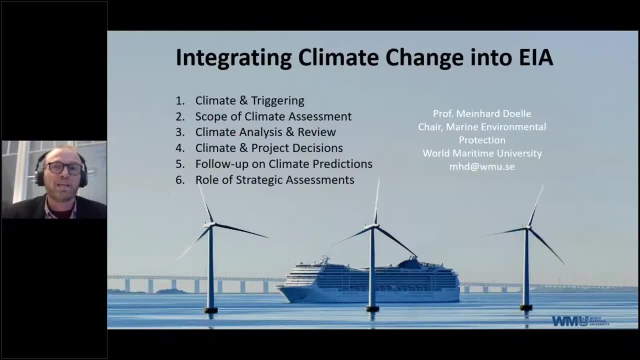 triggers and dealing with cumulative effects analysis at the project And, of course, both regional and strategic assessments are particularly important for high-risk activities such as geoengineering, extractive sectors- new sectors that have come along- and for preventing loss of productivity of climate sinks and reservoirs. And I'll leave it at that for 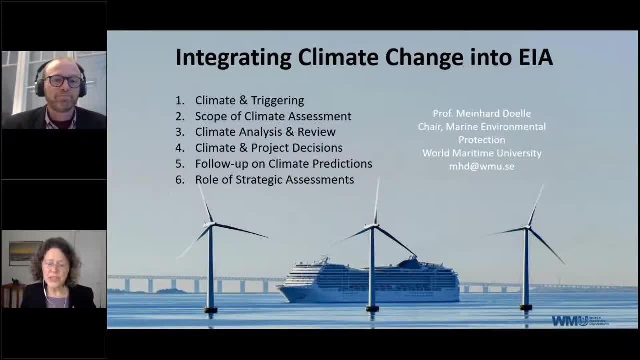 now, Thank you. Thank you so much, Meinhardt. I think that you have laid out a clear path, based on experience, for how to integrate climate change into different aspects of project assessment, and that, I think, will be very reassuring as we go forward and think about how to. 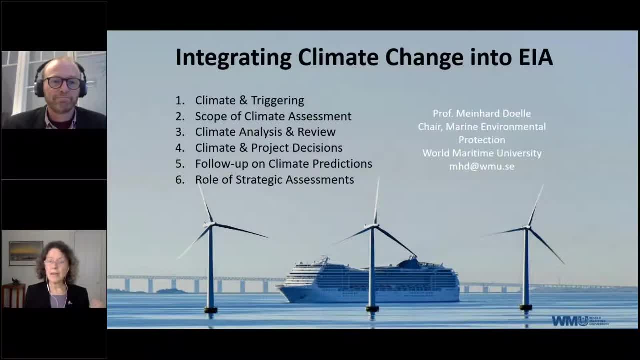 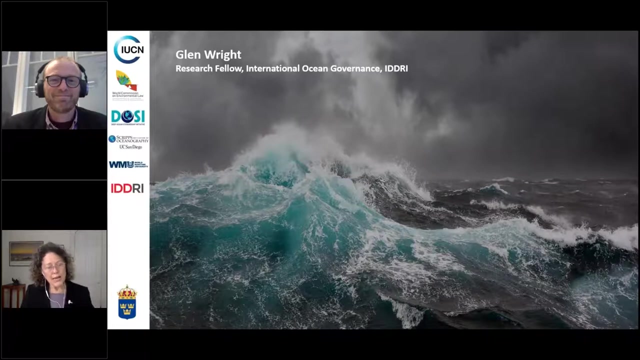 do this as an international community. I would also like to remind the audience that in the poster you'll see links to some of Meinhardt's writing and to Lisa's Ravel talk that you might find interesting if you haven't been taking close notes yourself. So our next speaker will be Glenn Wright. 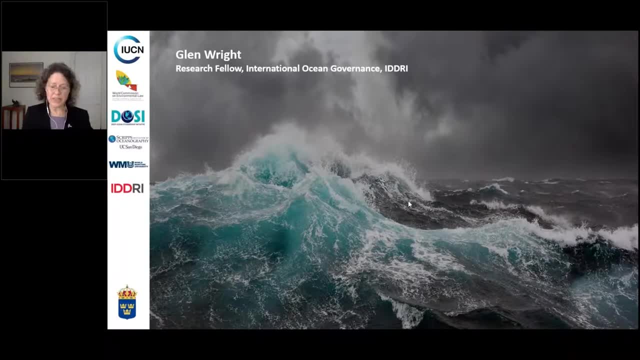 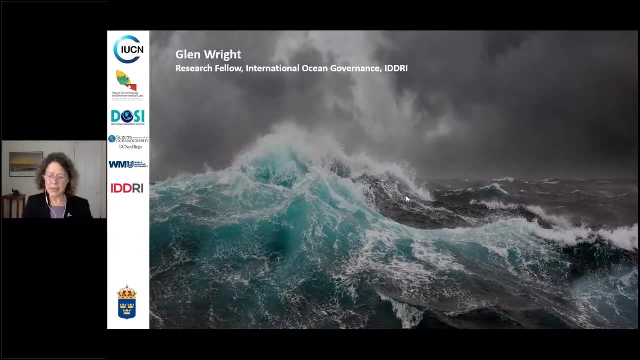 Glenn Wright is a senior researcher at the for Sustainable Development and International Relations, IDRI, based in Paris. At IDRI, he has authored many exceptionally useful publications on marine policy and ocean governance. My personal favorite is The Long and Winding Road to BB&J, a must read to understand the negotiation. 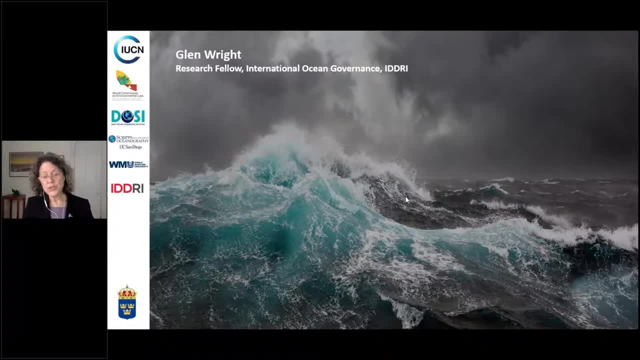 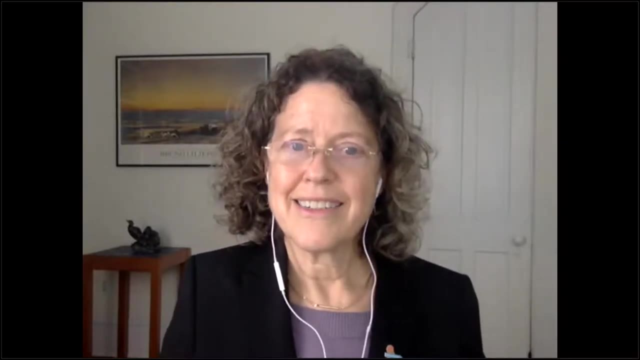 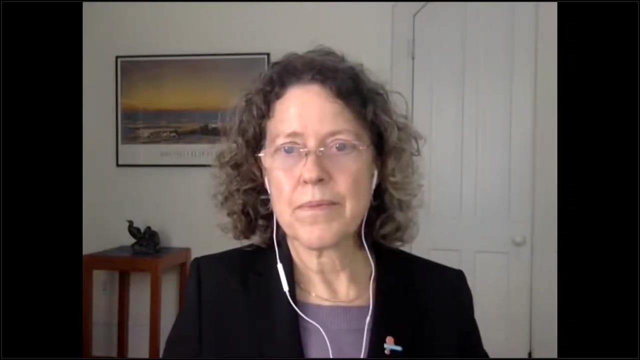 He also runs Little Blue Letter, an uplifting ocean newsletter curated each week by a young leader in marine science and policy. So, Glenn, would you join us and tell us a bit more about the Mesopelagic Zone? So the Mesopelagic Zone is a part of the ocean. 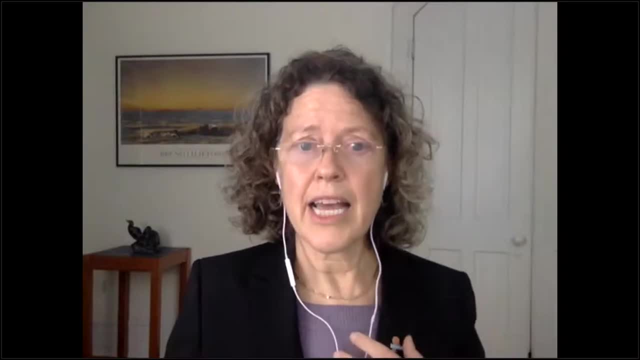 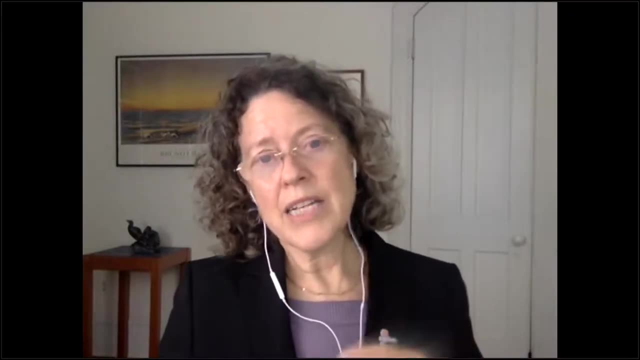 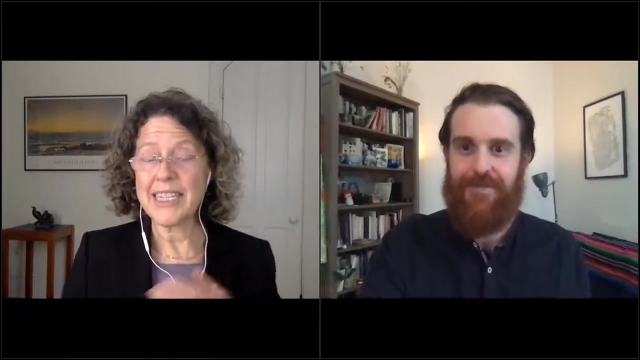 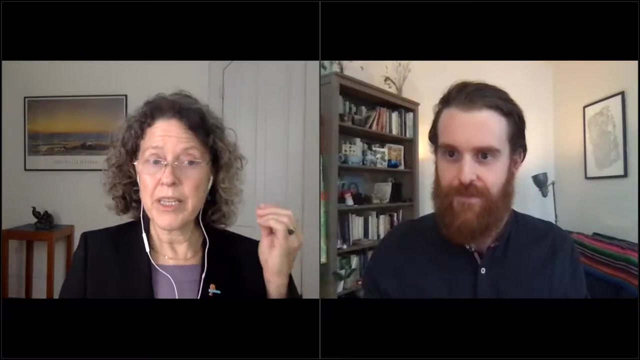 that is only recently been studied and it is an area there for a particular interesting concern as we develop regulatory tools, governance tools, And so it'll be really wonderful to have Glenn take us into that zone and help us understand how EIA and climate change can be addressed there. 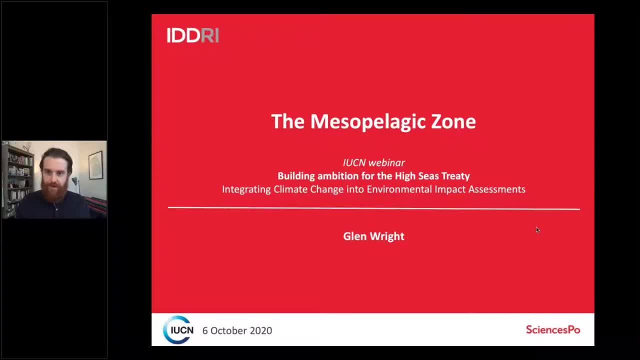 Thank you. I'm hoping that you're now able to see my slides. Someone could confirm You can see them. Fantastic, Wonderful, That brief moment of panic there when the settings dialogue box popped up and told me I wasn't allowed to show you my slides. 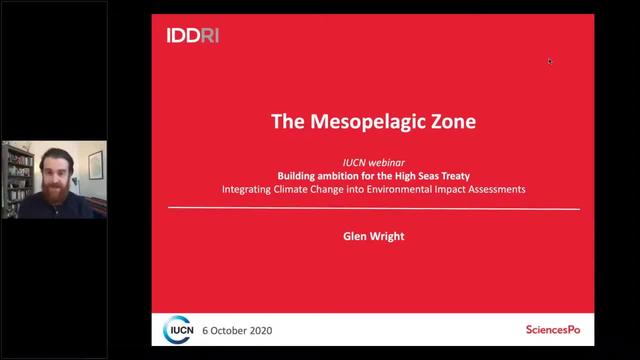 and I would be somewhat lost without them. This is a subject, actually, that is relatively new to me and to the work that we do at IDRI, And so it's quite exciting for me to be able to give this to you, And so I'm looking forward to where you will be, I think, in a few weeks. 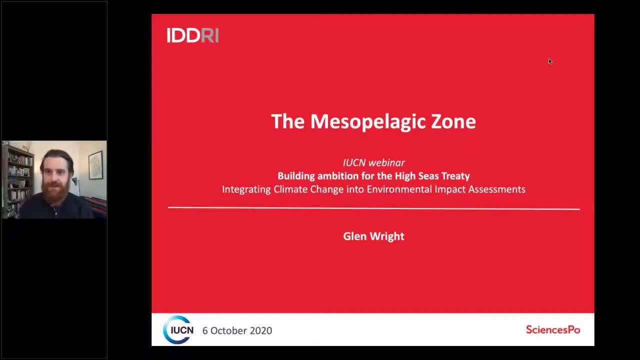 Okay, give this presentation in the context of the high seas negotiations, and what I'll try to do in this presentation is: I don't have time to go into a huge detail on the mesopelagic zone, possible future development of fisheries and the regulatory framework, but I would like to give some idea and 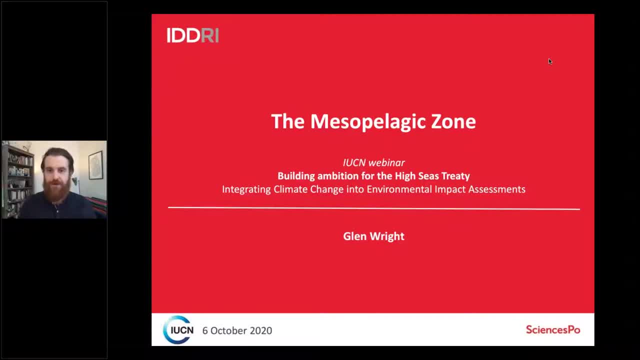 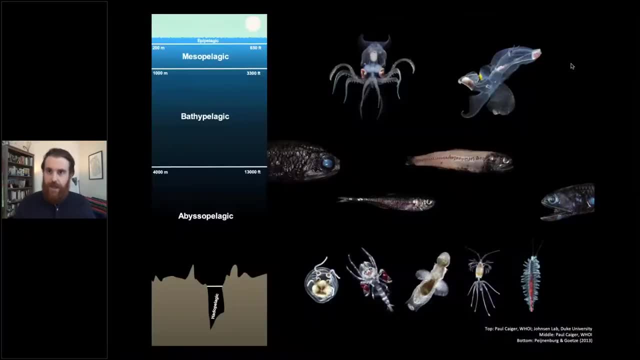 some concrete example about how a new agreement could affect impact assessment and using this as a case study. so if you haven't had the pleasure of seeing some of these sorts of images before from the mesopelagic zone, it's a vast ocean realm that very little light reaches, and it's 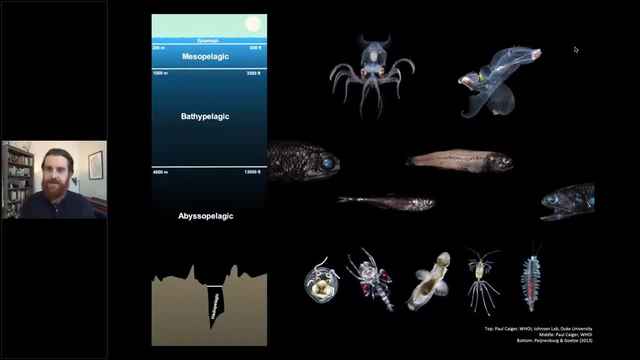 approximately 150 to 1500 meters of depth, and it's dominated largely by the kinds of organisms you see at the top and cephalopods, siphonophores, but there are also huge quantities of fish you see in the middle here examples of different species of lantern fish and then of 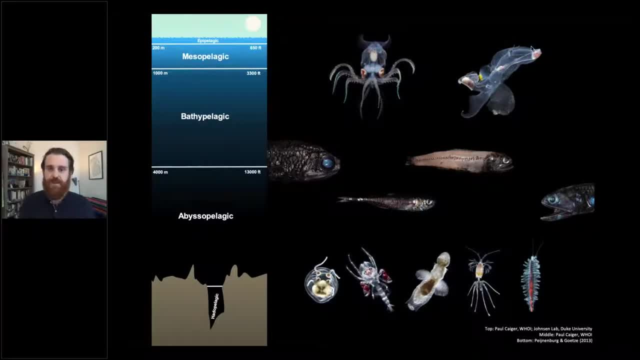 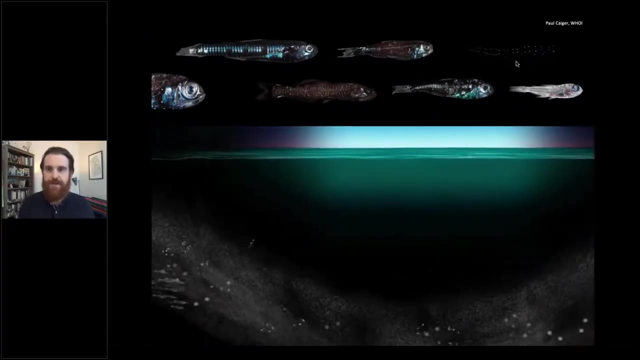 course, interesting plankton and other other creatures. it's a highly connected ecosystem and these are the aspects that we're just starting to learn more about in terms of marine science. I'm hoping the animation that you see on the screen works, but what this shows is the huge migration. 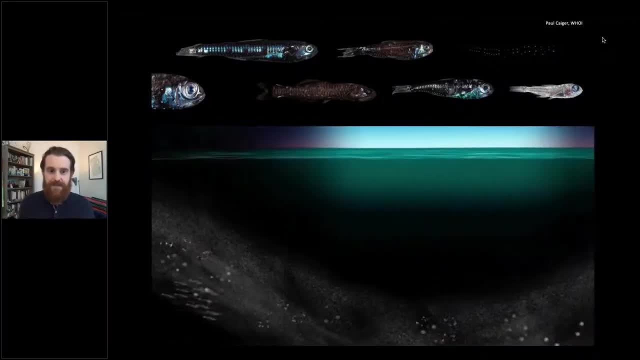 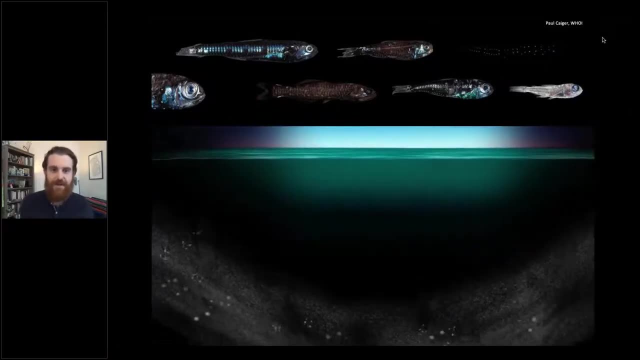 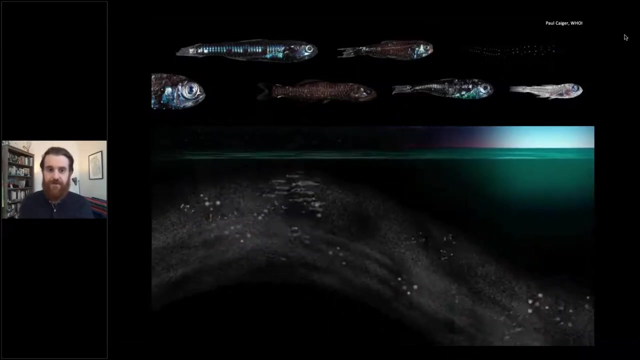 that happens overnight every day, from lantern fish and other organisms that come up from the bottom as the Sun goes down. they're less liable to be eaten by predators, so they come up to the surface to feed, and in doing so, what they do is bring a huge amount of minerals and nutrients from the bottom up to the surface. 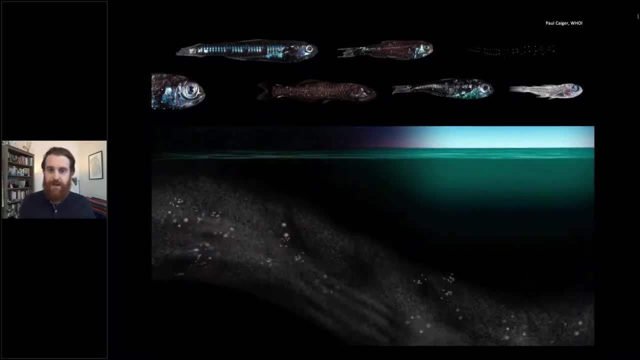 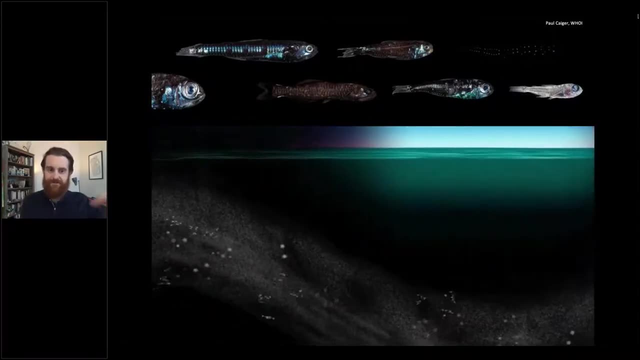 and vice versa, and they also, in doing so, play a huge part in the global carbon cycle. so essentially everything that that sort of begins at the top layer of the ocean passes through the mesopelagic zone eventually on its way down to the bottom of the ocean, where eventually, things 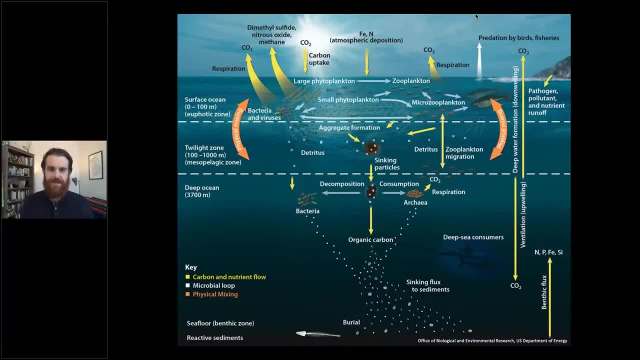 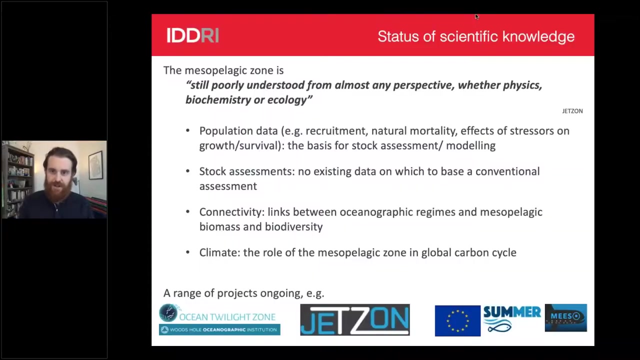 get stored as carbon. so this is a very busy diagram but just essentially showing, showing those different aspects, so how these different zones are connected and, in particular, how the mesopelagic zone connects things like primary producers, like plankton, to higher level predators like tuna, for example. so it's a very brief introduction of the mesopelagic zone and the 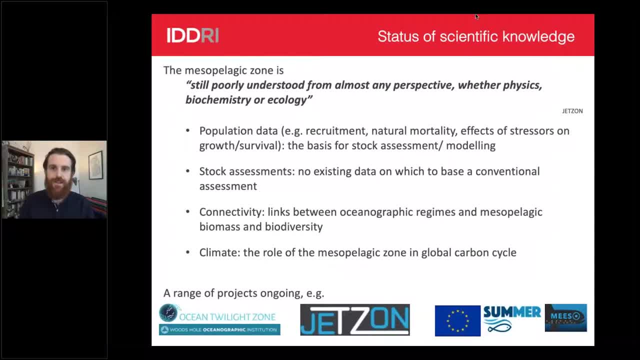 ep: 0 19 0iva. 0, 20, 0, 21, 0, 23, 0, 25 0 26. we would normally use for stock assessments and modelling. We just don't have that kind of information yet, But there was a huge amount of scientific research ongoing, Woods Hole. 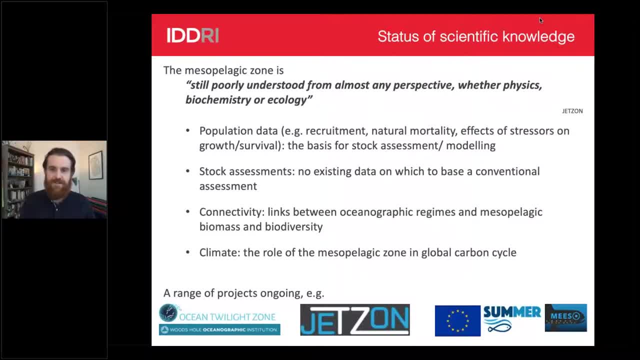 whose photos I've used extensively here, have an excellent Ocean Twilight Zone project, which is looking at these ecosystems. There's Jetson, which is a collaboration between various organisations, and the EU is also currently funding a couple of large-scale projects that are looking to improve the science space, improve scientific knowledge, but also starting to look at possible. 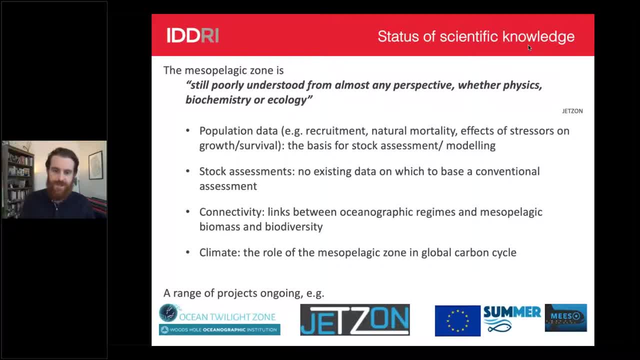 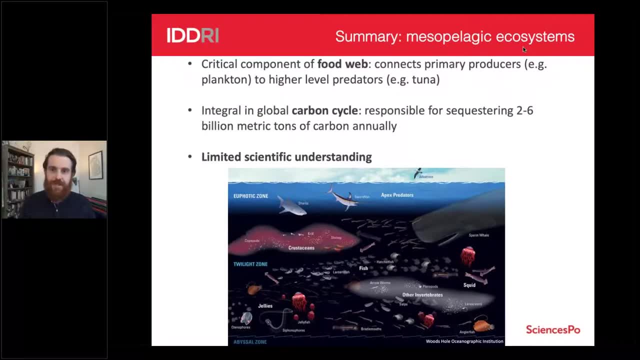 exploitation of this zone for fisheries resources, which I will come on to shortly. So just a sort of summary of the critical points. I mean I would emphasise the limited scientific understanding It really is developing. We still have a lot to learn about this zone and 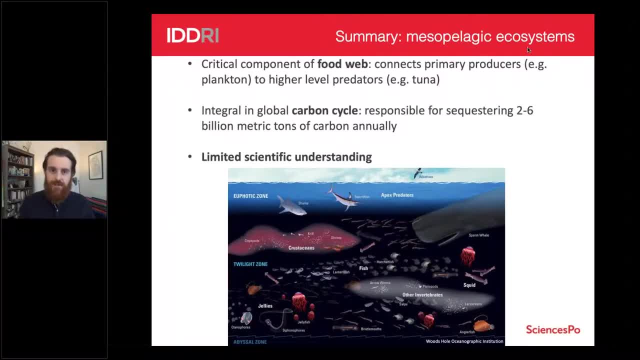 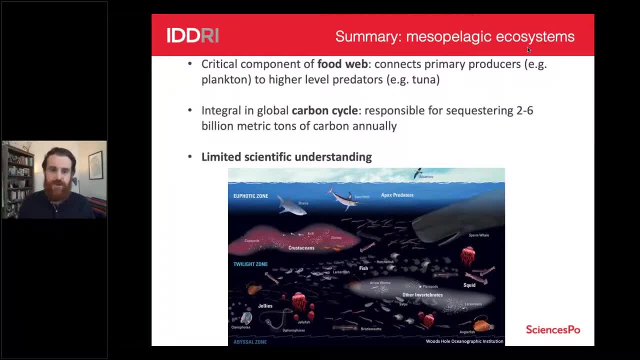 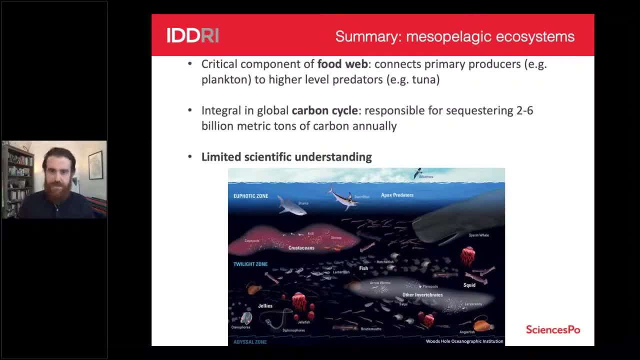 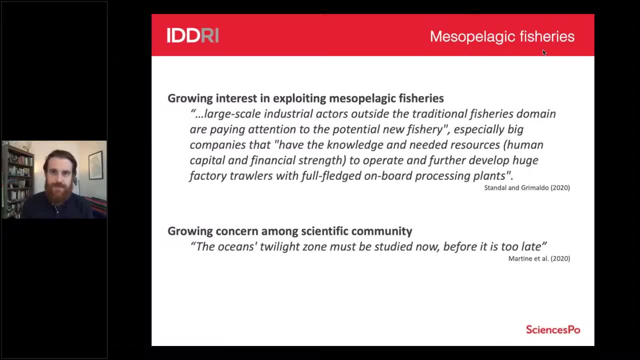 important role in the global carbon cycle. So that's just to stress the sort of importance In terms of fisheries development. we've known about the possibility of this being an exploitable fishery source since about the 1960s, but for various technical reasons and 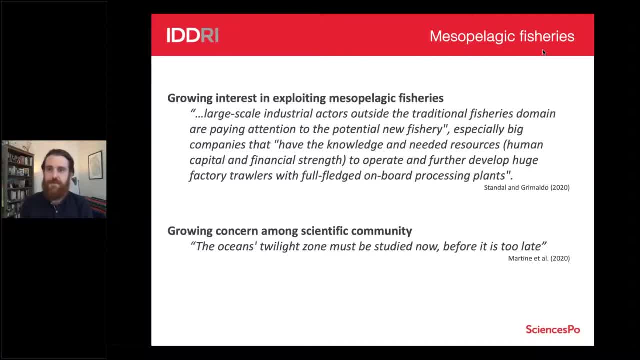 also that the fish aren't very palatable. there hasn't been a development of large-scale commercial fisheries to date, But there is now growing interest in exploiting these fisheries, and particularly for use in what we call nutraceuticals like omega-3 oils. 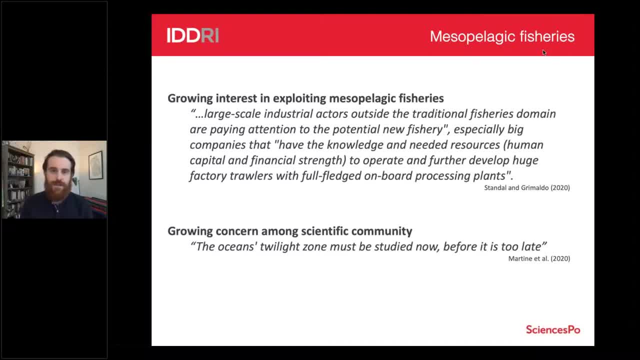 and possibly also to use in fish feed for aquaculture. And at the moment we see in the literature and sort of amongst the science and kind of policy fields this sort of growing tension between the interest in exploiting the fisheries on the one hand, but a growing concern. 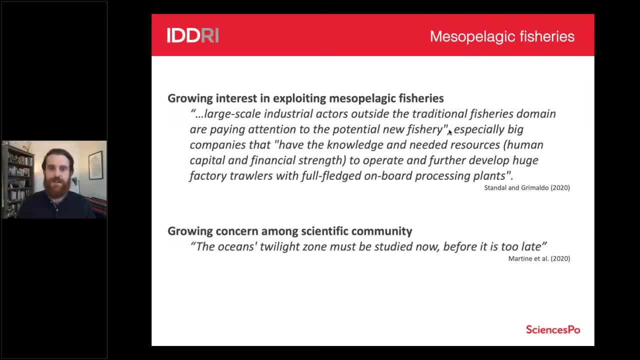 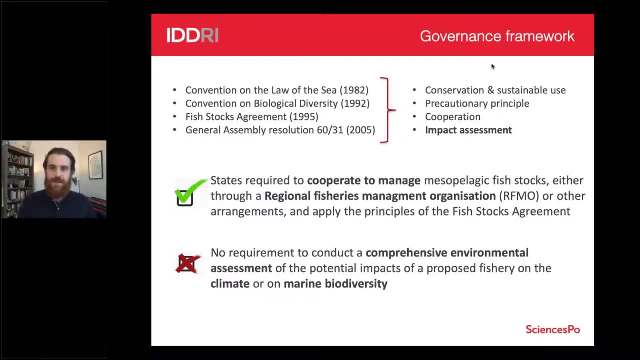 amongst the scientific community. that stresses the lack of science and technology. And so, in terms of the governance framework- and this is where the impact assessment becomes relevant- I can't go into a huge amount of detail here, but on the left, here you see- there's a range of 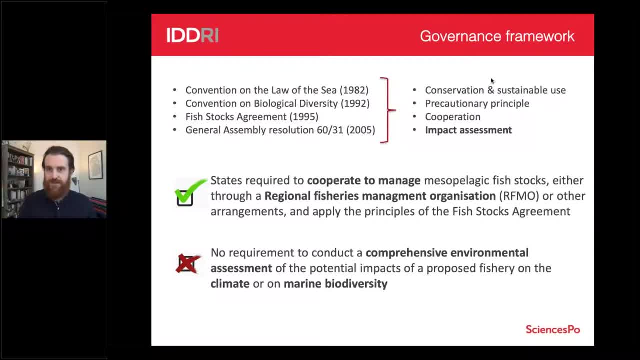 existing international instruments that apply to fisheries in various guises and in some sense apply or are likely to apply, according to our sort of analysis of the framework, to mesopelagic fisheries, At the very least the Law of the Sea Convention and Fisheries Act, which is the law of 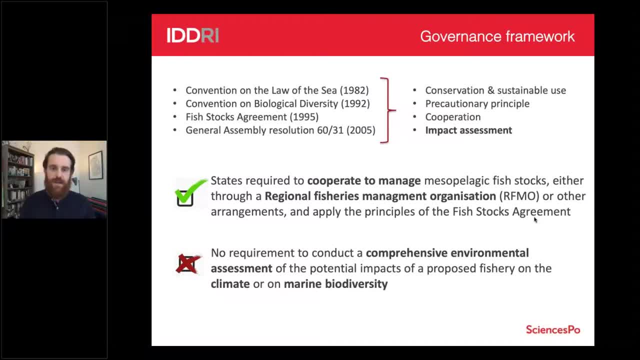 the sea is a very important part of the framework, And also the law of the sea, the law of fish stocks and fisheries. if you know the land and county in question, I think that's a very important part of the framework, So the name of the section in there and for everybody who's interested in going out to the 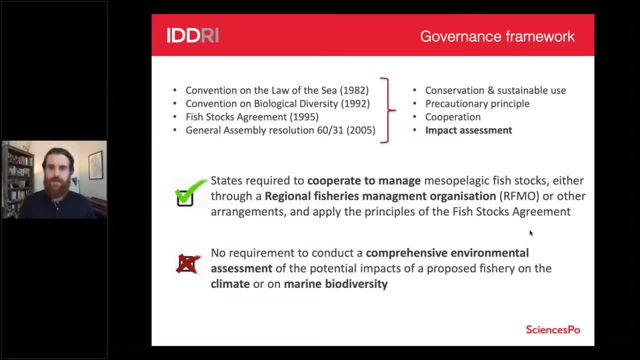 market for any kind of concern regarding fish stocks and fisheries for all kinds of reasons is a little bit different. But yes, this is the law. there's multiple terms on it. we'll discuss that in a little bit. is the law, So this sounds very good. 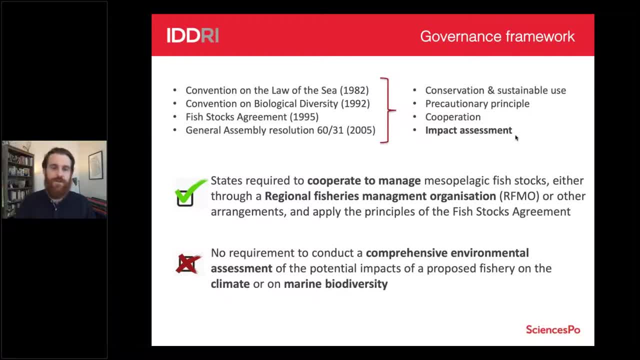 but I think there's a lot of questions in there that I think also pop up quite a bit. I'm going to go back to the end here. there is no requirements under any of these instruments to conduct some comprehensive environmental assessment, so that would include the impacts of the. 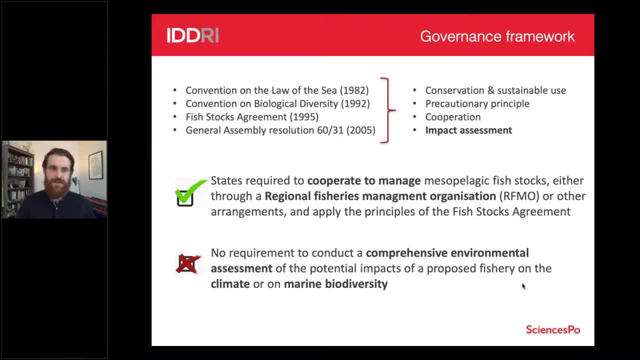 fishery on climate or on other aspects of the ecosystem. so for lands and fish, this type of mesopolitic fish that may be used for eventually, for human consumption, for example, we wouldn't necessarily need an impact assessment on what that would cause for the predators that feed on them. one minute: 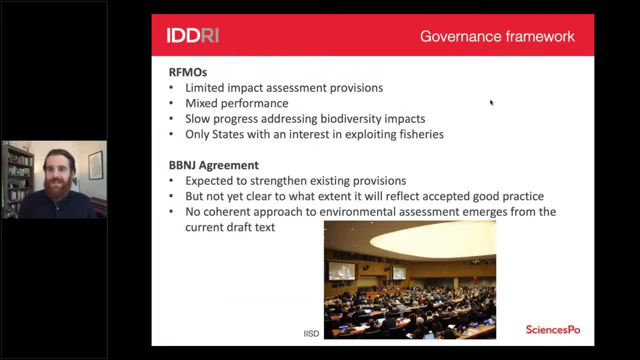 thanks. and in terms of the institutional framework, I mean, RFMOs have had a very mixed performance and often been very slow to address biodiversity impacts, and they don't tend to include states that have an interest in biodiversity. so in this regard, the BBNJ agreement could strengthen the. 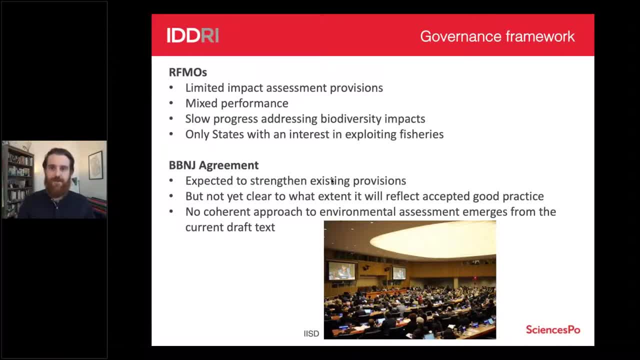 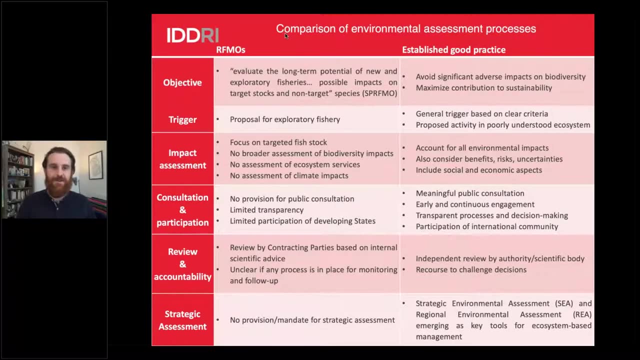 existing provisions, but it's not yet clear to what extent this will have sort of a new global process versus leaving it to the existing sectoral bodies like RFMOs. I won't go, obviously, in the 30 seconds that are left into this, but I will leave this in the slides. it's just a comparison of some of the 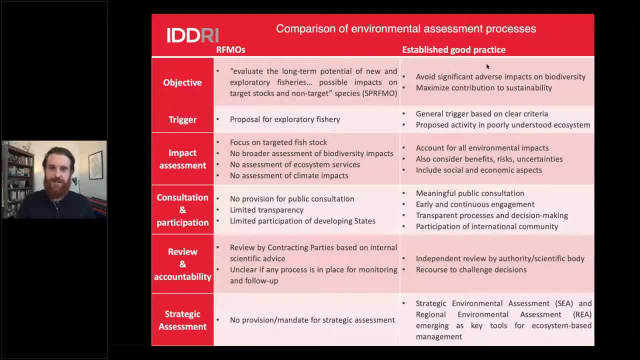 established good practice in impact assessment that Mynhardt has already mentioned, and so, for example, having triggers based on clear criteria and, particularly for poorly understood ecosystems or vulnerable ecosystems, having more sensitive triggers and comparing this to the current practice under fisheries management standards organizations, which are very much focused, understandably, on the potential for fisheries. 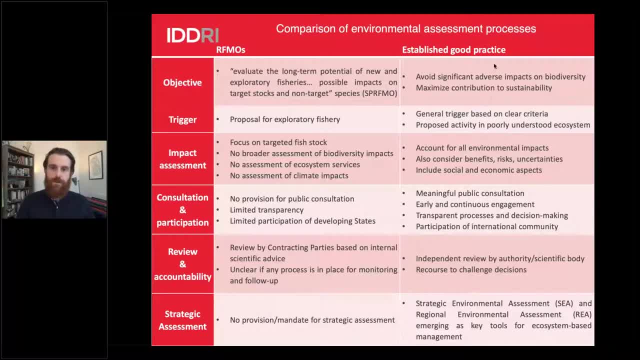 on the impact on stocks, um, but if i could take one thing from from this table, um, the most important i would say is the lack of mechanism for consultation of non-fishing states within rfmos. and so, currently, if you want to have an impact assessment for a proposed mesopelagic fishery, 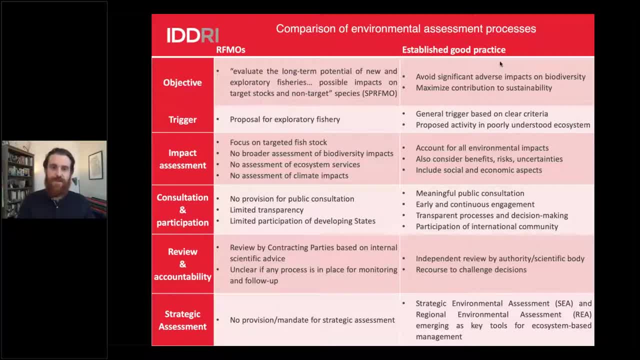 it would be limited to an rfmo process which is quite focused on sector-specific provisions in terms of integrating climate. of course, a single sector impact assessment will not account for cumulative impacts, won't account for climate impacts, and so it seems clear that a new international agreement has to set some sort of standard that would either raise the bar for 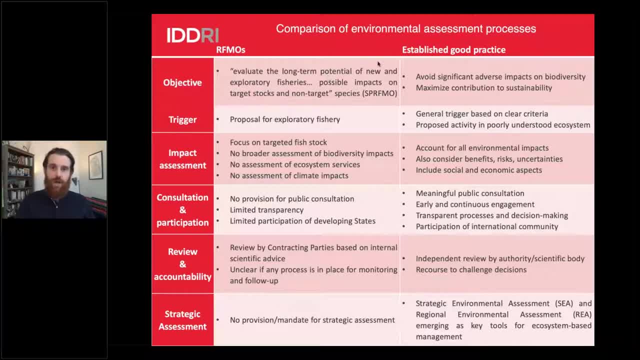 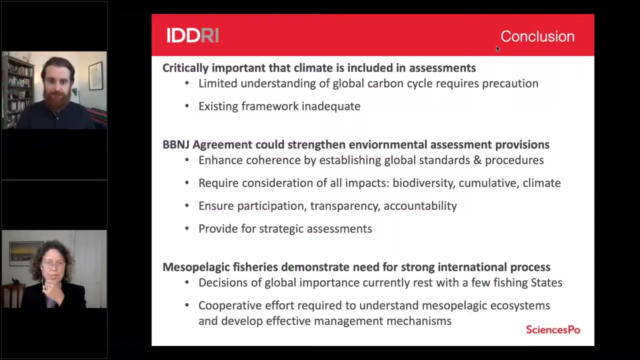 impact assessment done under the current framework or um, likely better would be to provide a more global process where different states and stakeholders can be involved, where climate impacts can be discussed and, hopefully, where strategic assessments of the kind meinhard mentioned could also take place. and so, just in concluding, um, i would say it's 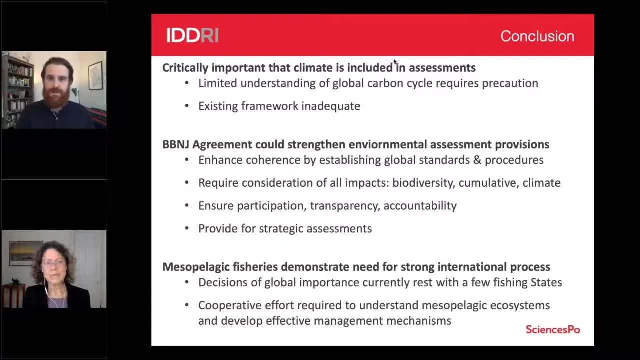 oops, i've lost mine. it's critically important, obviously, that climate is um included in impact assessments. the current framework, which is focused on fisheries, wouldn't be um suitable or effective for such a proposal. um, the agreement could strengthen this with global standards and sort of ensuring participation. um and i think mesopelagic fisheries provide a sort of a case. 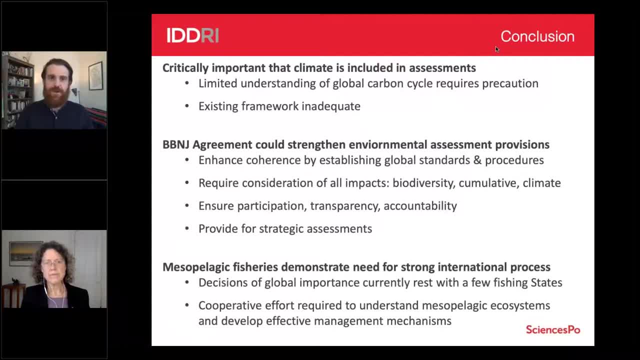 study of a clear example of a new activity where the current framework would not adequately address climate impacts or biodiversity impact. so we really need a cooperative effort required to understand these ecosystems, to understand their climate links and to develop effective management mechanisms, and so hopefully that'll be the case. 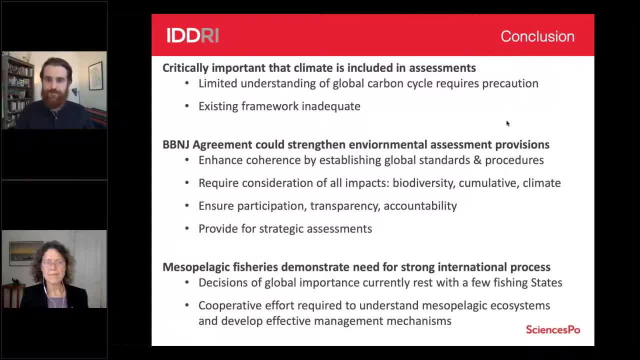 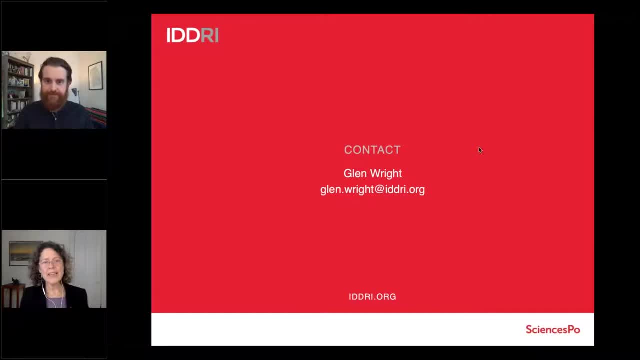 that's something that a bbnj agreement could could bring, so i'll stop there, thank you. thank you, glenn, that i think your presentation really illustrates how this can work and why it's important. um so, thank you very much, and i'd like to now invite all the speakers to join. 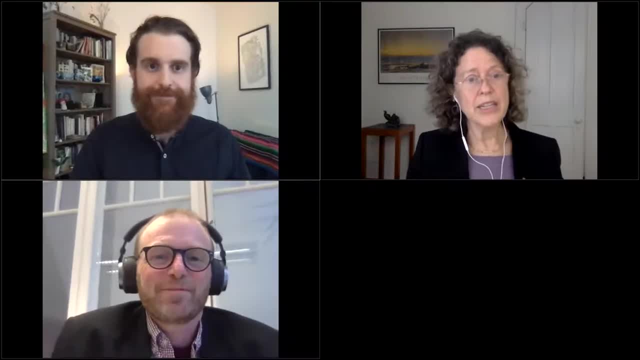 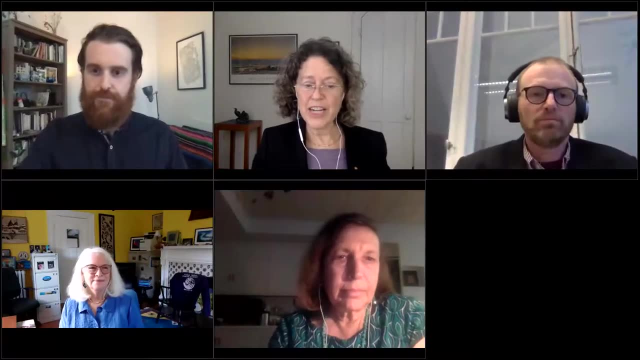 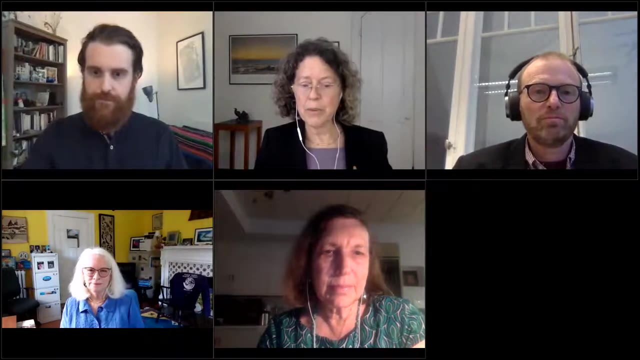 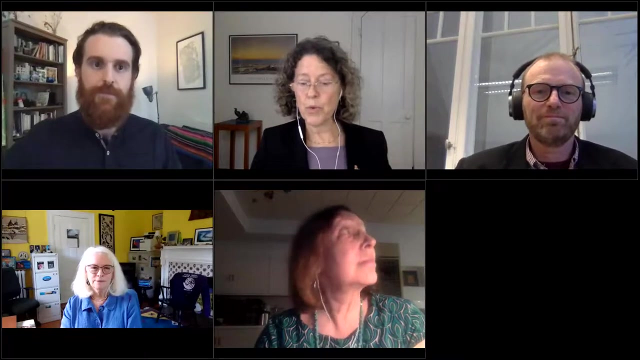 us for the discussion by turning on their cameras, and we're also joined by professor christina gerda, who is high seas, senior high seas advisor for the international union for conservation of nature global marine and polar program and adjunct professor at middlebury institute of international studies at monterey, california. in addition, she's a member of the world commission on environmental. 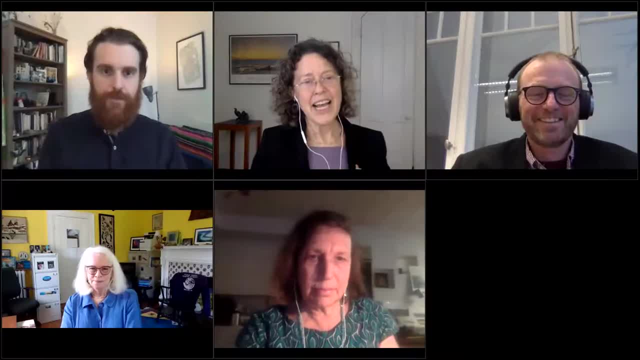 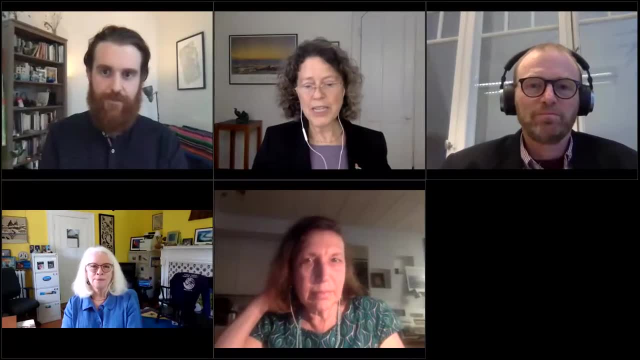 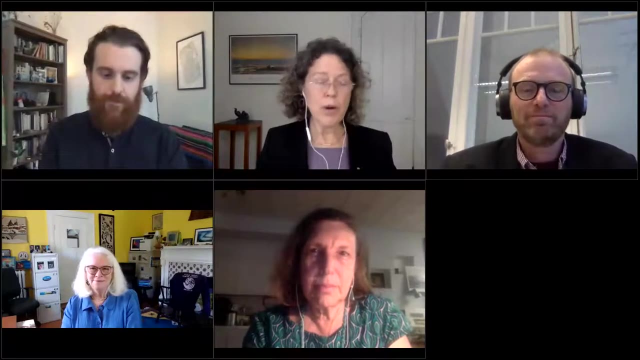 law array, the world commission on protected areas and, with lisa levin, serves as co-lead of the deep ocean stewardship initiative, dosi, and is a long-time participant in these negotiations on behalf of iucn, and we thank her for that work. so, opening the question and answer. we have a number of questions from the audience and we'll 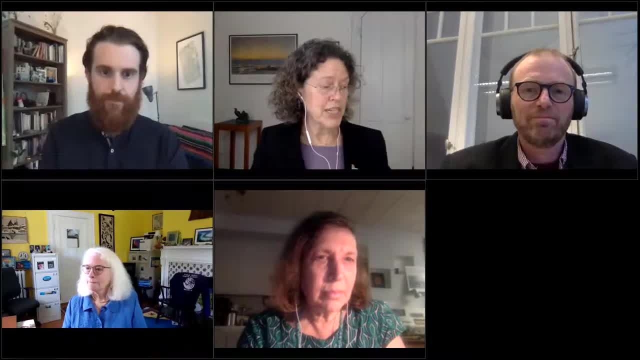 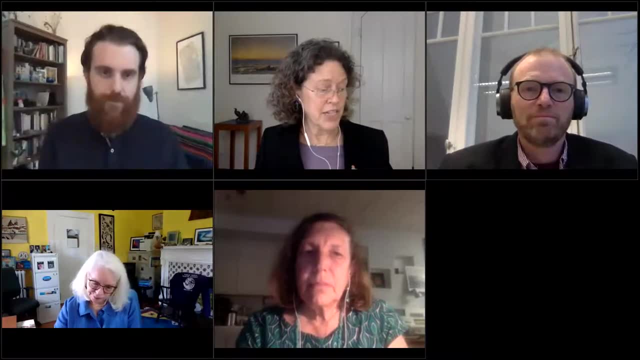 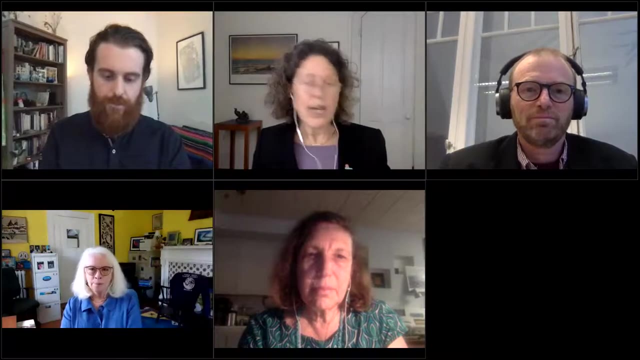 begin with, roderick hart from the european commission asks. professor doell stated that certain climate impacts are difficult to resolve at the project level alone, suggesting that strategic assessments would be better suited to address such issues as climate change impacts. uh, meinhardt, could you elaborate on that, and perhaps with a concrete 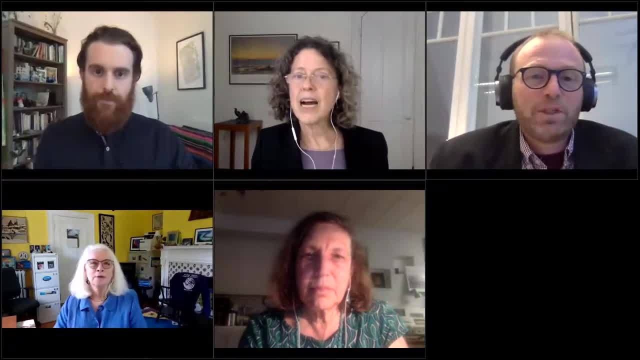 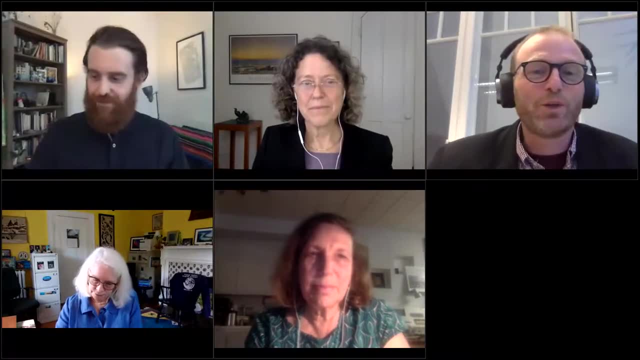 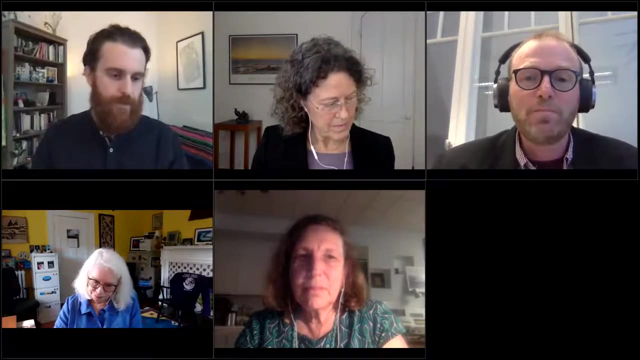 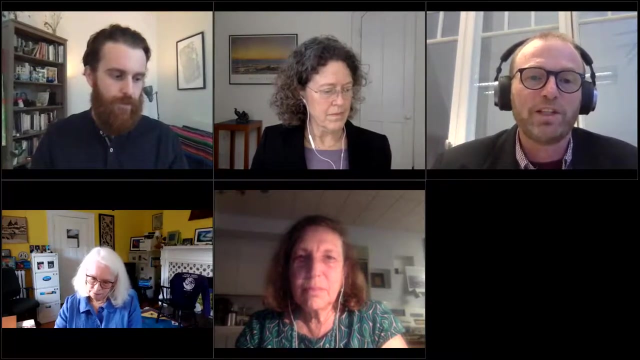 example, you're muted. oh sorry, um so sure, happy to. i think the example glenn gave is actually a perfect example of this. for us to understand the impact of climate, of projects on climate change, we have to understand the impact on the mesopelagic, because it is such a significant uh sink and carbon sink and reservoir. 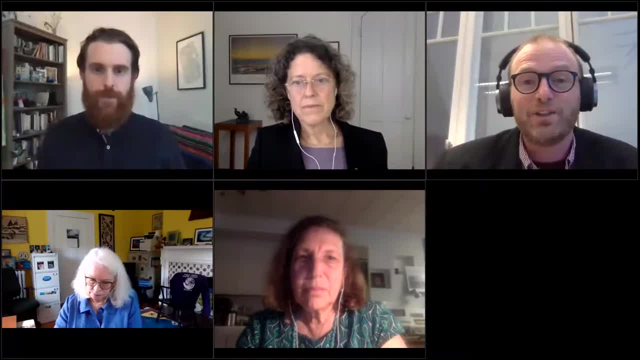 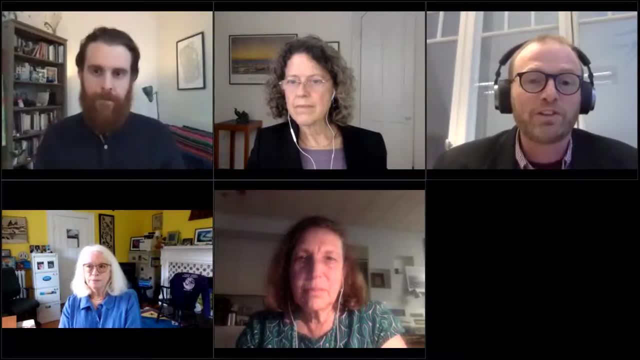 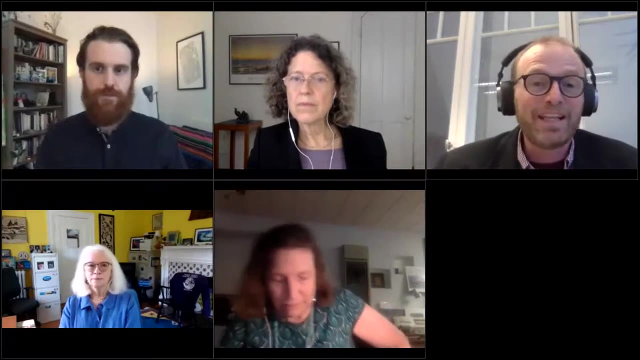 um so, um so. that means that you have to understand all these dynamics. so if you're, for example, if there's a proposal to start to fish the mesopelagic zone, um, you have to consider, uh uh, the impact of of that, and that's very difficult to do in the context of one particular project. but if you did a 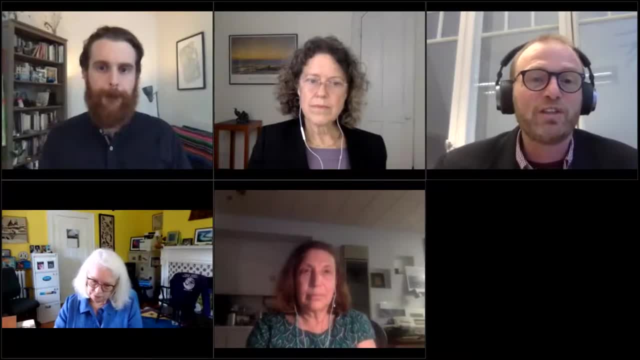 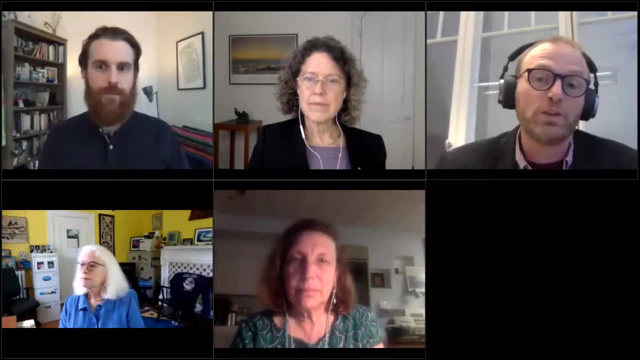 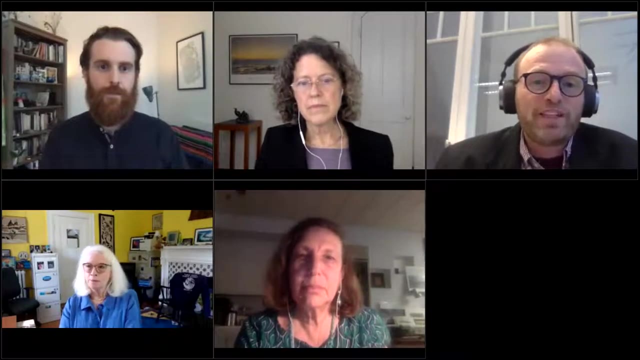 strategic environmental assessment of fishing the mesopelagic, then you, i think you would have a much better chance of create, of raising some of these issues. and let me just give you one other example, and that is that whenever you're faced with a region where all kinds of different things could, 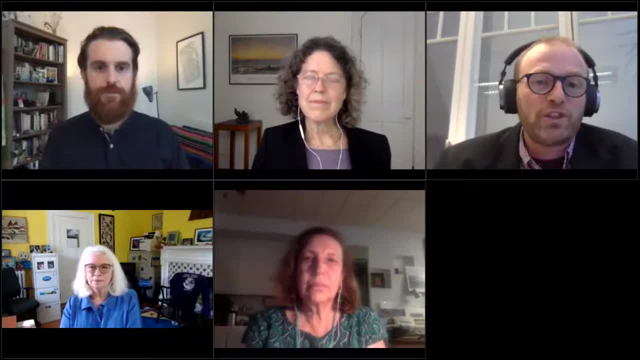 happen. it's very difficult to address all those different scenarios at the project level. so you can have different levels of activity, different kinds of activities and you can't just say, oh, i'm going to do this and that, but you can have different levels of activity. but you can also have 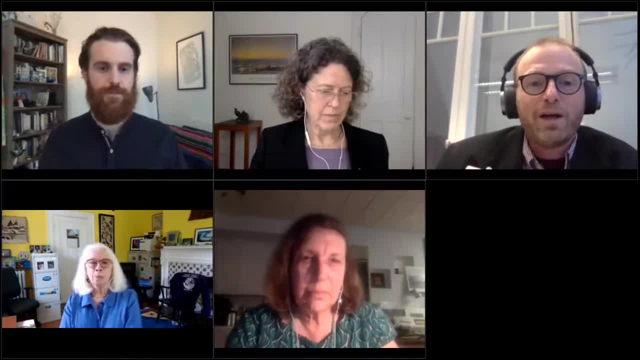 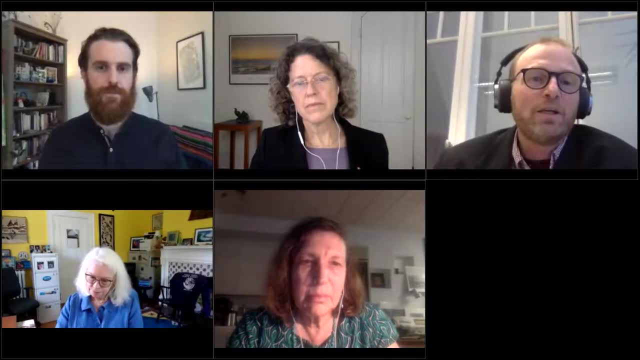 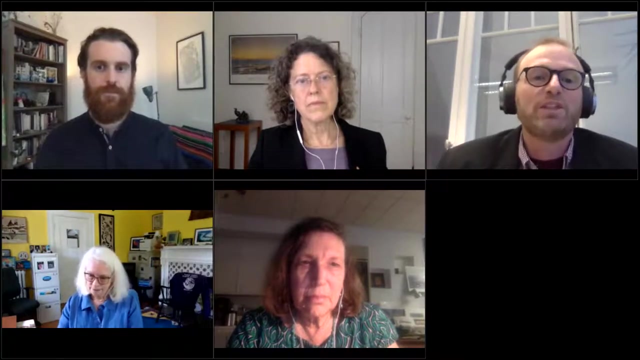 we also have to create different scenarios for uh, what the mitigation efforts will be like globally and what impact that has on climate impacts in a particular region, because those climate impacts will interact with project impacts to then have impacts on ecosystems. so those are things that are very difficult to do at the project level. but if you set up regional assessments and strategic 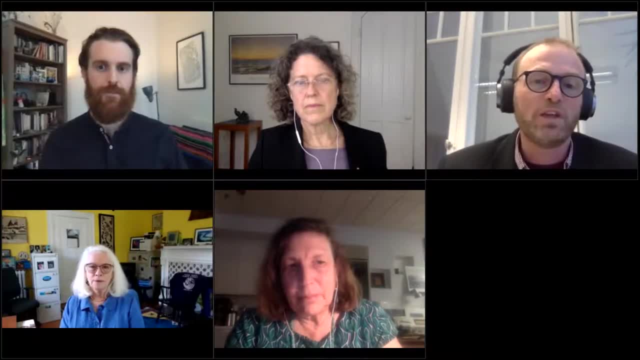 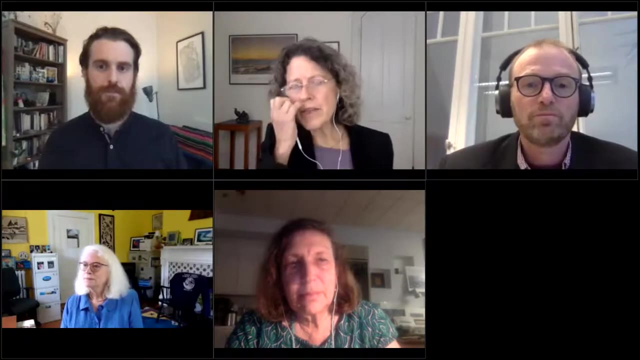 assessment, assessments prior to project level assessments, you can make significant project process, project progress and you can set the context for doing effective and efficient project level assessments. thank you, yeah, i think you. you know what we start to see is that this kind of collaboration can also make the projects better and maybe open some. 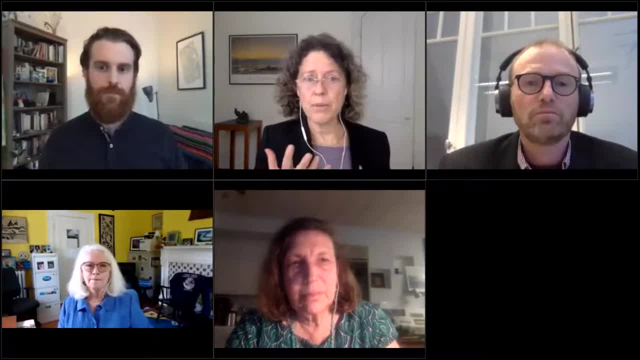 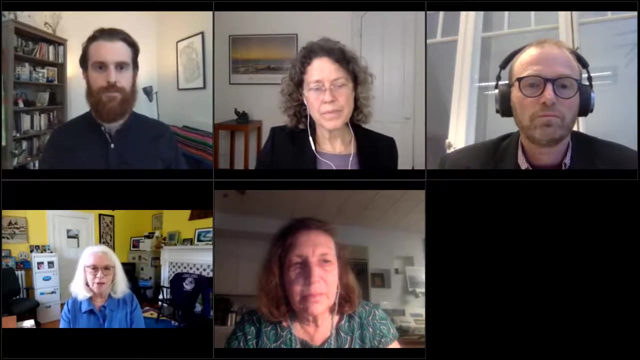 options that hadn't been thought of originally by the project proponents, and that doing this in a larger collaboration through an sea state research center or a commercial space is a longer-term kind of planning option. yeah, christina, please hi, just in terms of examples. another good example is, of course, deep seafood mining. that's where contractors have been expected. 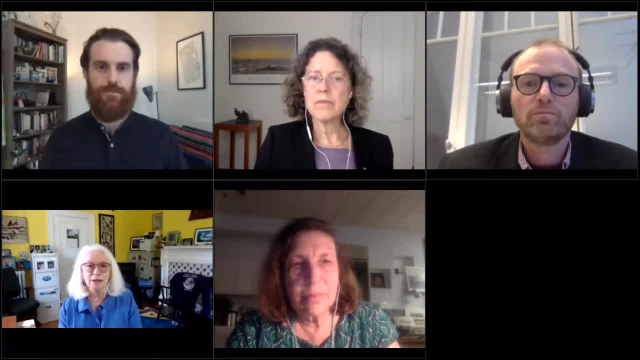 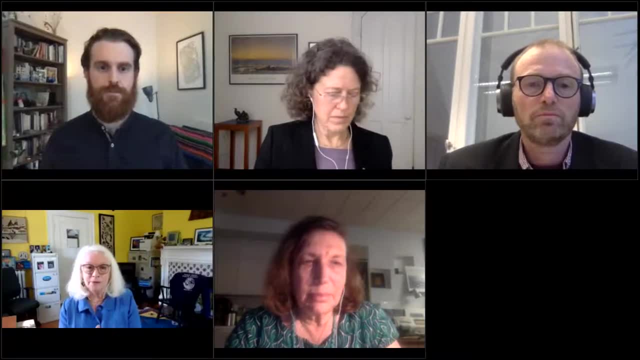 to conduct these 15 years of exploration. but only recently have we really discovered the importance of the mesopelagic in these climate change and food provision services for all of our commercially important fish species. So it's really important to go back and sort of try to think through. 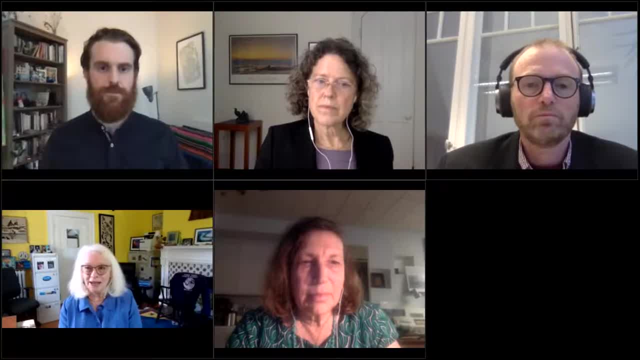 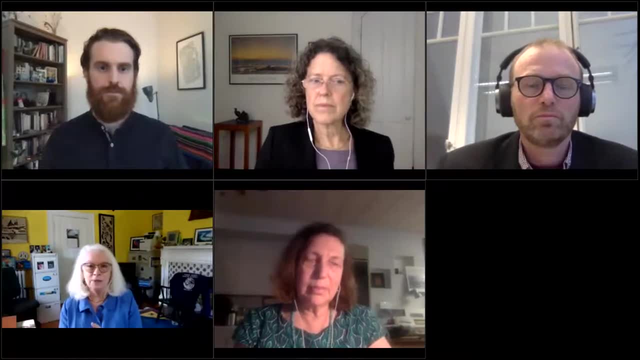 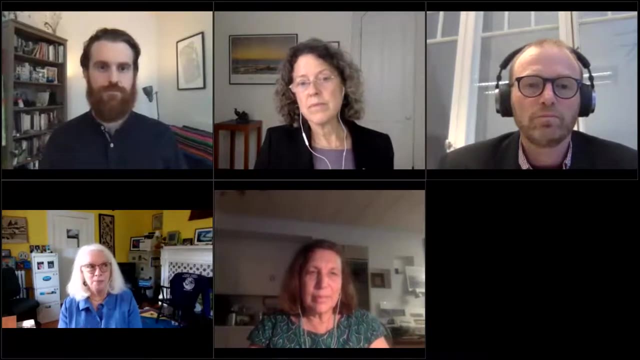 who needs to be involved in these discussions? how can we better engage these different sectors, as well as the biodiversity interests, and look at what the potential impact of deep seabed mining could be on CO2 sequestration? And, of course, as Lisa Levin was stressing, what are the added? 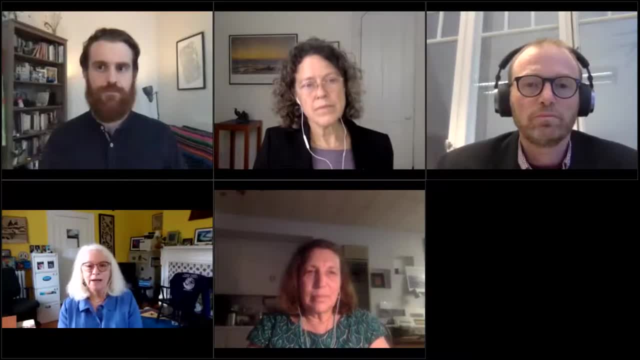 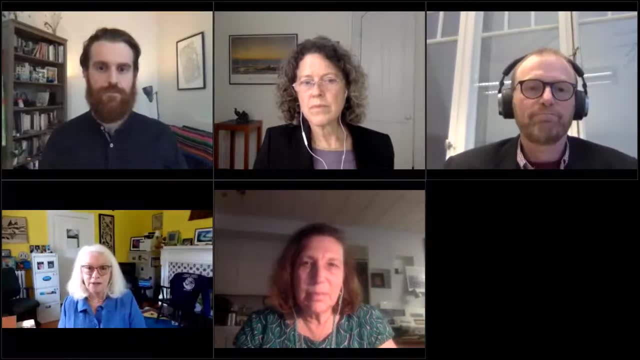 impacts of a new activity like deep seabed mining on an already climate-stressed ocean. It may be different in different parts of the ocean, but we need a far better understanding of how these things interact. Thanks, Are there comments on that or other reflections that you'd like to add? 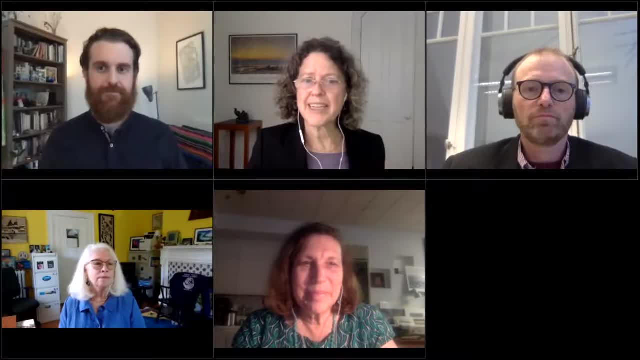 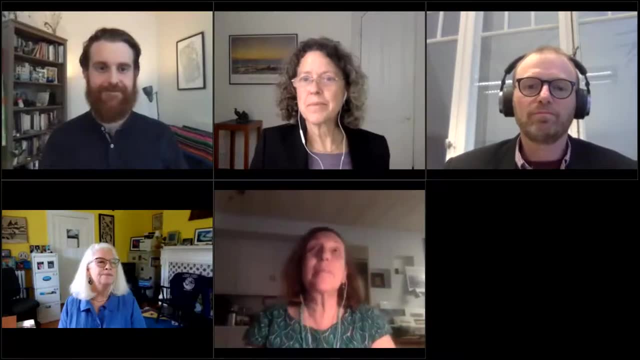 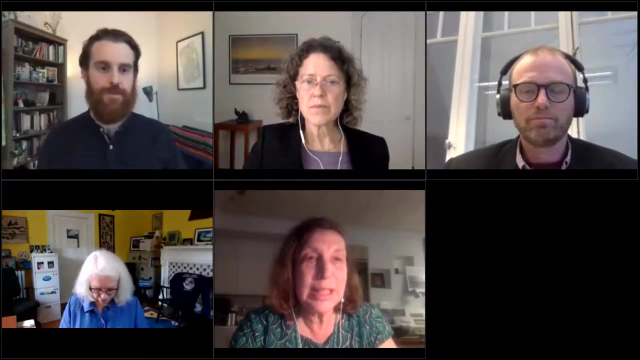 on the strategic and environmental assessment, Lisa, I mean, let me just say that the modeling tools that I talked about are particularly useful in that regard for doing regional assessments. I think it's important for us to look, because there's so much heterogeneity in how climate 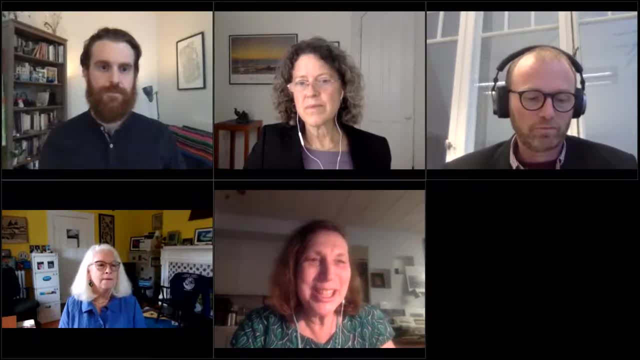 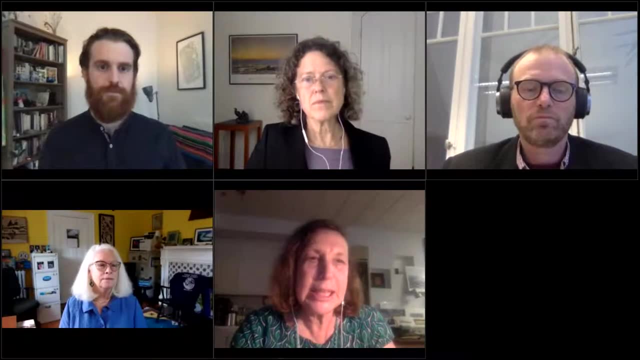 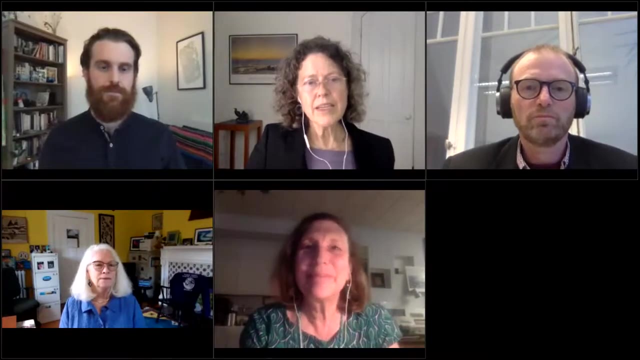 change manifests itself. It's not uniform across the ocean, and so, even within a single region, you can see areas that will be more and less vulnerable, And so applying these tools can be very helpful in achieving what everybody else has been talking about. You know, I had a question. 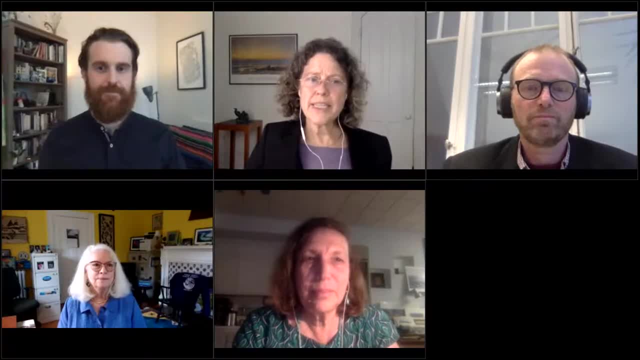 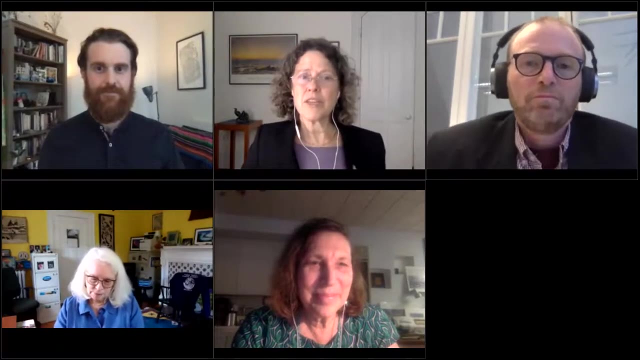 I'll take moderator's prerogative to ask it, which is: do you see the scientists as being maybe not in an ivory tower but off on a research vessel and maybe somewhat inaccessible? So if I'm a policymaker, back in capital looking at this and 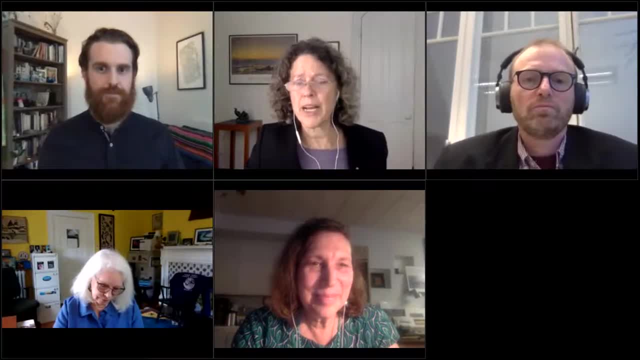 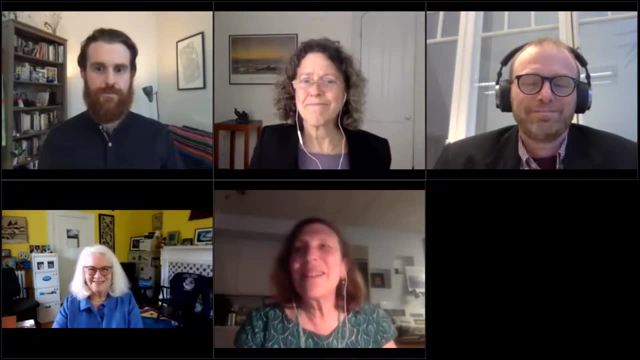 thinking: well, this is all great, but I don't have scientists on tap who I can call on. can you offer some thoughts on what can I do? Well, this is exactly why the Deep Ocean Stewardship Initiative was created. really, 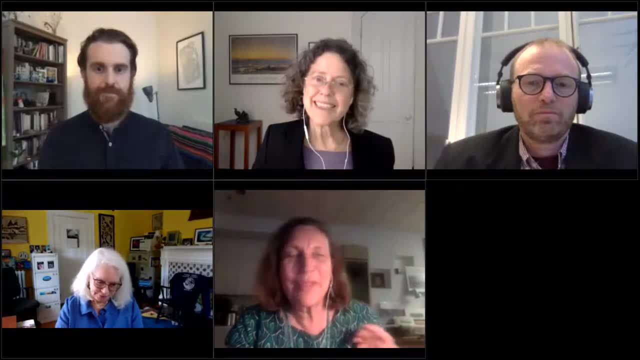 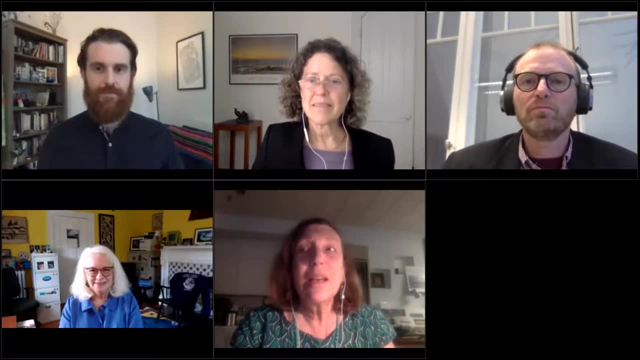 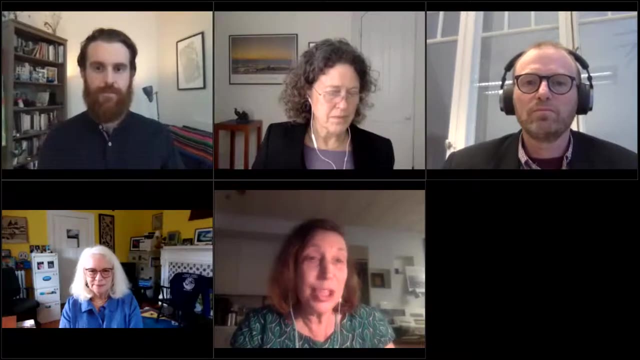 This is a group of. I just learned yesterday there's more than 1,500 people involved now from 70-some countries- 78 countries, something like that, and 11 working groups, And one of the working groups focuses exclusively on the BBNJ Treaty, but there are groups a climate working. 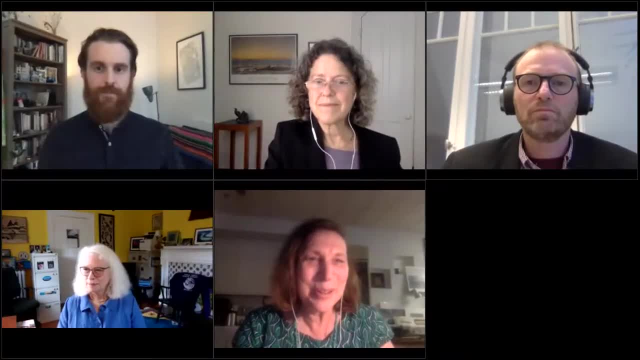 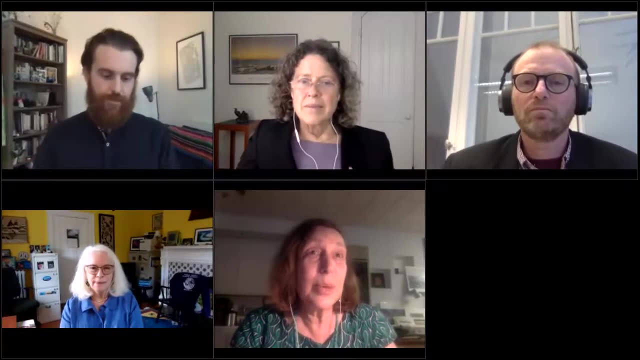 group, and a fisheries working group, and a marine genetic resources working group, and a pollution and debris working group, and so on. And so these are all working groups, And so I think it's important for us to look at the data, And these are all scientists who've indicated a willingness to engage in policy. 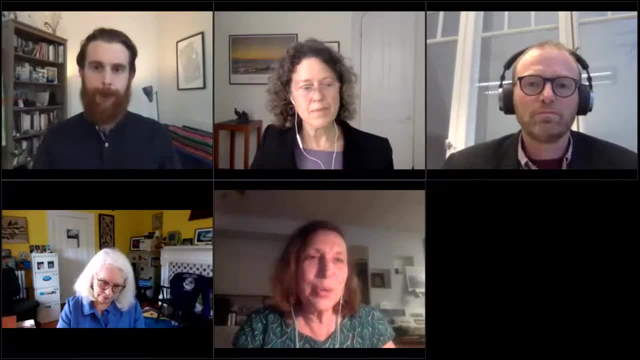 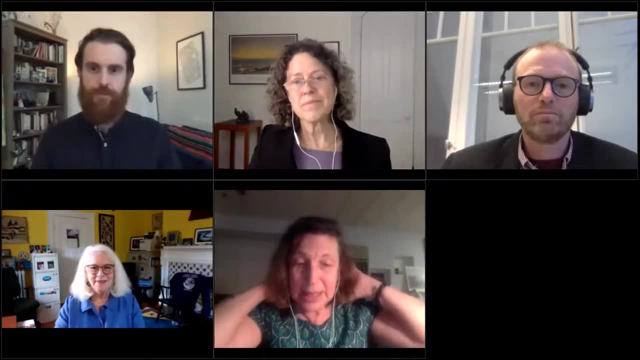 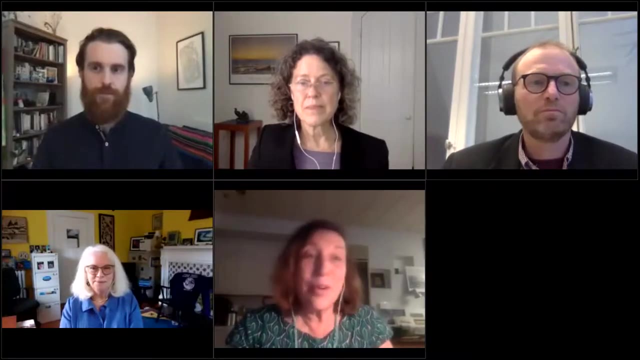 and many of them do now try to work with policy people like those of you on this webinar, And I think you know. all I would say is, if you are in need of access to scientists, contact me or Maria Baker at doci-projectorg. 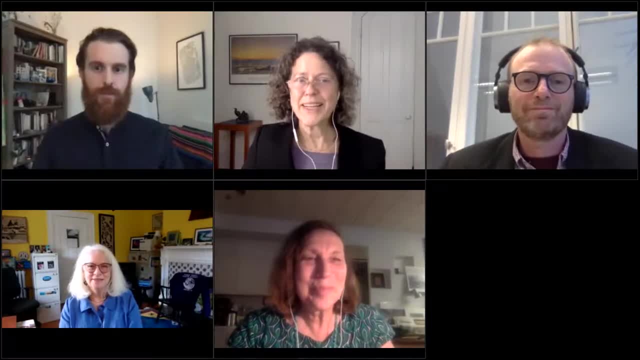 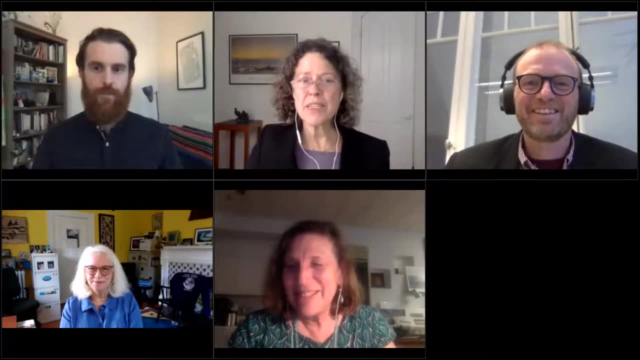 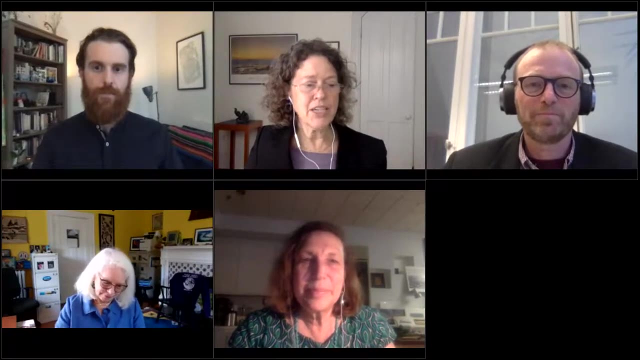 Or our emails. Yeah, Great, Thank you. So there are scientists on TAP. Excellent. So we have another question. This is for everybody: How should the BBNJ instrument treat with other processes under existing relevant EIA frameworks to prevent a fragmented approach? 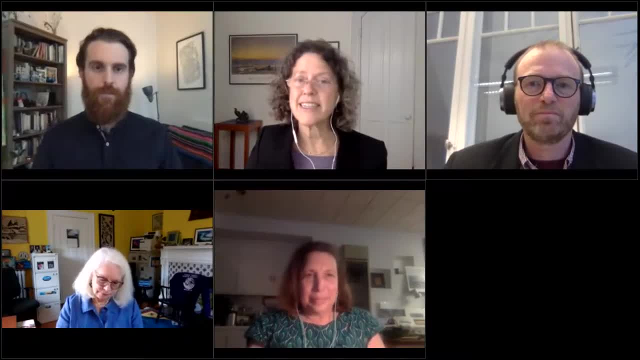 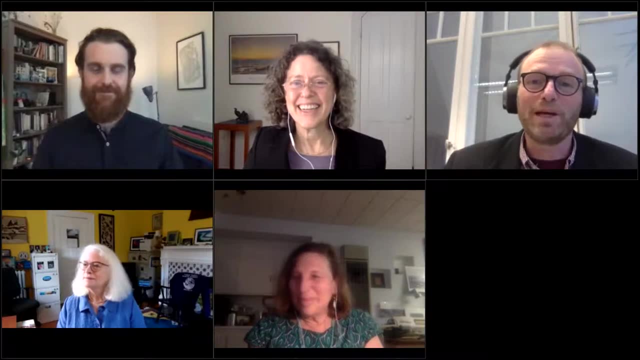 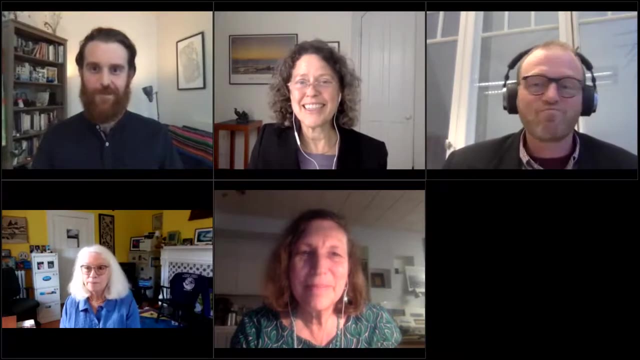 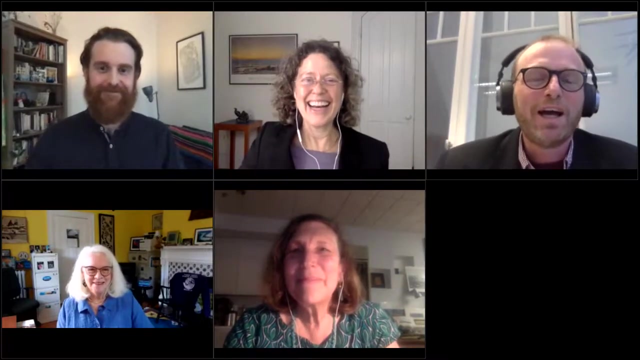 to incorporating climate change considerations. We'd like to tackle that first. Maynard, You're unmuted, You're on mute. Oh, you can't unmute, Oh no, Oh okay. Sorry, I lost control over my mute So I lost my train of thought. now, But, 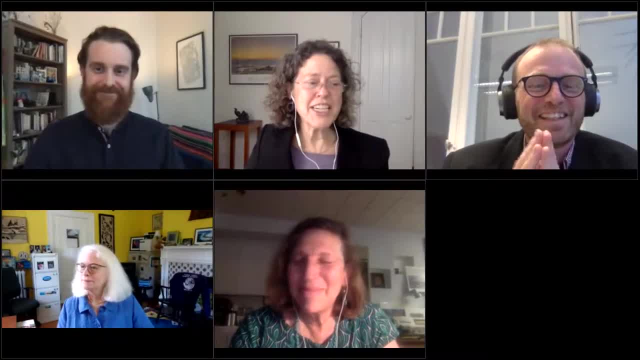 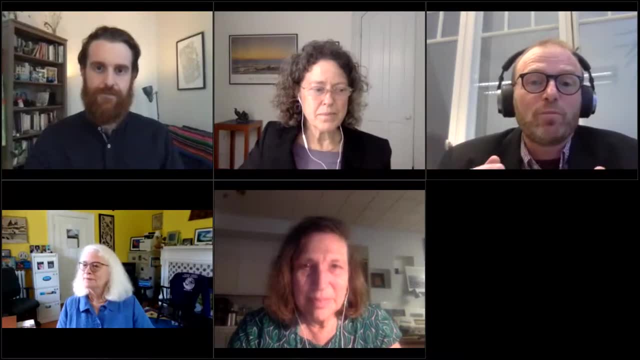 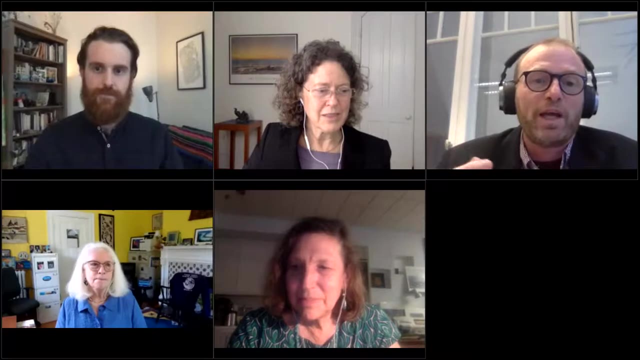 what was the question? So how should the BBNJ instrument interact with other processes? Oh, yes, Yeah, I mean. I think we have learned from environmental impact processes in many jurisdictions that the most efficient, effective and fair way of doing environmental assessments is to have 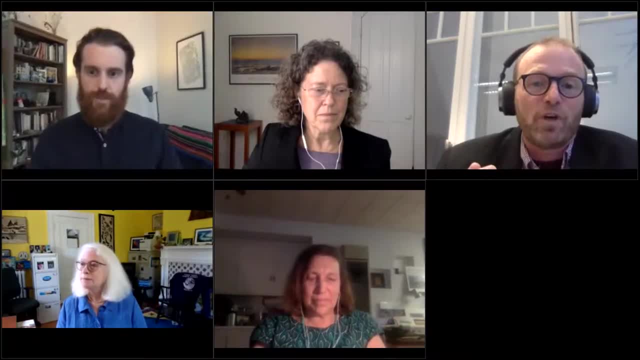 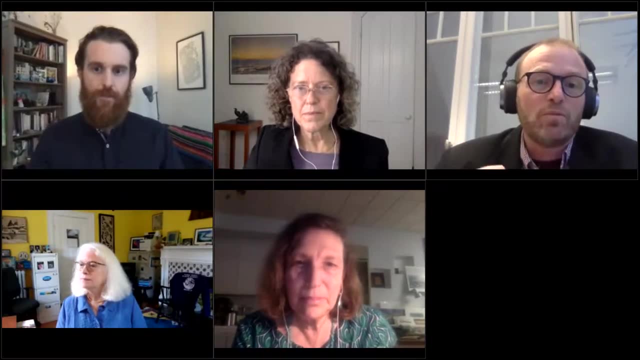 all decision-makers actively involved in one process. So the ideal scenario is that we create a mechanism whereby all decision-makers with respect to a particular proposal or activity come together. So that we can create a mechanism whereby all decision-makers with respect to a particular proposal or activity come together. 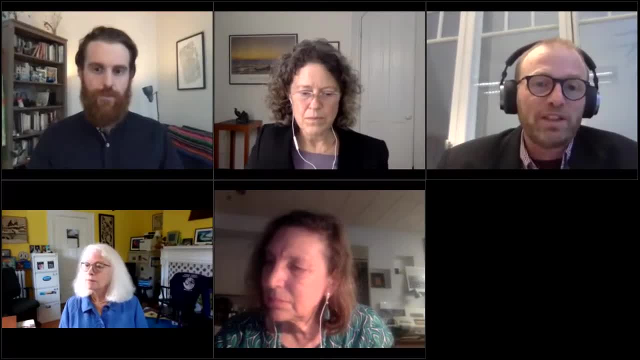 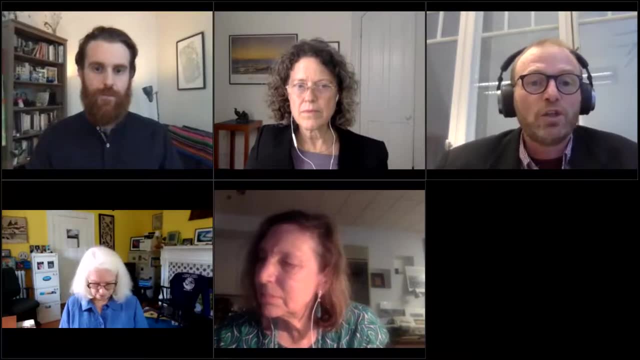 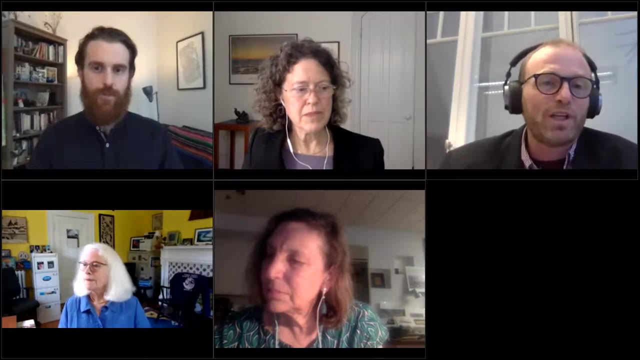 I mean that is. I think one thing we would have done is to have the decision-maker come together to jointly design and implement one process and then the Environmental Impact Assessment Report informs the various decision-makers. So if you have a region where there are decisions to be made by the International Seabed Authority, 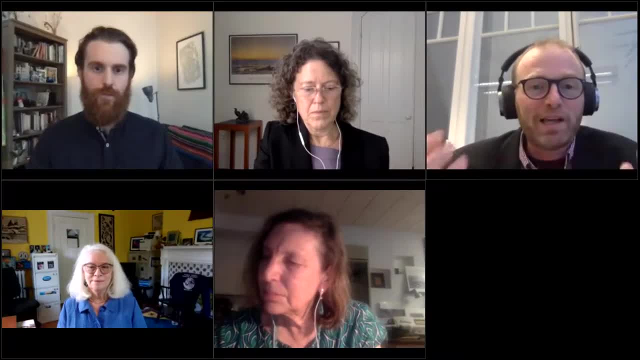 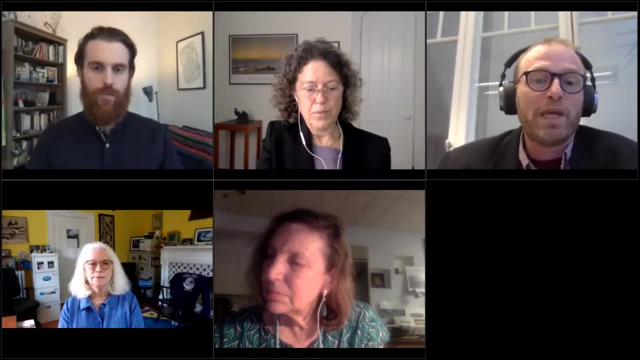 by regional fisheries management organizations, by the IMO and maybe by the decision-makers set up under the new BBNJ regime. it would be important to have the decision-makers involved in the decision-making process too. ENJ regime: all those decision makers would come together and do one assessment. That is the ideal. 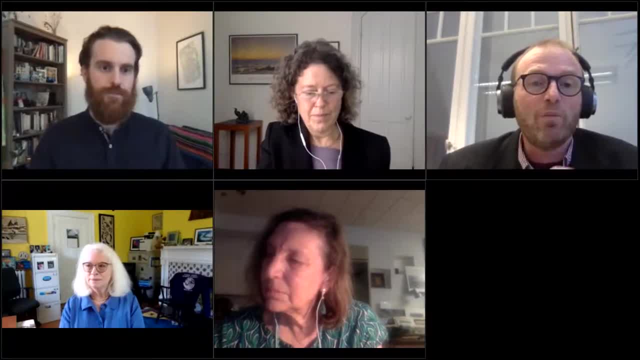 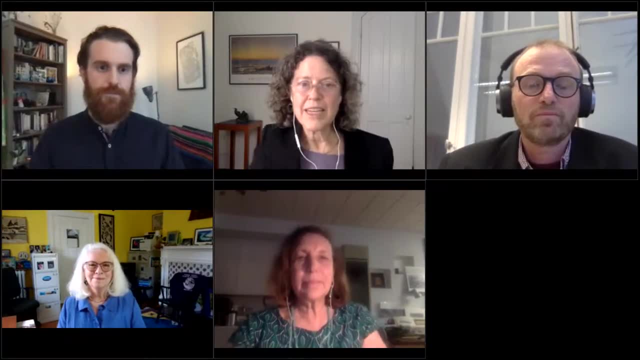 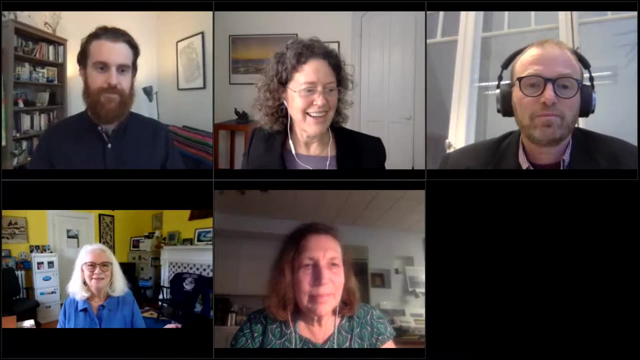 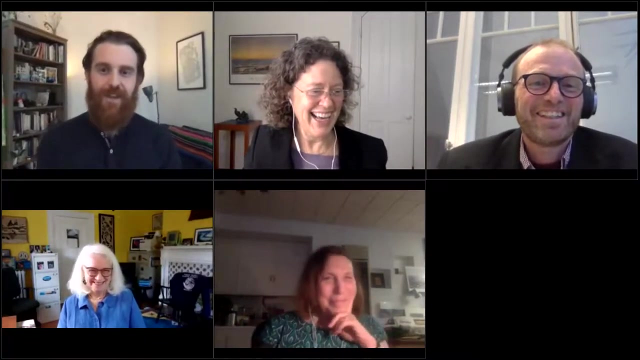 scenario for integrating all the considerations into an environmental impact assessment process. Any other comments anyone like to make on that question? I'll go after Glenn. I was going to say I'll go after Christina. I mean perhaps just to sort of build on that and add something on where the negotiations 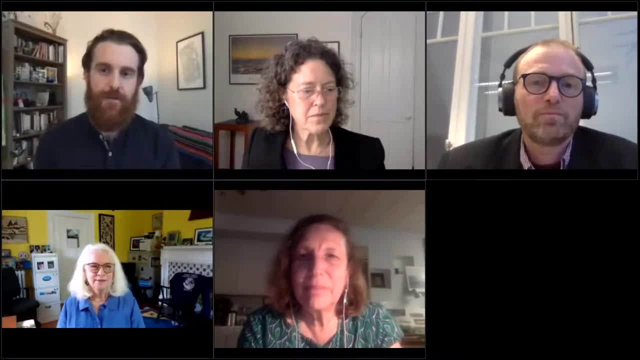 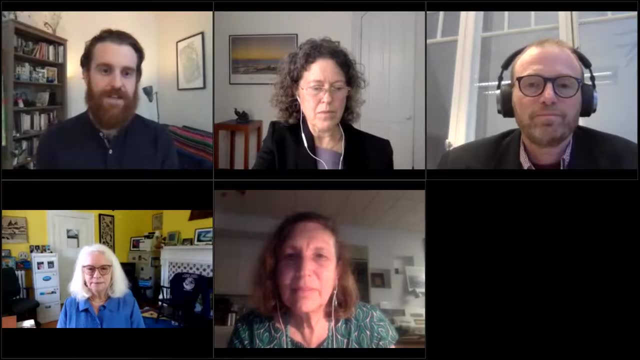 are and what the current framework looks like. I mean, no really sort of coherent approach seems to emerge at the moment from the draft text And there's sort of two branches, almost. One would be more towards a global approach and the other more of a global approach. 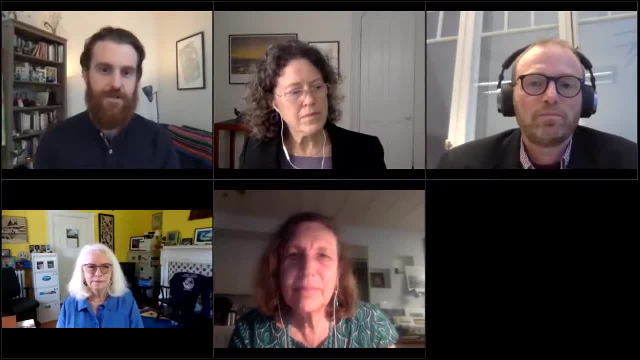 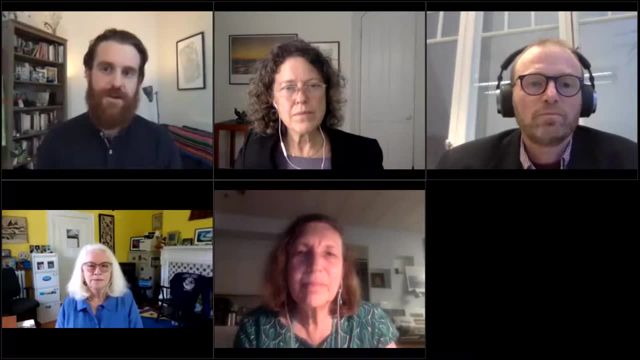 internationalized process which I think would be closer to what you're referring to, Meinhard, where you bring these things together and try and reduce that fragmentation. And another strand is more the not undermining approach, which would be to sort of where impact assessment. 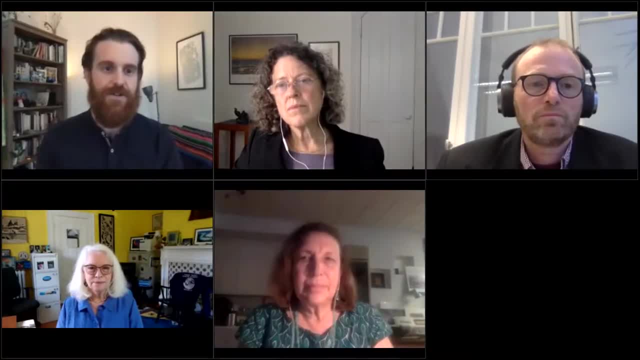 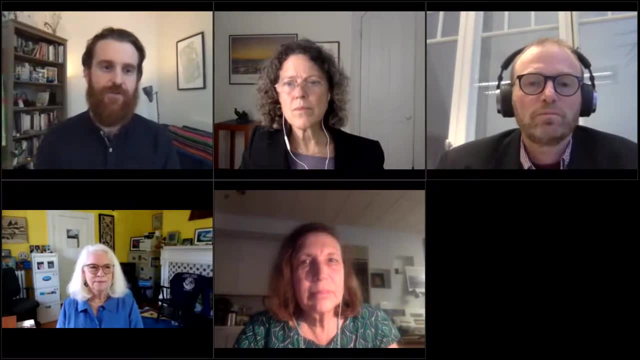 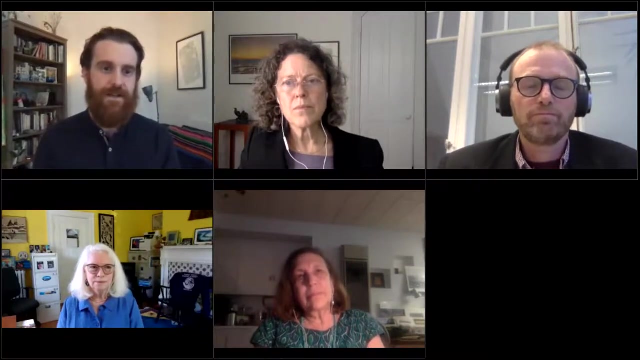 processes already exist for certain sectors or regions under existing instruments. We would leave them alone in some way or only do a brief review of whether those processes are actually effective. To bring that to the mesopelagic fisheries example, there would be a concern there that a regional fisheries management organization could do a very minimalistic. 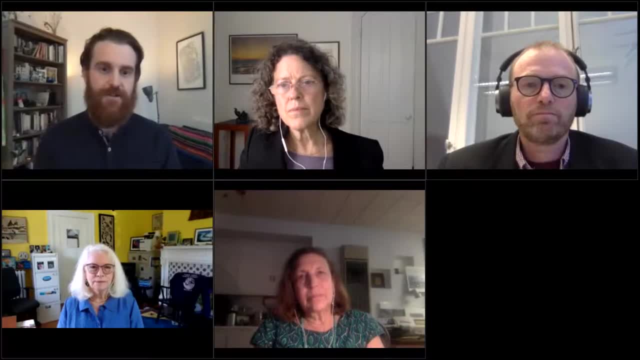 review of an exploratory fishery that wouldn't include all the different stakeholders, climate impacts and all of these other aspects that would effectively be rubber stamped or wouldn't be looked at more closely by the high seas agreement because there's a process in place. 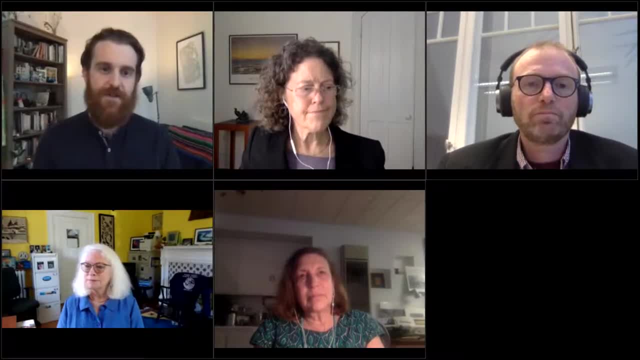 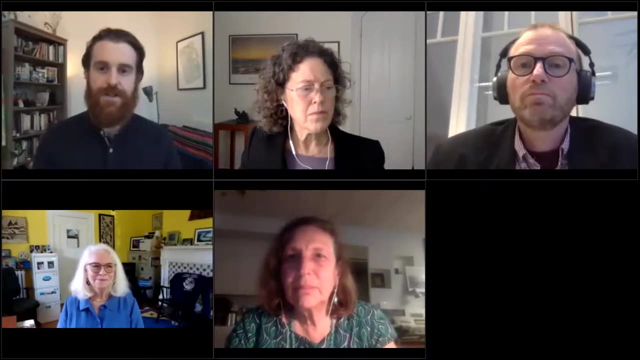 And they don't want to undermine what's already there. So I see two very different routes: that the treaty and that the future of this could go down, And indeed one wouldn't really contribute much to reducing that fragmentation. And maybe just a final thought is just that 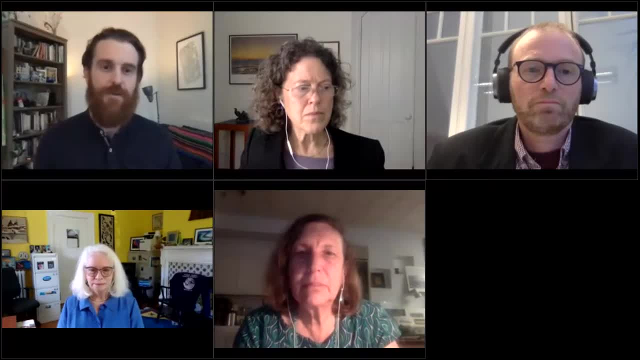 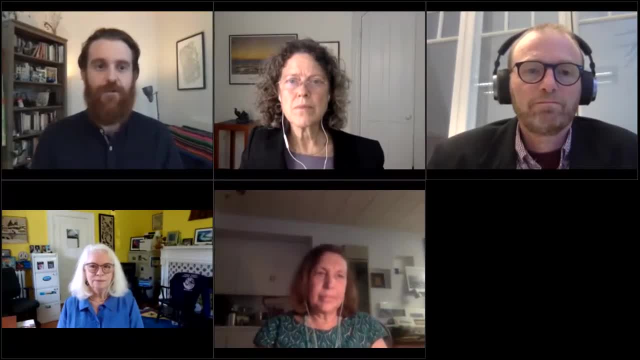 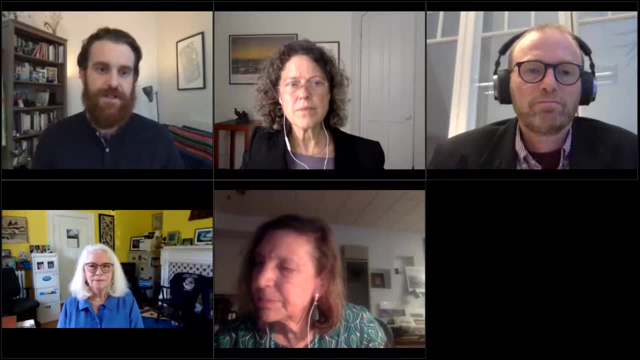 to be done- And I think there's a lot of work that needs to be done- And I think that biodiversity impacts must be integrated. If, then, all of the existing sectoral approaches could incorporate at least those minimum standards, I would go some way to increasing the coherence. 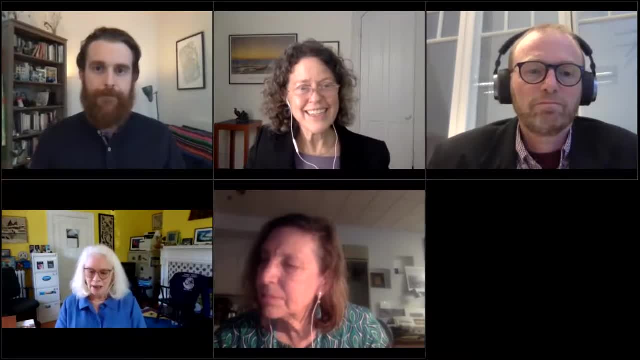 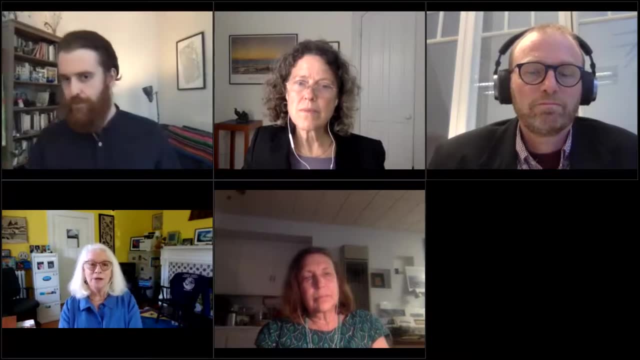 I think I just say the environmental impact assessment provisions are one place where the BB&J agreement can truly help to strengthen existing organizations as well as enhance cooperation and collaboration. I would agree on the need for global minimum standards, and by providing these global minimum standards, 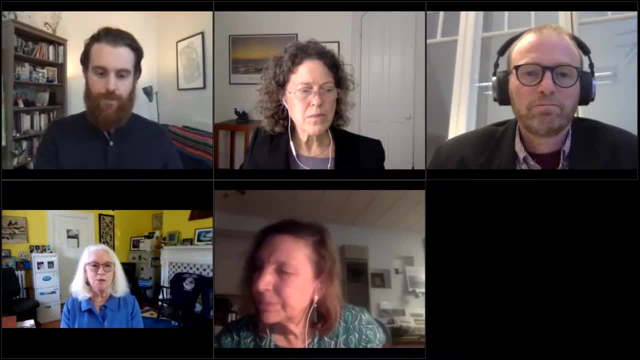 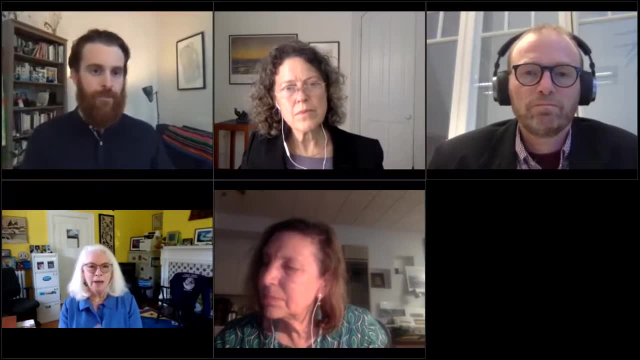 you're actually able to uplift and strengthen the performance of these regional and sectoral organizations by ensuring they have access to the best available information. You can't talk about deep seabed mining if you're not engaging with the fishery scientists. There are many. 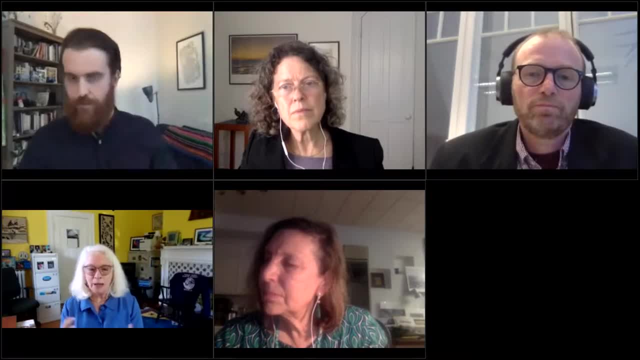 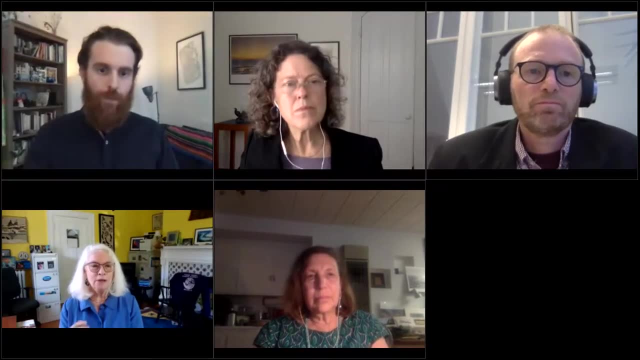 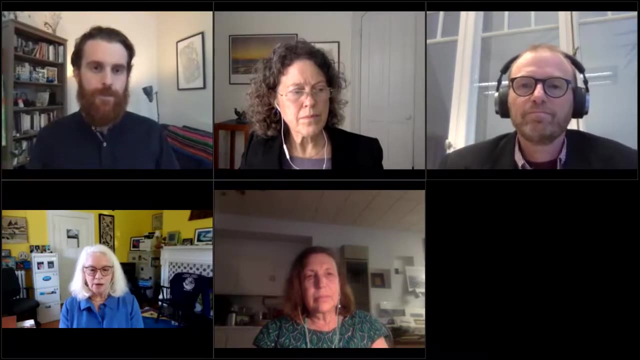 aspects of the changing environment that we need to be able to cooperate and engage at a much higher level and a much more frequent level than they're currently doing. So the approach that would create the BB&J agreement with the EIA provisions as sort of at the gold standard: 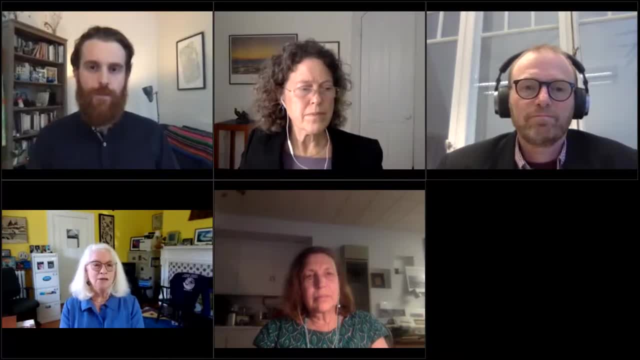 and engage and encourage all players to actually live up to these standards And, as Glenn said, the consultation is absolutely vital at all the stages of the game, including at the scoping, where the critical decisions are really being taken about what questions need to be asked. 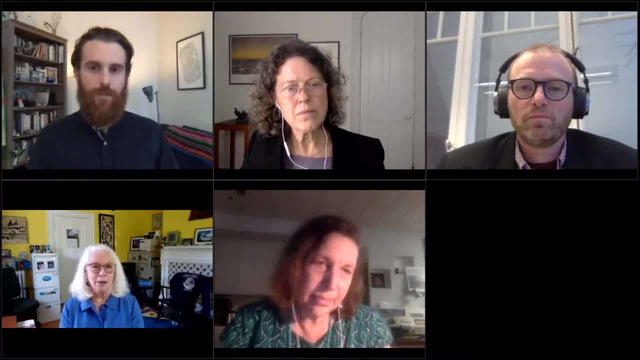 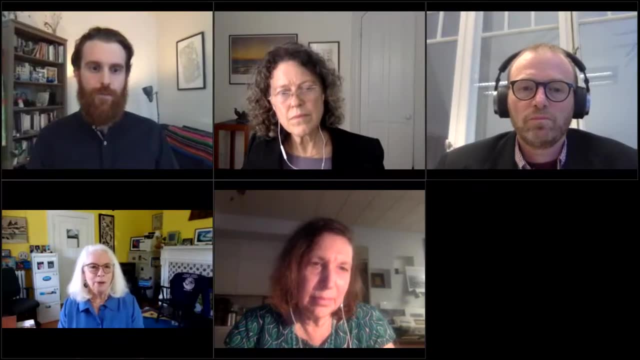 In order to create an effective environmental impact assessment And, just as Meinhardt was saying, you need to be going up the streams of strategic environmental assessment. What's going on in the region and how are these regions interconnected? I would just like to recommend Meinhardt's article. 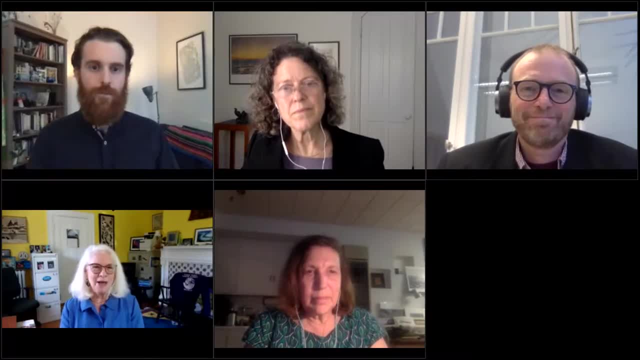 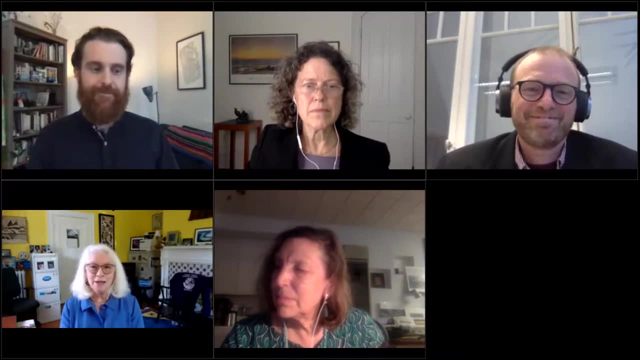 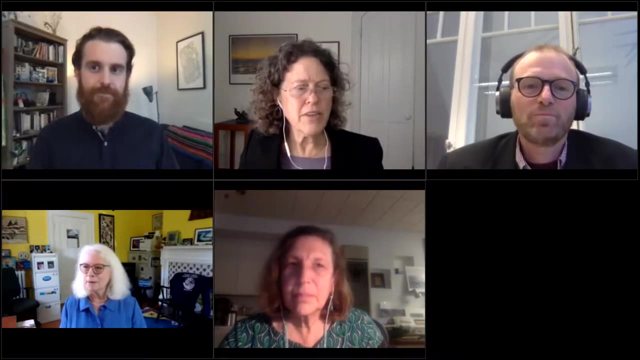 with Gunnar Sanders on next generation environmental impact standards and integrating those into the BB&J agreement. That's been my Bible while working with Glenn on this study, the case study on the mesopelagic Great. We're getting towards the end of our time, So I'm going to put two questions and invite. 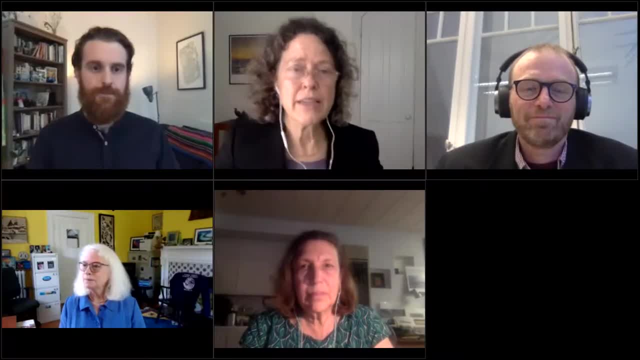 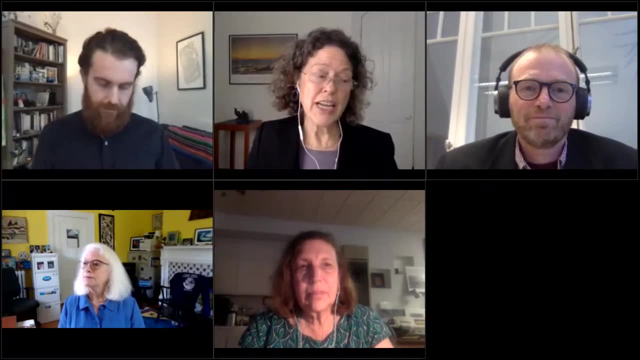 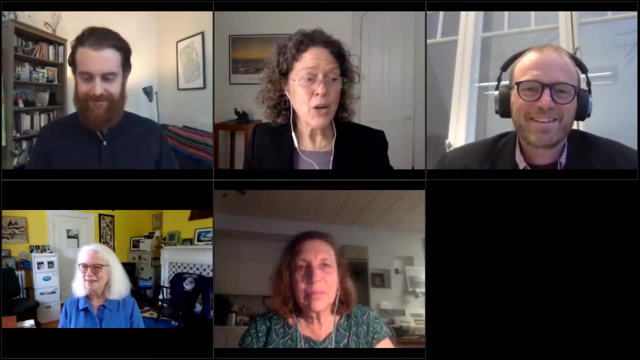 the panel to respond to those and perhaps offer a final comment, if I leave it to you. So the first question. I'm sorry my knowledge of the French environmental code is not what it should be, But from Mel Martin, would it be relevant to get inspiration from chapter one? 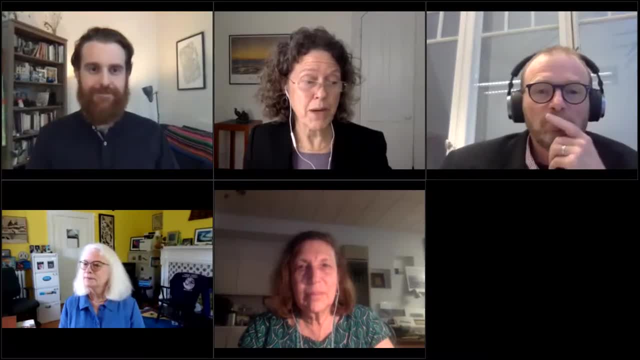 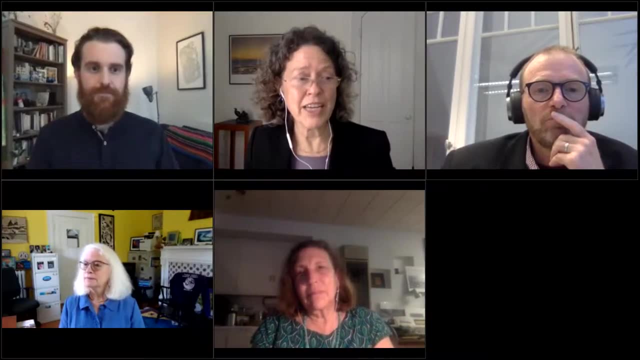 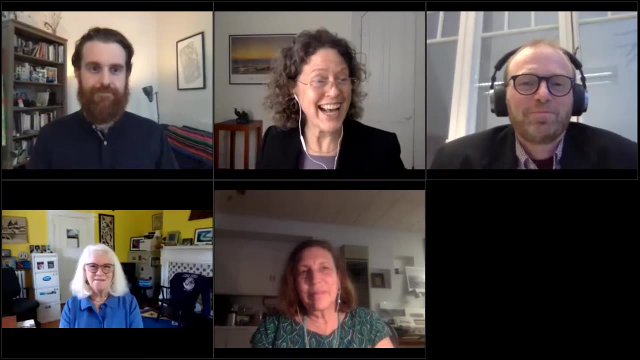 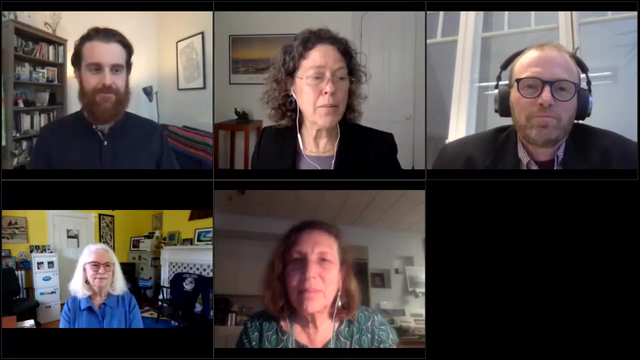 two and three of the French code of environment, especially for the public consultation slash investigation. that is crucial to decision making process regarding a given project. It probably would be well worth looking at it. in any case, And if anyone can answer specifically, excellent. And then from Ipshita Chaturvedi, a question about how important is including people. 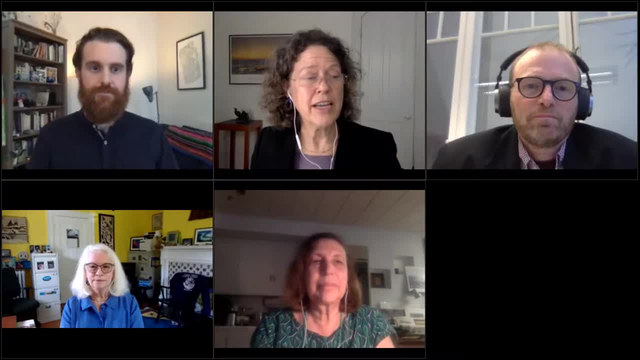 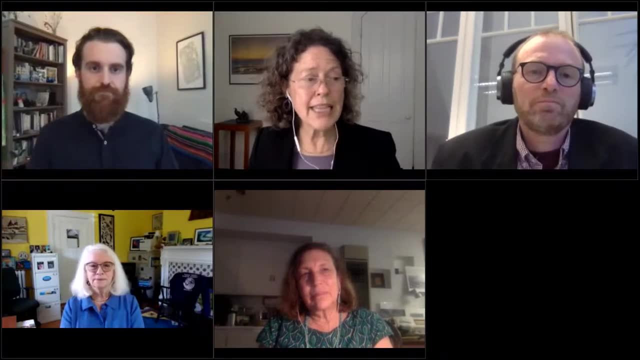 from other countries to discuss EIA parameters in the oceans. If it is important, then why do we see their representation missing constantly, And I'd like to make a quick comment to that myself, which is that it's one of the things that I find extremely valuable about the UN. 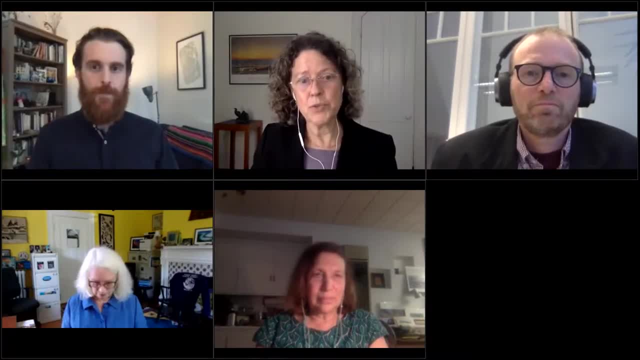 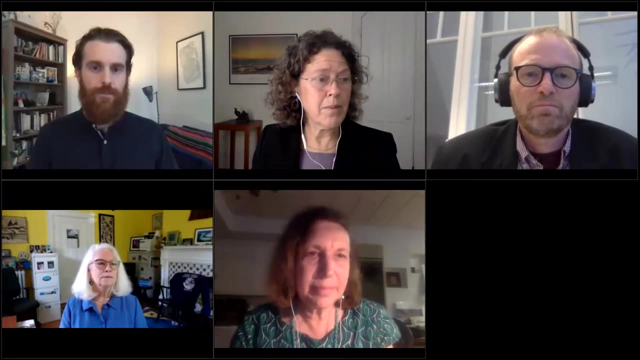 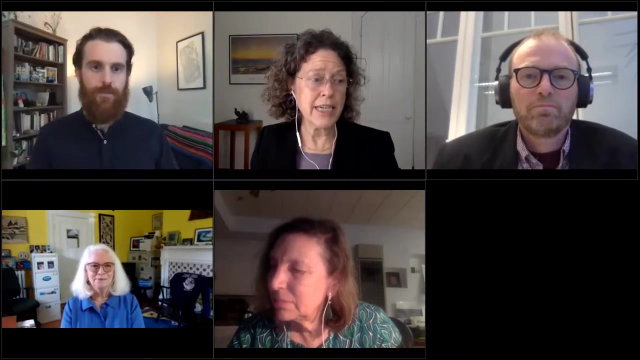 which is often derided, but it is a place where we do get to hear voices from developing countries, and they are not necessarily small islands states which are often have difficulty because of resources having access. And finally, a question: The Antarctic Treaty System has a detailed EIA. 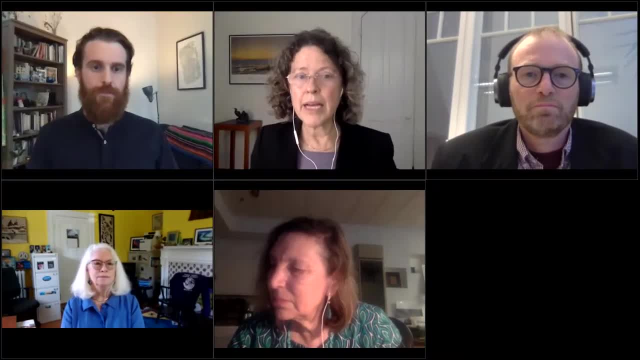 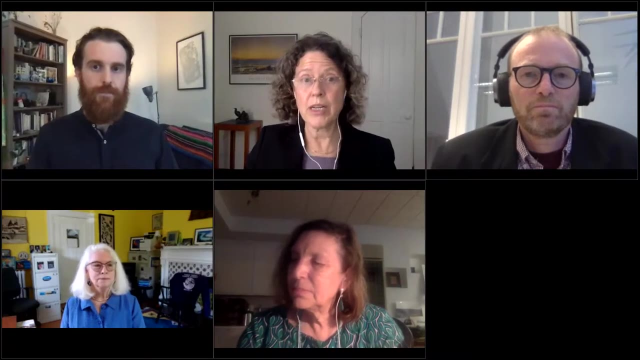 system, What lessons can be drawn from it? And I will also make a quick note that the high seas Alliance has a paper about the Madrid Protocol on its website. So if you Google high seas Alliance, you can find a very interesting paper talking about exactly this. 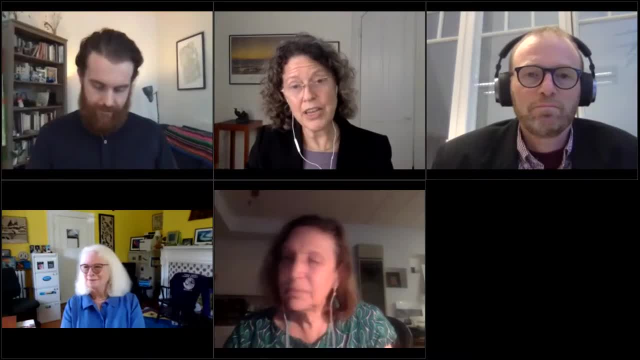 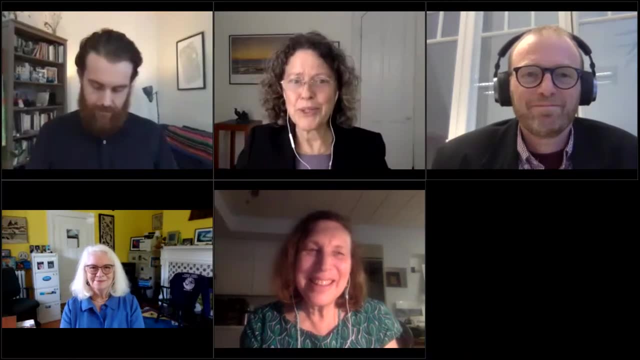 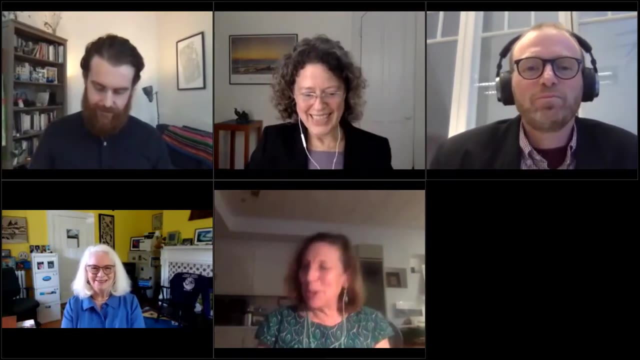 So now let me turn it over. Dr Levin, would you like to start off with your valedictory words and comments? OK, well, all right. I am perhaps the only non-policy person on here. I'm a scientist, but I guess I'll just come in on one of these questions. 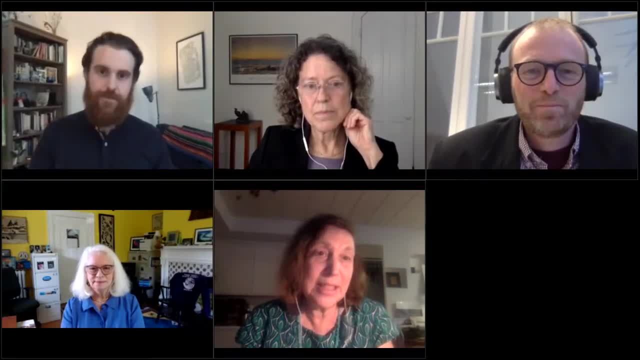 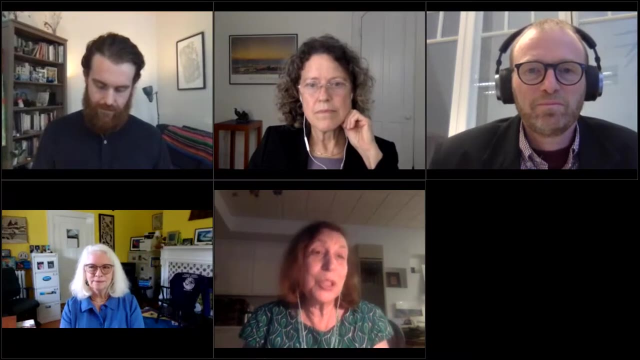 And that has to do with the engagement of these less developed countries, And I would say that we have not done an adequate job of raising awareness about the importance of areas beyond national jurisdiction. Most people, if they know anything about the ocean, it's what's in their backyard, if they live near the coast. 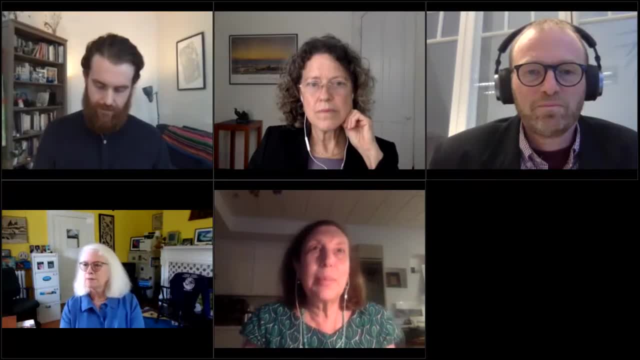 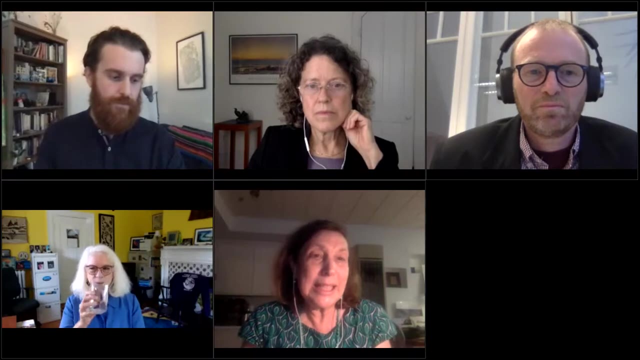 And I do think that the incredible importance in terms of biodiversity and climate regulation and more needs to become more common knowledge in not just less developed countries, but landlocked countries as well. I think everybody has a stake in what happens in areas beyond national jurisdiction. 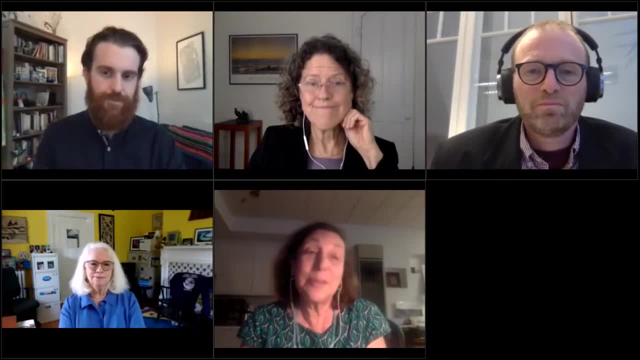 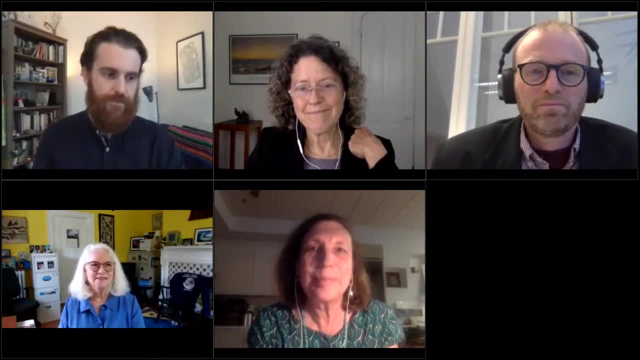 but most of the people on this planet don't know that, and they need to, And we need to work harder at making that information available. Meinhardt, would you like to Thank you? Lisa? Thank you for your participation. Yeah, So. 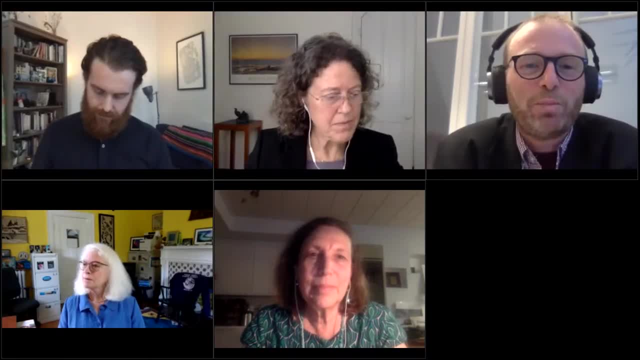 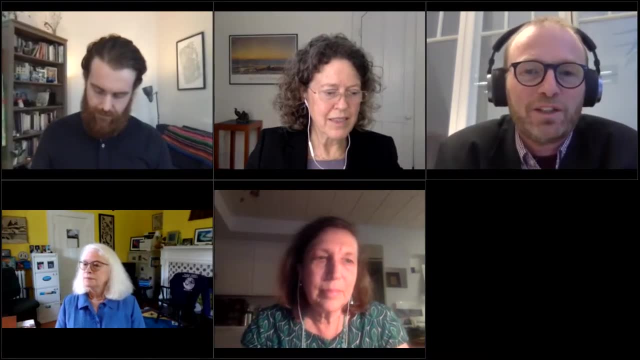 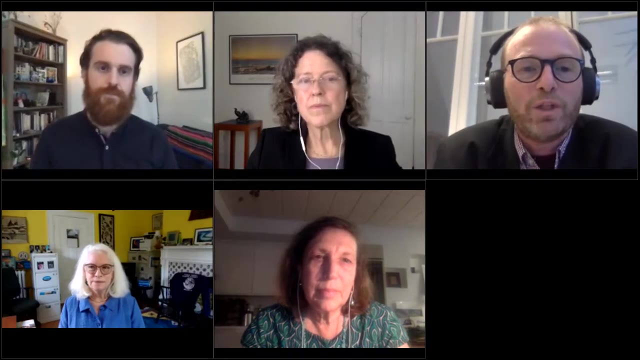 I'll just make a couple of general comments that I think maybe go part way towards answering some of the questions, And so my general observation and recommendation is that we need to draw on all experience with environmental impact assessment, with how to integrate climate change into environmental impact assessment. 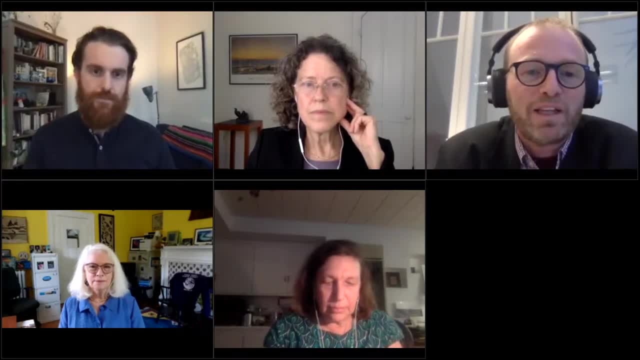 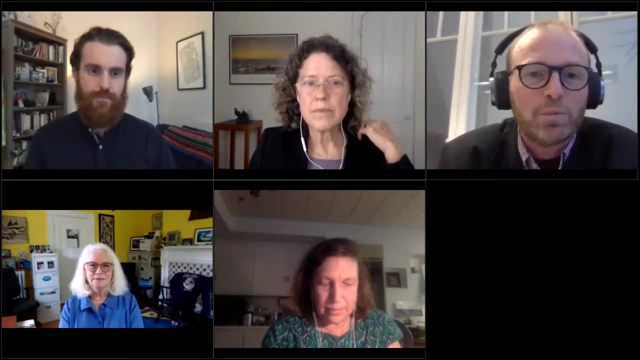 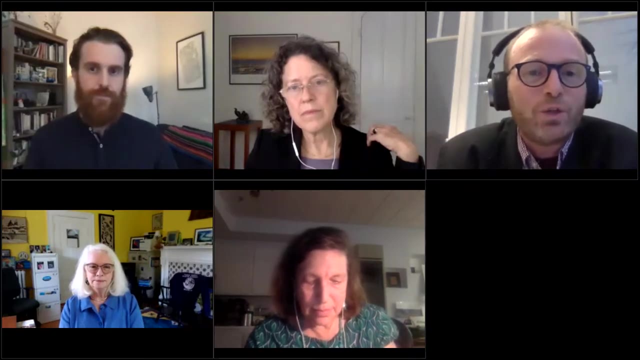 with how to engage the public effectively: environmental impact assessment. So, whether that's the French code, or whether that is experienced in developing countries, or whether that is the protocol, we need to draw on all of that. But what we need to avoid is to try to look to one existing system and just copy and paste. 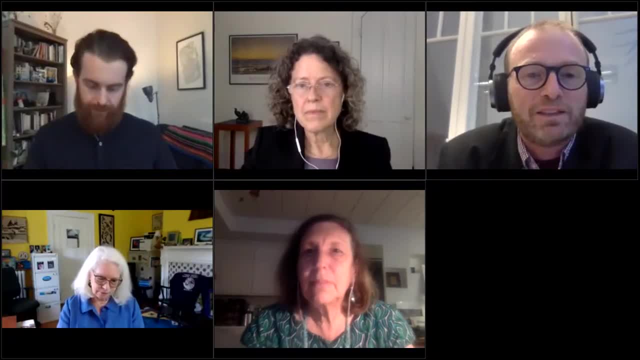 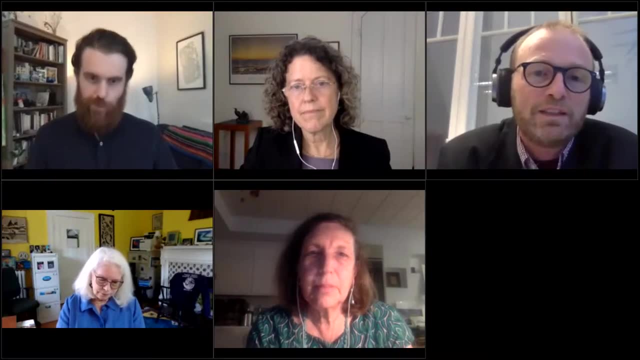 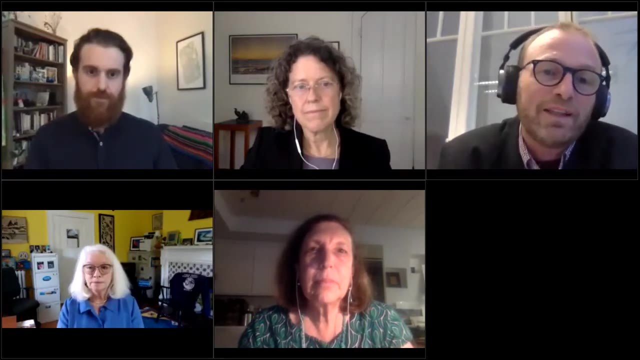 because we're trying to develop an environmental impact assessment process that will stand the test of time and that is ready for the huge challenges that the high seas are facing, And we cannot do that by simply basing this process on past experience, And that is, frankly, the biggest concern I have. 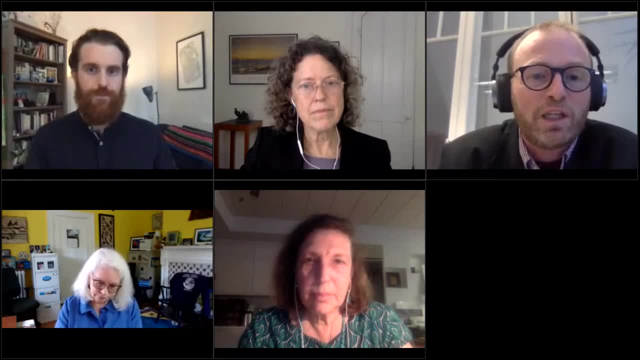 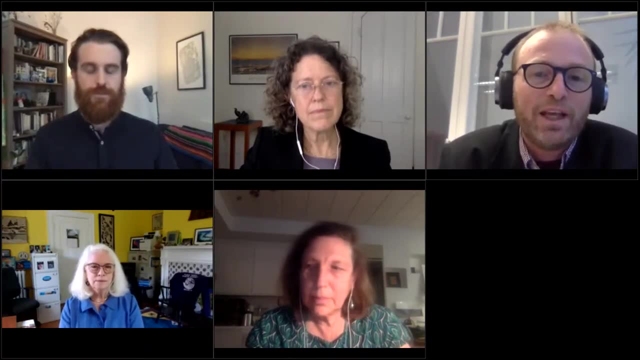 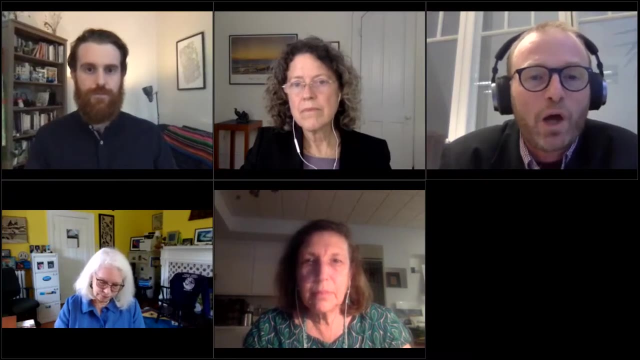 And the reason Gunnar and I wrote the piece that we did is because we feel that we need new perspectives on how to do this effectively, And that means going beyond current practice, And there are many rich ideas about how to do things better going forward. 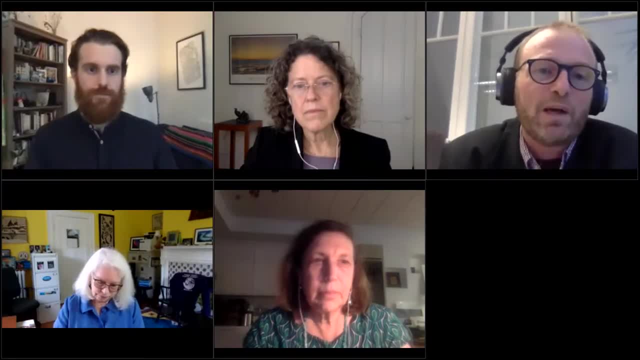 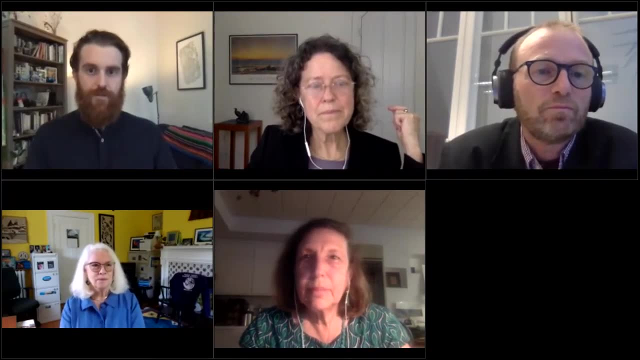 And I think we need to draw on those lessons if we're going to set up an effective plan. Thank you, That's great, Glenn. I really don't have much to add to that. I mean, I would stress very much the same. 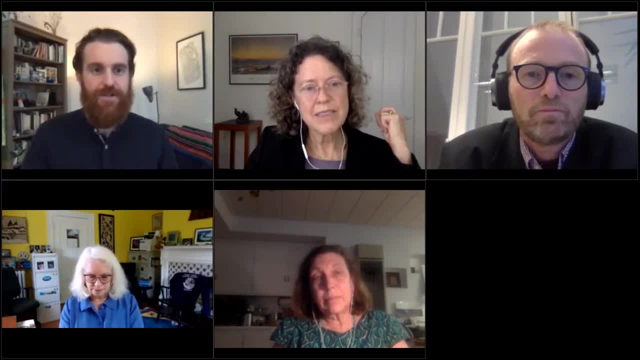 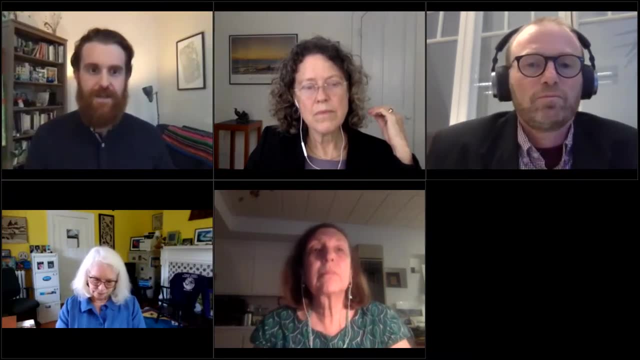 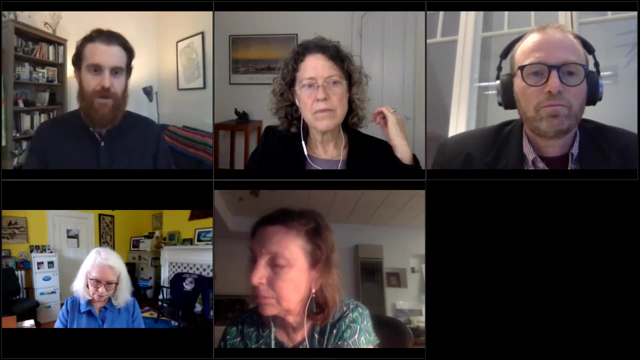 I mean, my concern is that in the negotiations we are still focused very much on a kind of procedural and technical EIA process and missing that bigger picture sort of assessments and regional and strategic assessments and actually bringing a coherent process that is focused on biodiversity, climate and the ecosystems. 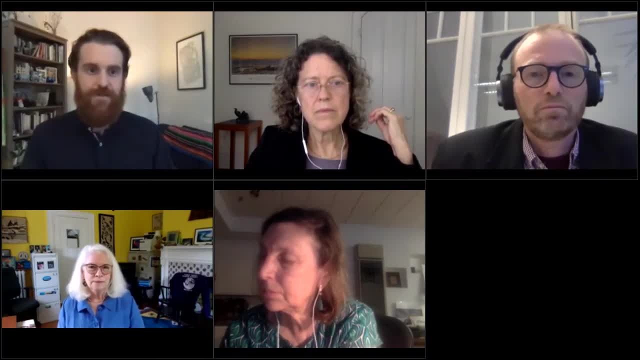 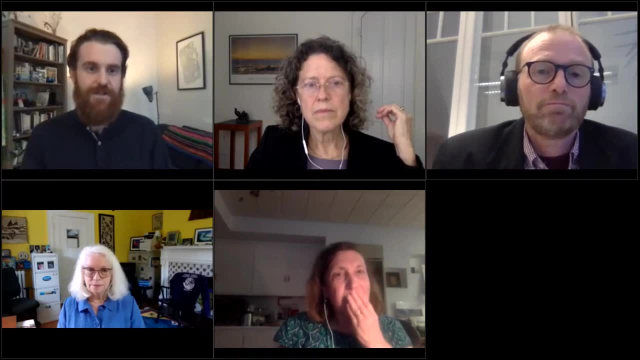 rather than on specific processes for projects and for sectors. And I mean, I think impact assessment has come a very long way in the last few decades and the treaty really ought to reflect that. And I think you're absolutely right, Meinhard. 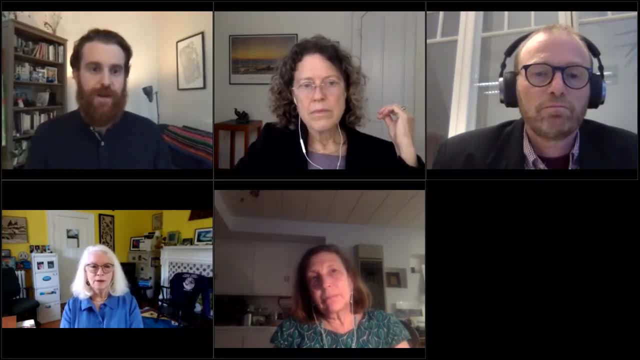 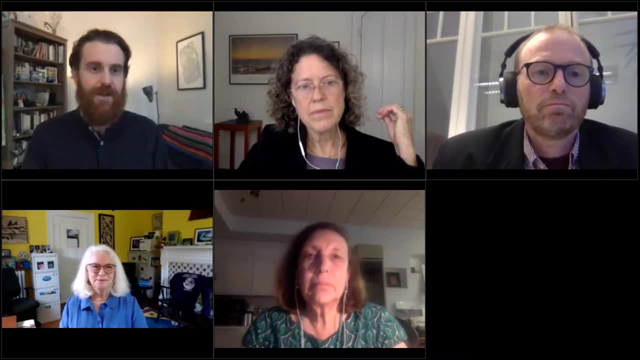 I mean, if you can draw from different examples that we already have, great. But actually the high seas is its own. you know specific context and it has its own challenges And so, if anything, we actually need to modernize and sort of 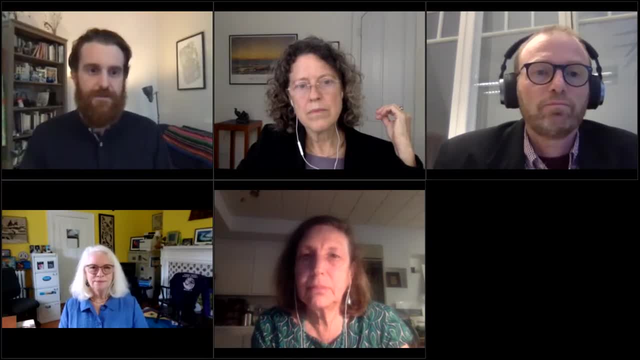 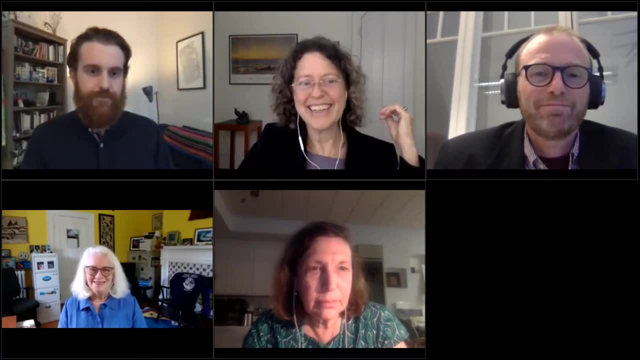 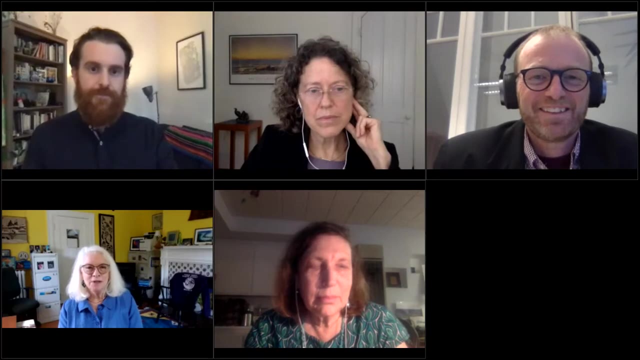 make bespoke processes even more clearly for the high seas. So, yeah, I would stress that also. Thank you And Christina, a brief word, Okay. Well, having been involved in the discussions on deep-sea bottom fishing, I would just stress the importance of now we have an opportunity to include at least a substantive 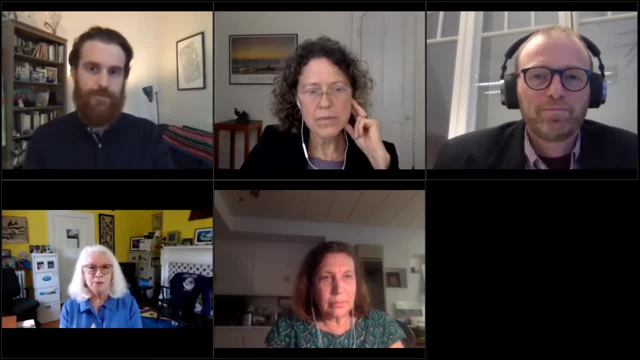 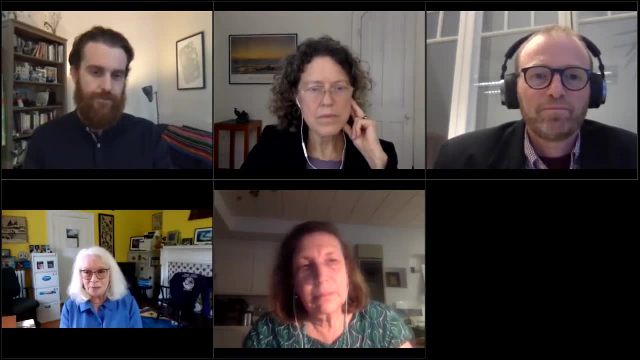 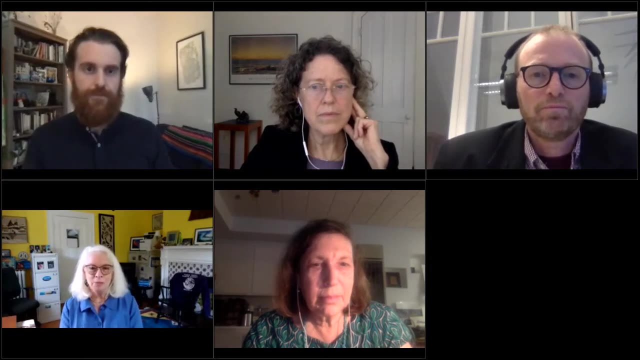 objective, Substantive direction, not to be causing significant adverse impacts. That was with the deep-sea bottom fishing. It took the United Nations General Assembly to adopt a resolution to say we need to be conducting environmental impact assessments and we need to be adopting managing practices to ensure we avoid significant adverse impacts. 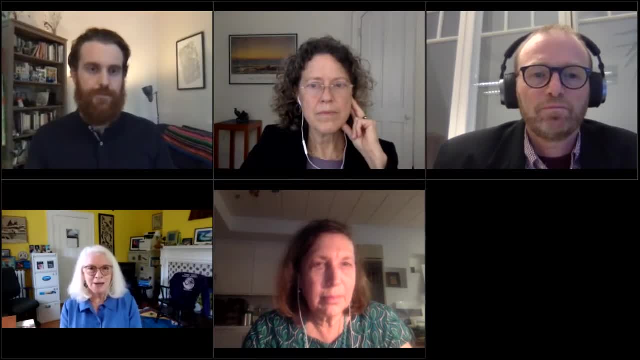 And this in many ways revolutionized fisheries management for the non-tuna RFMOs. but we still lack those procedural safeguards That we get from the Convention on Biological Diversity or from the best practice and, hopefully, the BB&J. 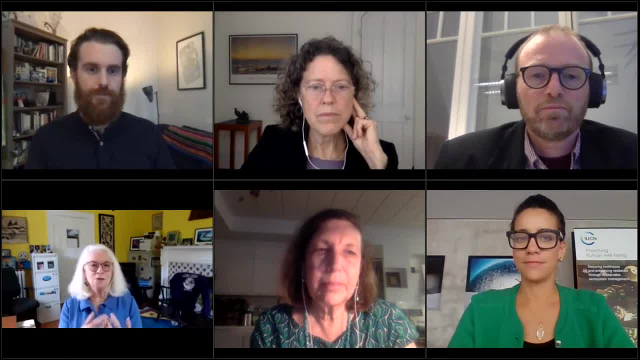 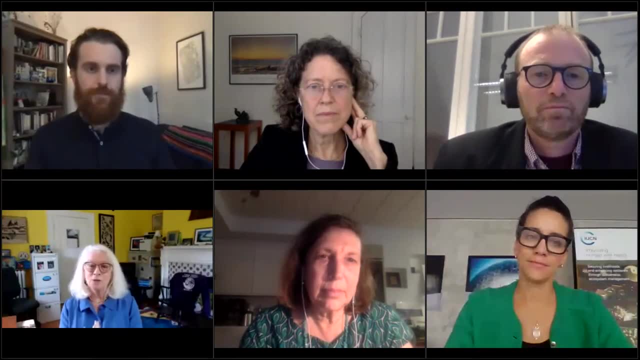 So we need a marriage of best practice from within, beyond national jurisdiction, to create a new agreement that truly is fit for purpose for the next 20,, 30, and hopefully 50 years. So thank you, Thank you all. 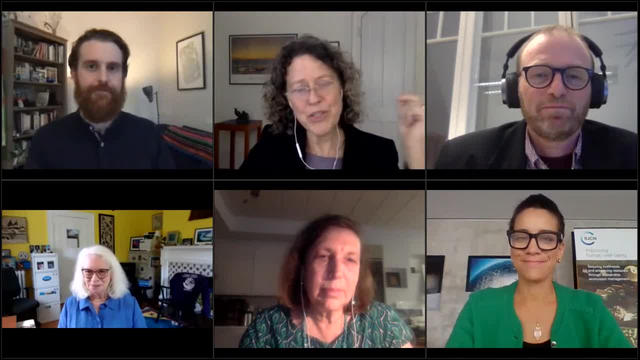 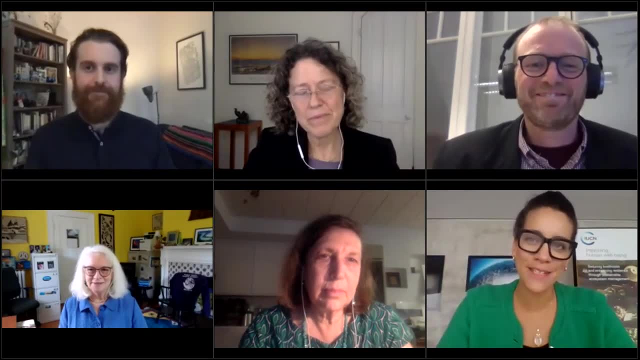 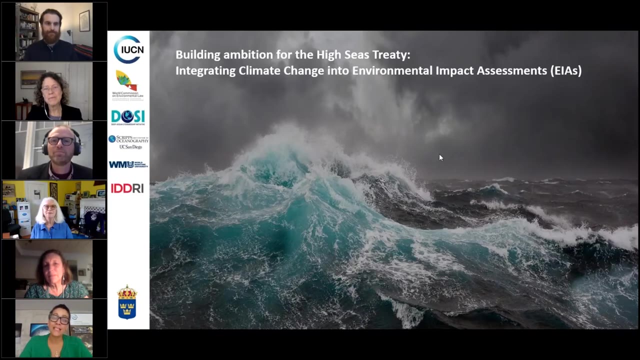 And I'd now like to turn the floor over to Mina Epps. please Yes out, Mina. Thank you very much, Simi, And thank you for excellent speakers, for your very concise and extremely informative presentations. You highlighted the need for baselines, triggers and thresholds. 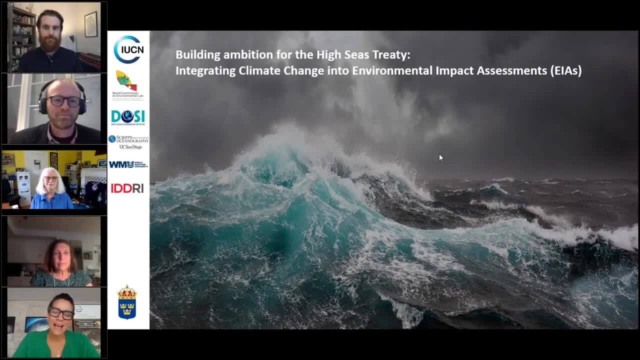 You shed a light on the mesopelagic zone, so thank you for that, But also to share your valuable knowledge and lessons learned and giving us some takeaways for concrete actions, to mainstream climate change integration, into environmental impact assessment and, ultimately, into 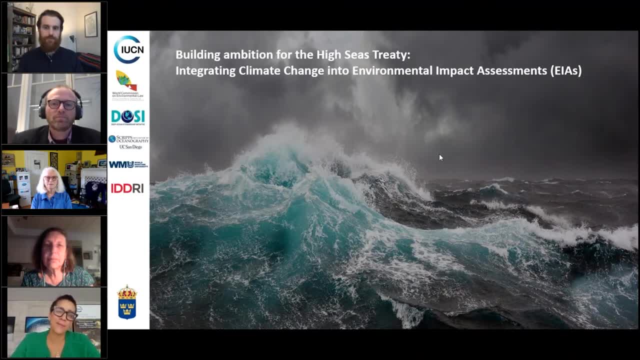 a new legally binding agreement. We need an ambitious agreement and the treaty needs to be future-proof. as we just heard- And with that I would also like to end- that we will actually be hosting another webinar on the 22nd of October, which is about continuing building ambitions for the High Seas Treaty.